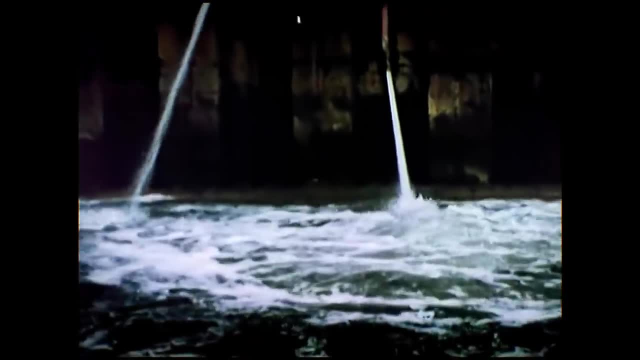 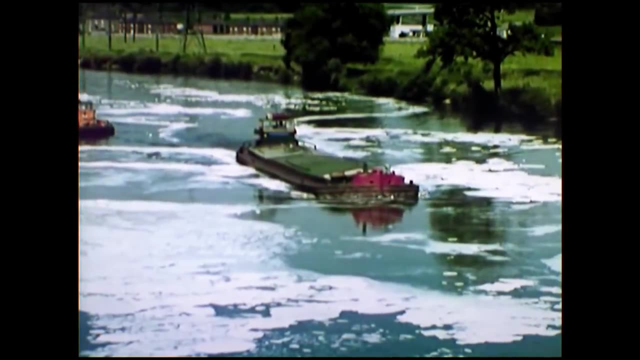 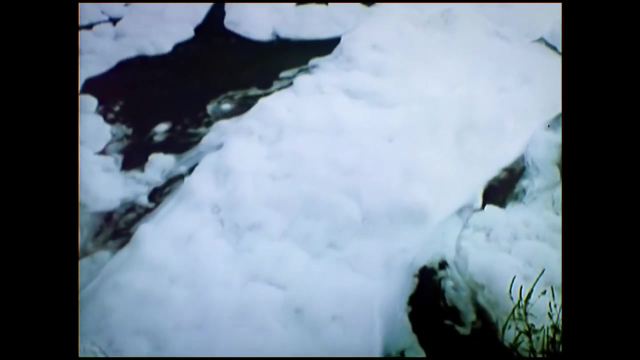 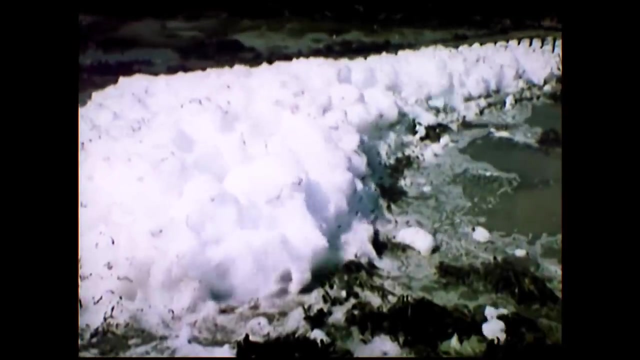 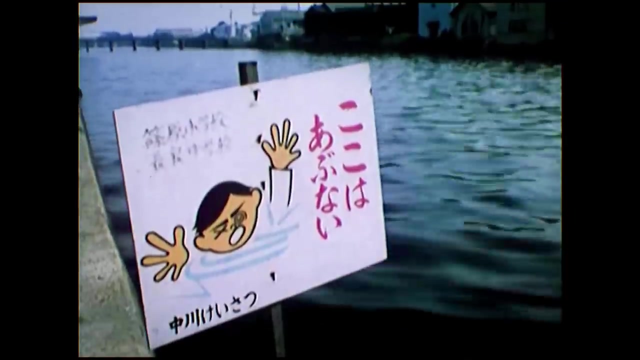 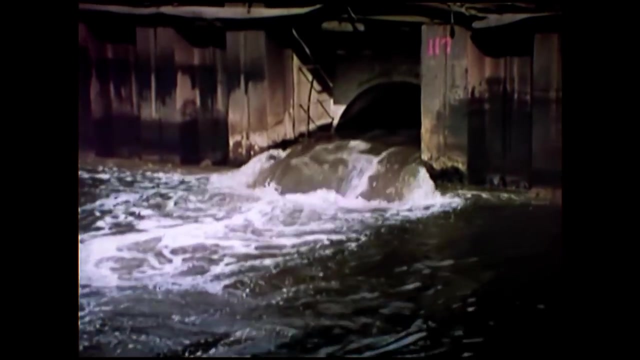 This is the shadow of progress. The sum of the world's water remains constant. Water cannot be depleted, but its purity can, and so can its usefulness. No one wanted this to happen. It is something we drifted into, a by-product of making things. 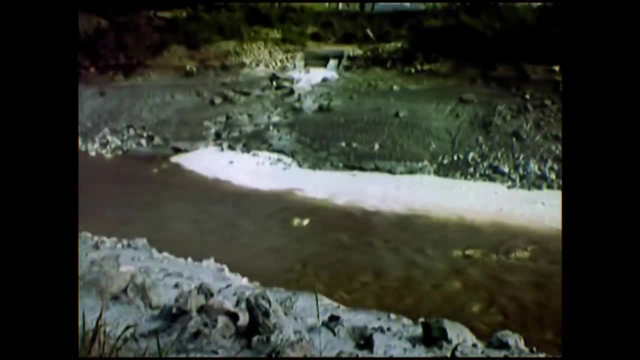 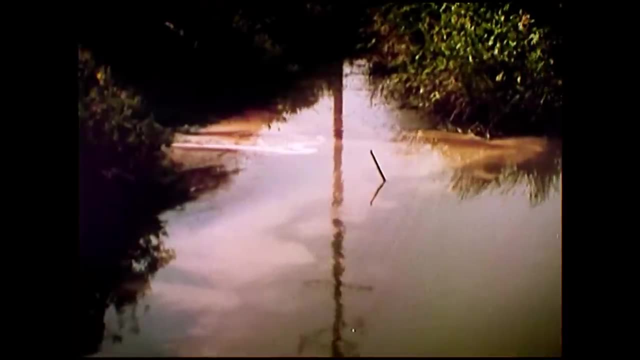 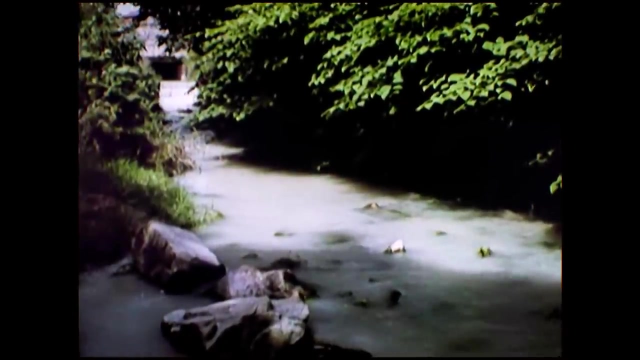 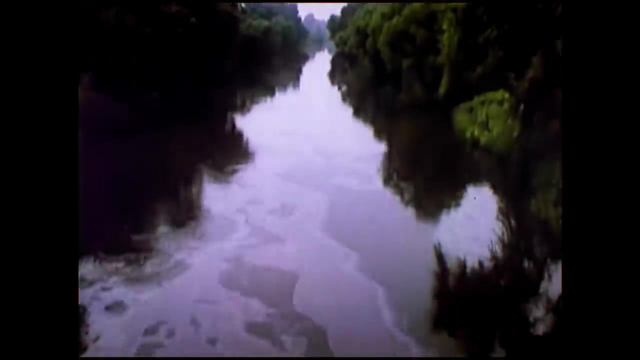 the good things, The things man wants more and more. We are all accessory to the murder of rivers, And so we have created a paradox: a scarcity not of water, but of usable water, An inexhaustible resource in short supply. 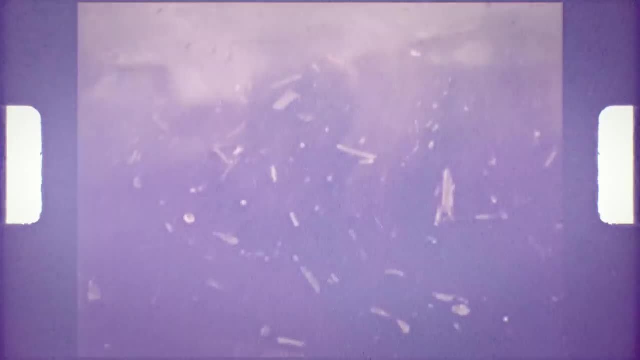 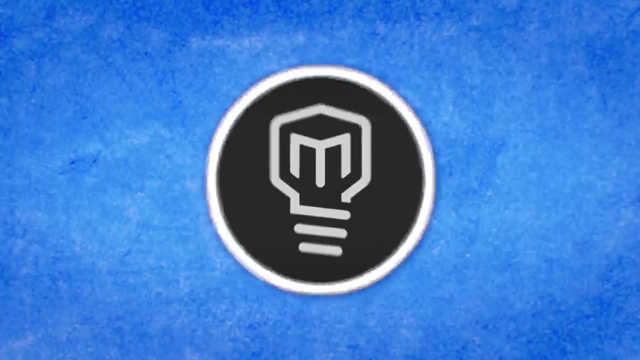 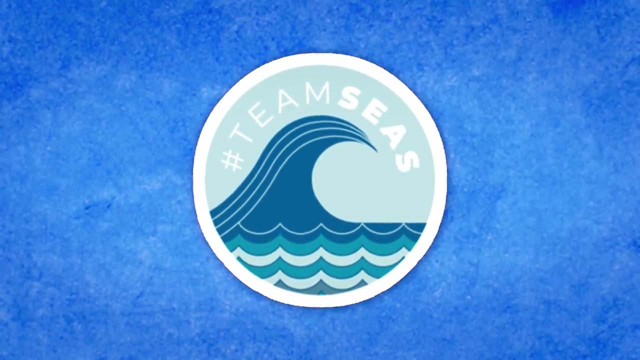 If you've been anywhere on YouTube over the past few weeks, you've probably heard that Mark Rober and MrBeast put together another big fundraiser like Team Trees, only now it's Team Seas, where every dollar donated helps take a pound of trash out of our oceans, and 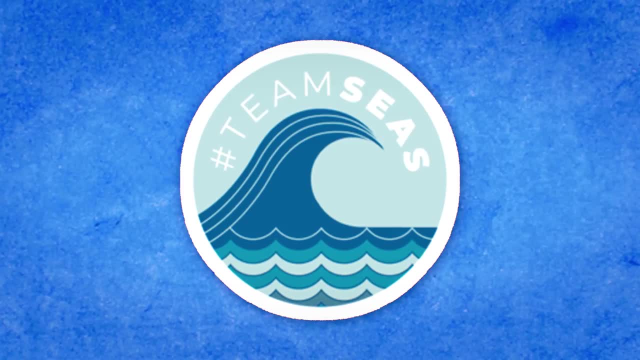 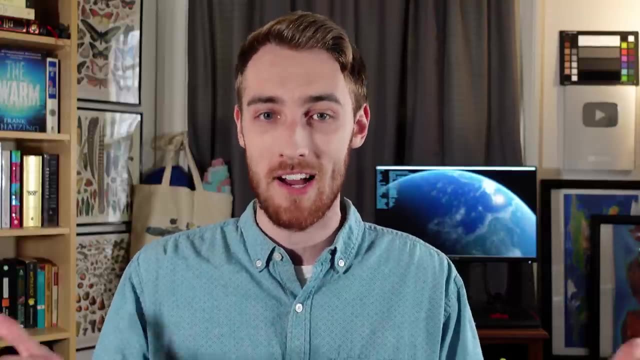 they invited any and all YouTubers to join in to promote it. And, just like last time, I had no idea this was happening. I was completely unprepared and I was already working on something else, But I was determined to make this video anyway. 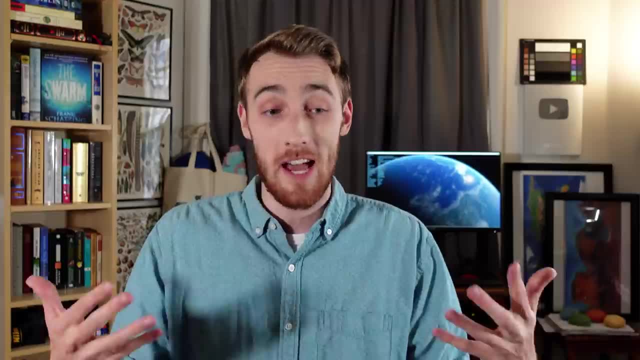 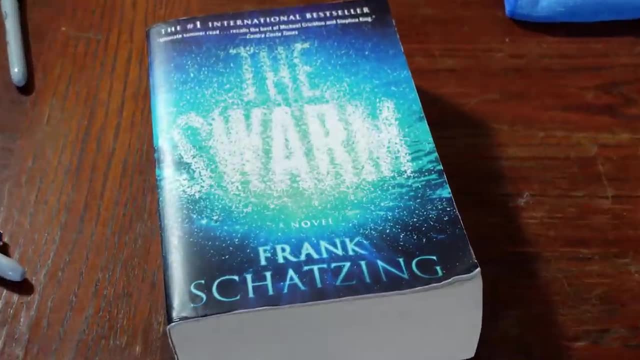 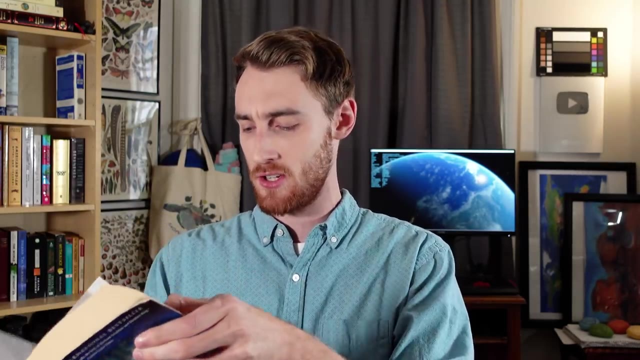 even if it had to be a month late, because, well, actually I've been thinking a lot about the ocean lately. You see, for this past year I've been reading this book, The Swarm, by Frank Shotzing. Yes, you heard right, I've been reading the same book for a year now, but in my defense I'm on page 691 out of 898.. 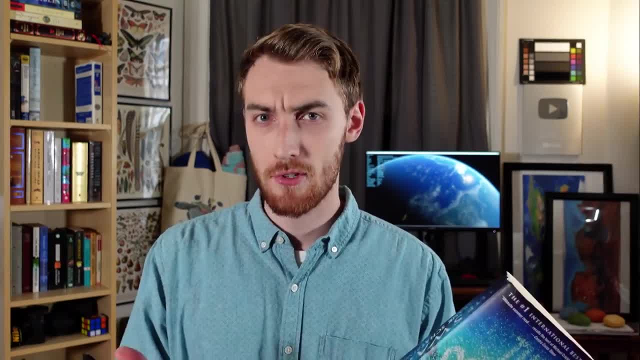 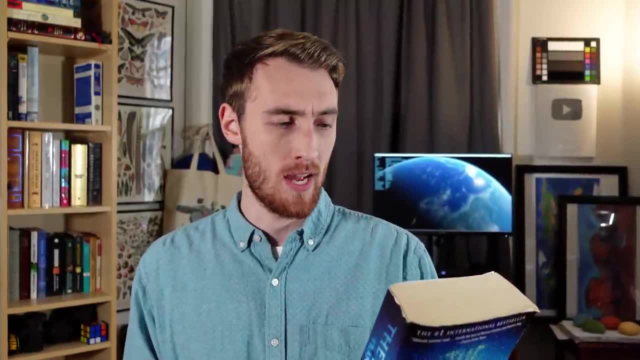 So close to finishing. To give a quick summary of the book so far, we can read the back where it says: Whales begin sinking ships, Toxic eyeless crabs poison Long Island's water supply. The North Sea shelf collapses, killing thousands in Europe. Around the world, countries are beginning to 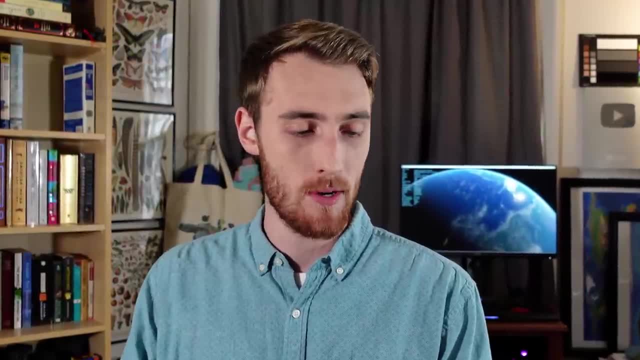 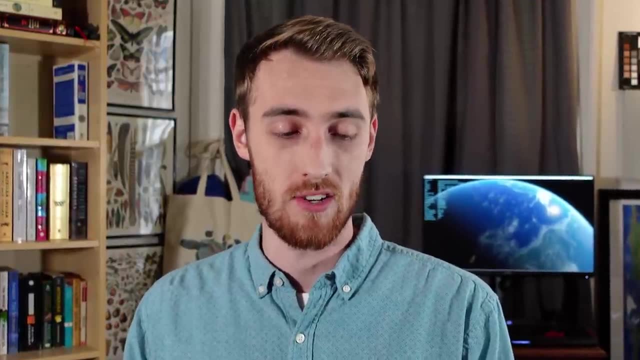 feel the effects of the ocean's revenge, as the seas and their inhabitants begin a violent revolution against mankind. At stake is the survival of the Earth's fragile ecology and, ultimately, the survival of the human race itself. And okay, while this is clearly a work, 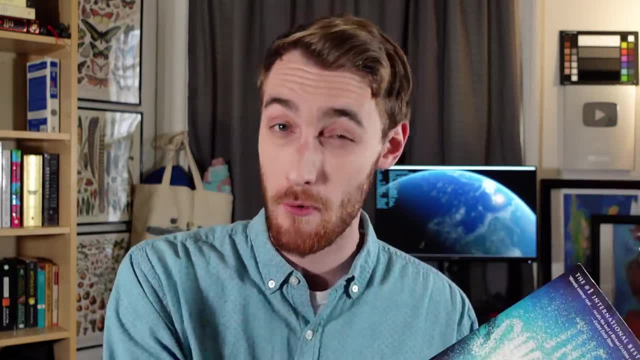 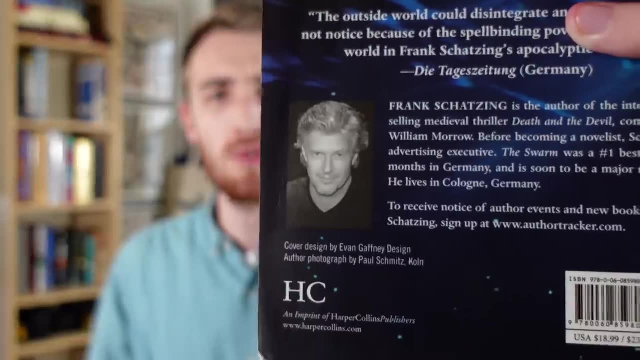 of fiction, one that was published all the way back in 2004 at that. while reading, it quickly becomes apparent that the author, Frank Schatzing- uh, this guy put a huge amount of research into his writing and approached the story in a very scientific manner. This is made no clearer than. 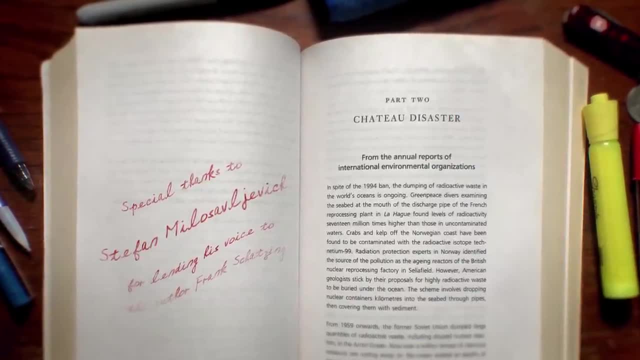 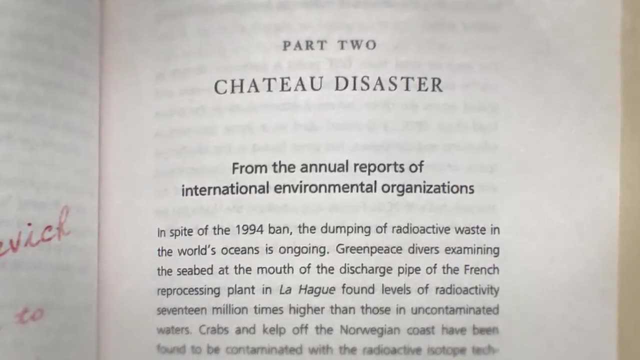 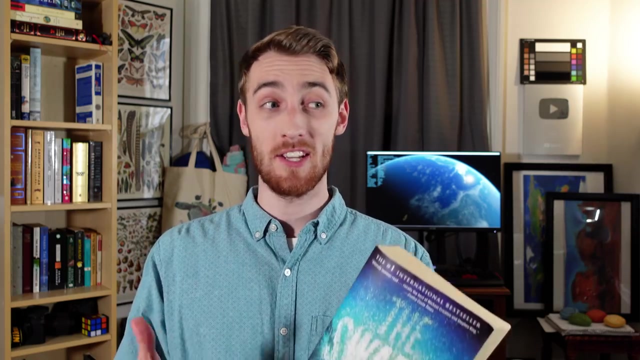 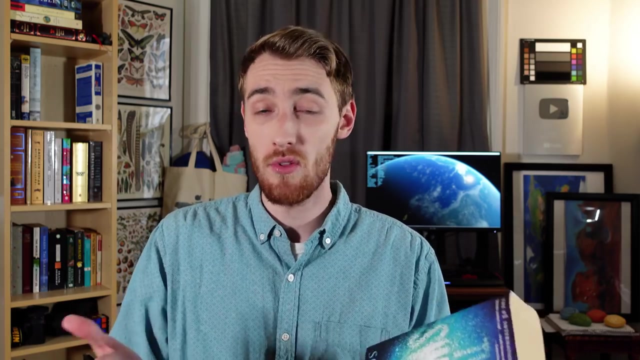 here on page 365, right after the climax of part one and before the beginning of part two, where Schatzing uses this phrase. And I'll be honest: ever since reading this passage earlier this year, I've wanted to make a video about it, because it more or less perfectly enumerates all the different ways. 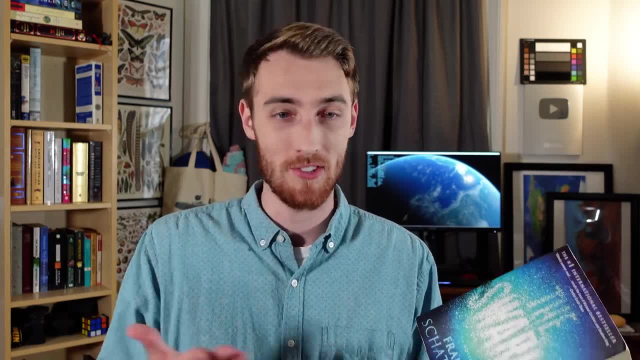 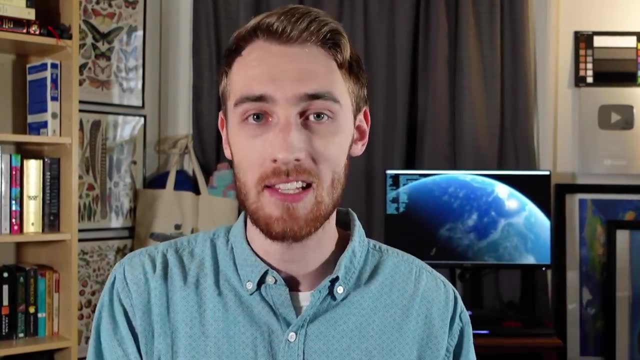 we're mistreating the ocean, And well, what better time to talk about this than right now? After all, I'm a firm believer that the first step in solving any problem is figuring out exactly what that problem is. So today, if our goal is to clean up the ocean, then we need to start with all the different ways. 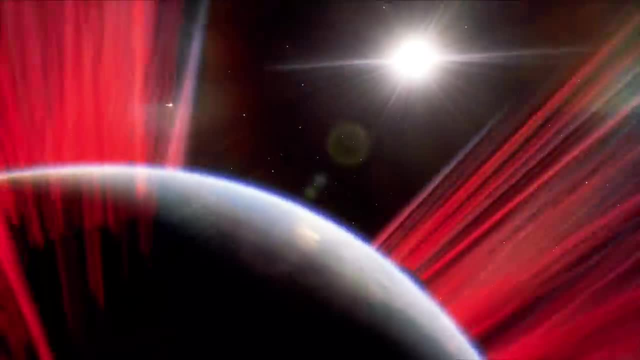 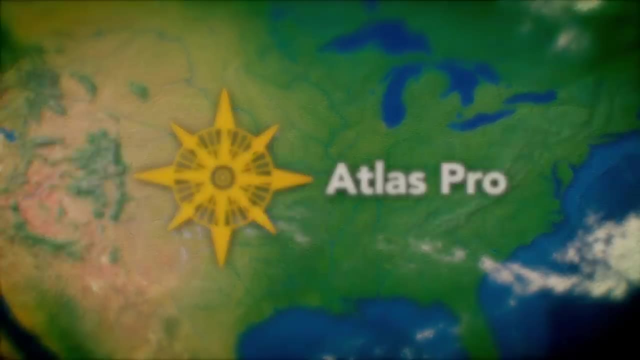 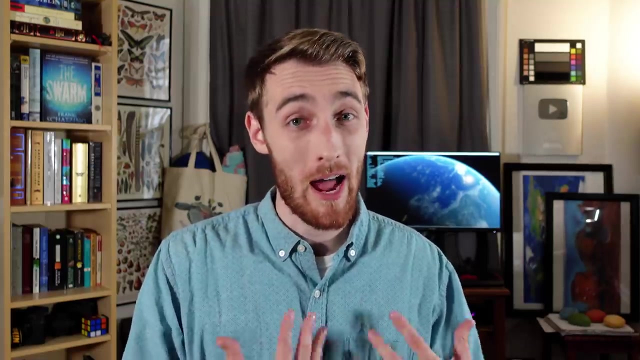 we're polluting it Now. I hate to be the one to tell you this, but the ocean is dirtier than you think- Though, to be fair, it's not all our fault- Thanks to the Earth's natural cycles of rain. 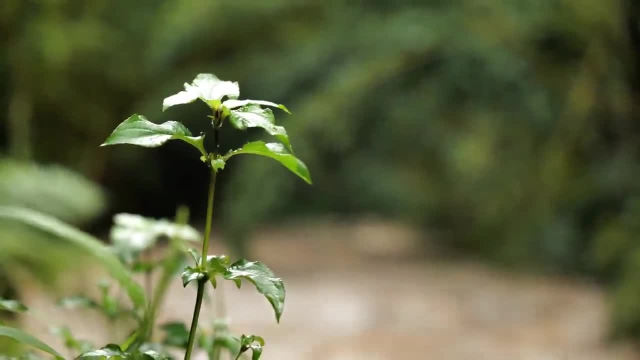 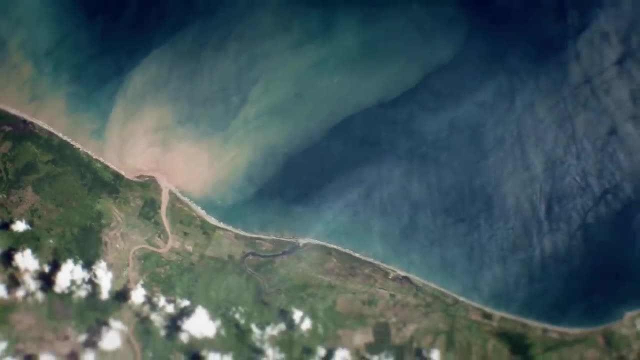 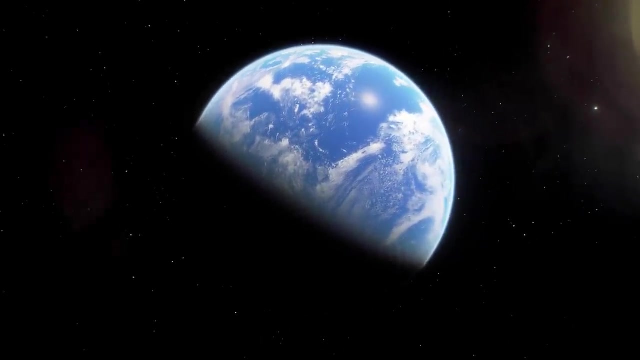 and runoff. virtually everything not secured to the ground ends up in ruins. The ocean is also a place where it's eventually taken out to sea. This means all dirt, debris and decaying matter inevitably makes its way here. Fortunately, the ocean is absolutely ginormous, and so most of this muck gets diluted down to. 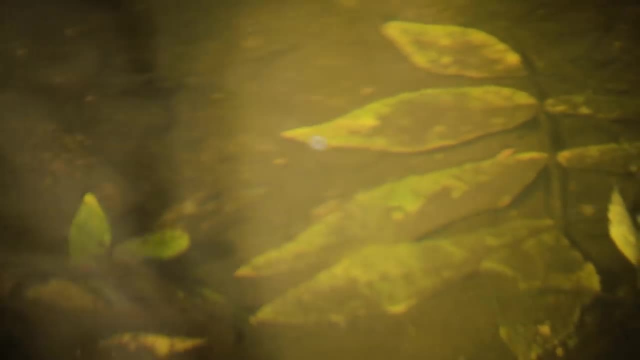 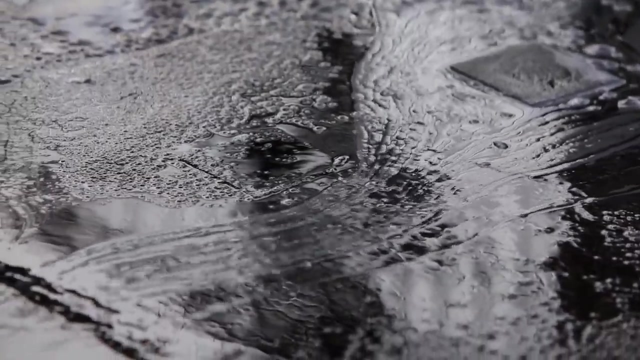 tolerable levels, to where natural systems can handle this constant influx of filth. But of course, in modern times, the runoff that finds its way to the ocean now brings with it new pollutants like oils, plastics, heavy metals, fertilizers, pesticides, chemical weapons, nuclear. 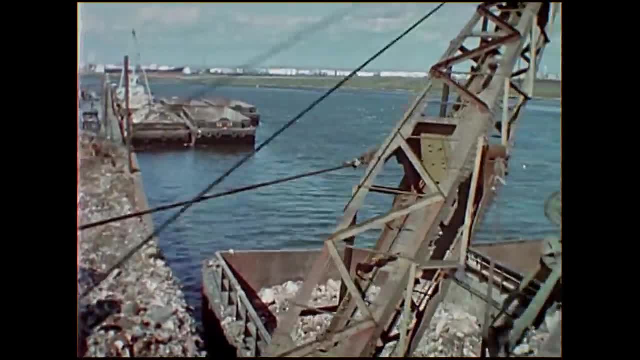 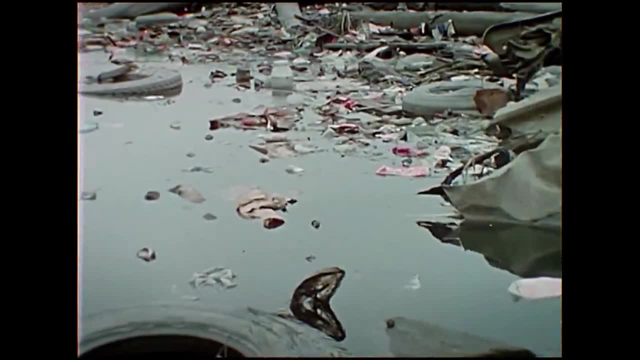 fuel. and don't forget heaps and heaps of trash, Garbage and silt. Sulfuric acid and DDT, Dieldrin and aldrin, Oil and cyanide, Silbestrol and phenol, Arsenic and ammonium chloride. 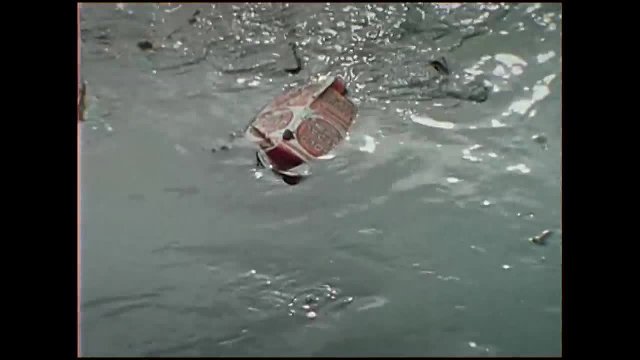 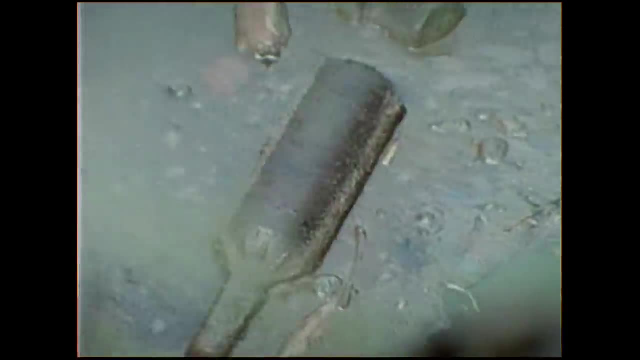 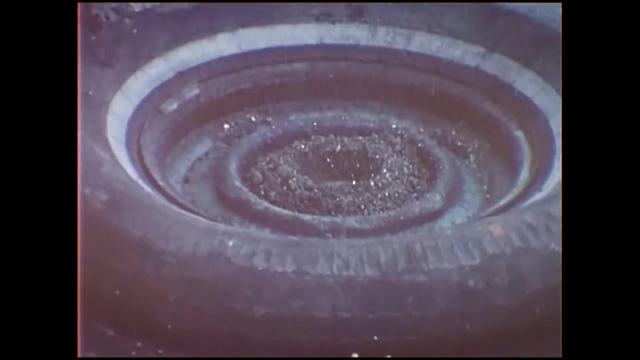 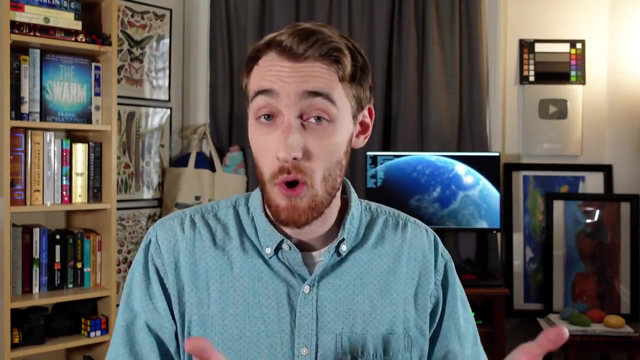 New chemicals for food, New gadgets for work, New products for a better life, New waste for the land and water. Now, the sheer magnitude of how much we've put into the ocean can be overwhelming at first. so for our sake, I'm going to group everything into a few general categories. 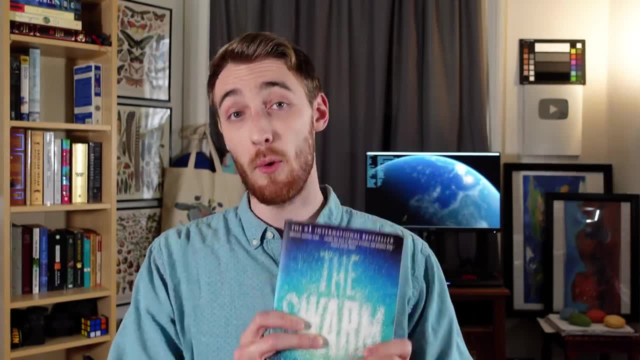 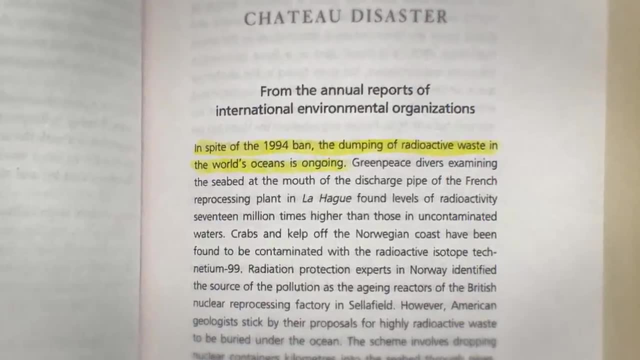 To get us started, let's look at the first words from this report. In spite of the 1994 ban, the dumping of radioactive waste in the world's oceans is ongoing. Greenpeace divers examining the seabed at the mouth of the discharge pipe of the French. 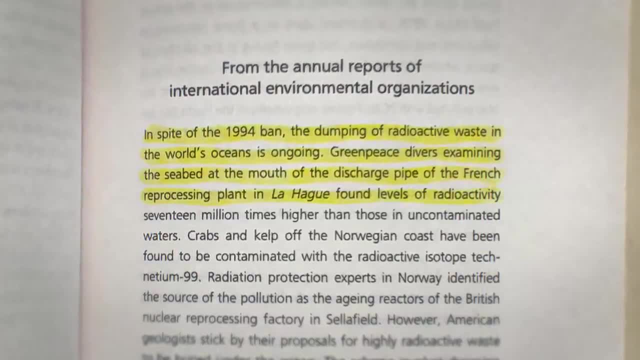 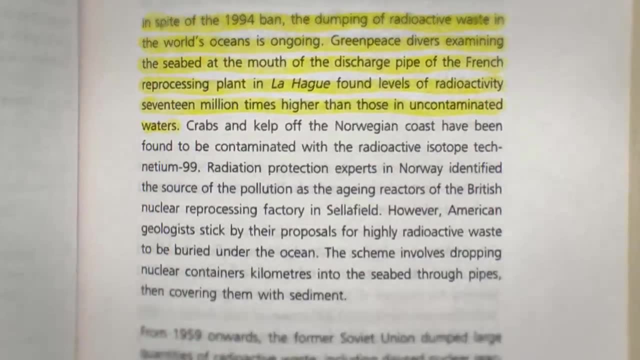 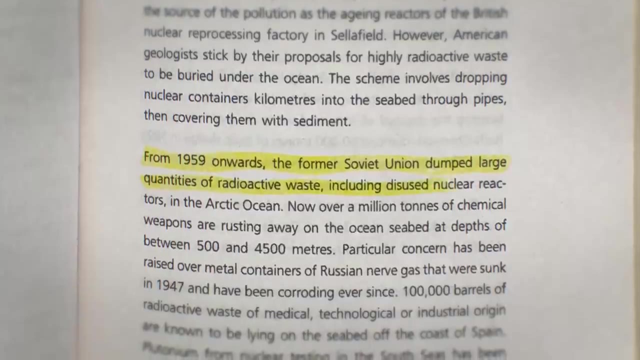 reprocessing plant in La Hague found levels of radioactivity 17 million times higher than those in uncontaminated waters. Further down, Schatzing writes: From 1959 onwards, the former Soviet Union dumped large quantities of radioactive waste, including disused nuclear reactors, in the Arctic Ocean. 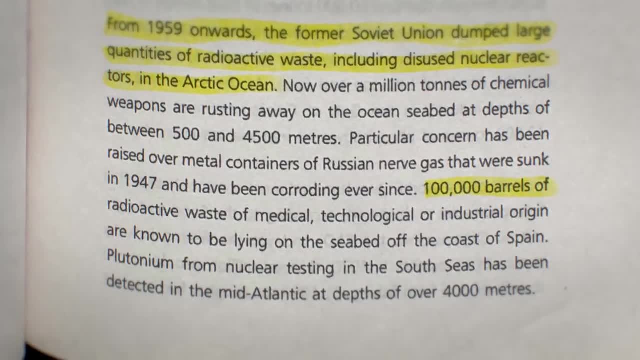 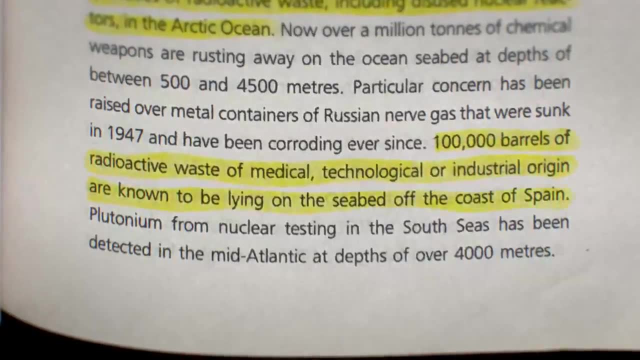 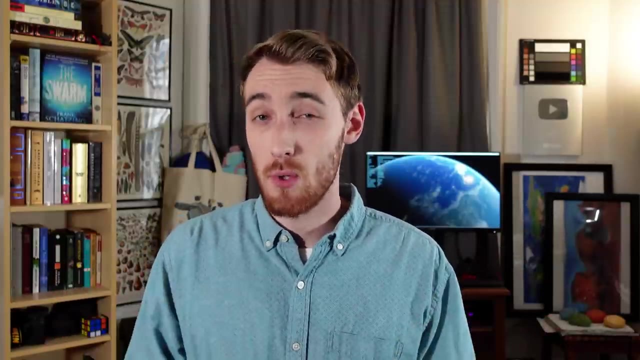 And below that, 100,000 barrels of radioactive waste of medical, technological or industrial origin are known to be lying on the seabed off the coast of Spain. Now, I'm not entirely sure if Schatzing meant to include these examples first, to indicate that they were the most pressing issue. 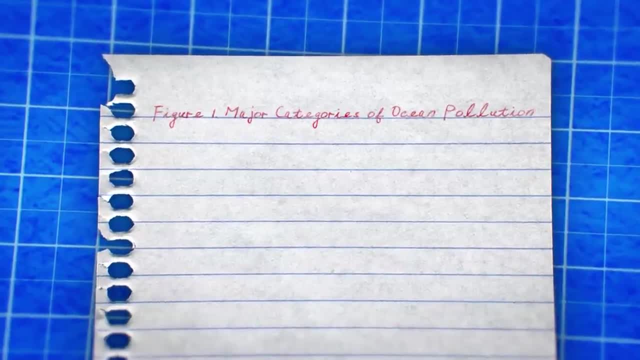 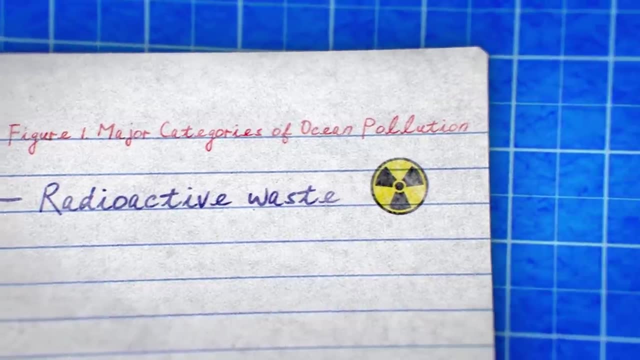 or if it just worked out like that, but either way, it's clear that our first category must be radioactive waste, And while most of these examples are pretty Eurocentric- Frank Schatzing being German, after all- it's also important to remember that the 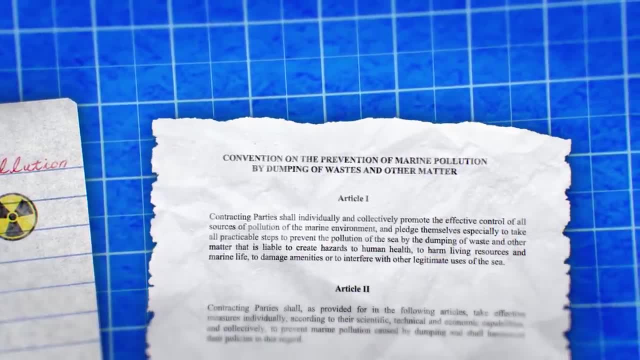 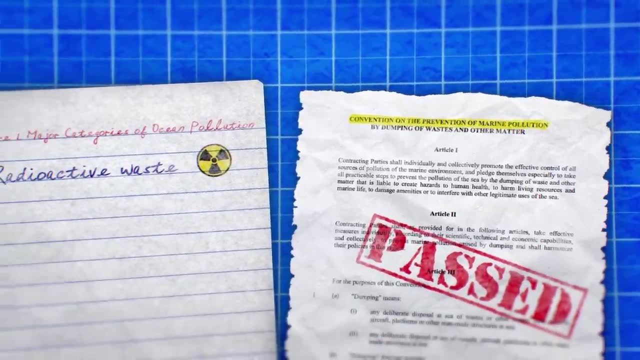 dumping of radioactive material was only banned with the Convention on the Prevention of Marine Pollution passed in 1994, meaning the only countries that really got to partake in this were nuclear's earliest adopters. The only upside to this is that, because most of this disposal was 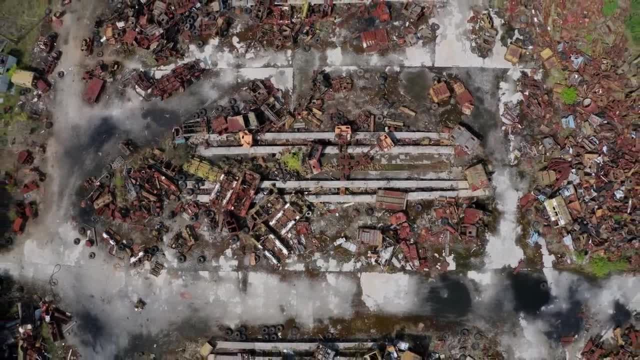 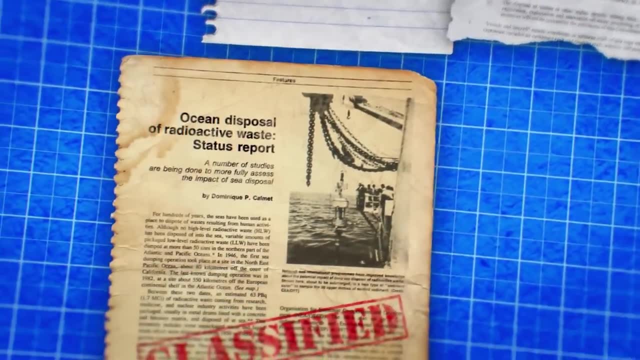 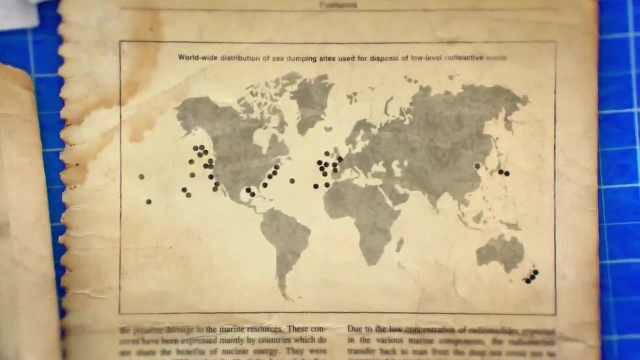 carried out by governments, pretty accurate records have actually been kept regarding where most of this waste ended up, Which is what has allowed us to create reports like this one, published all the way back in 1989, where we can find maps like this detailing the exact locations where nuclear waste has been dumped. 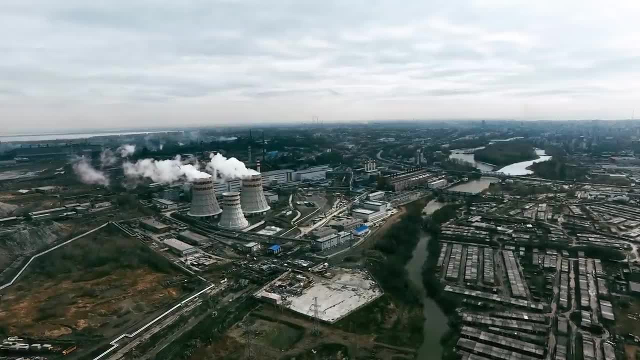 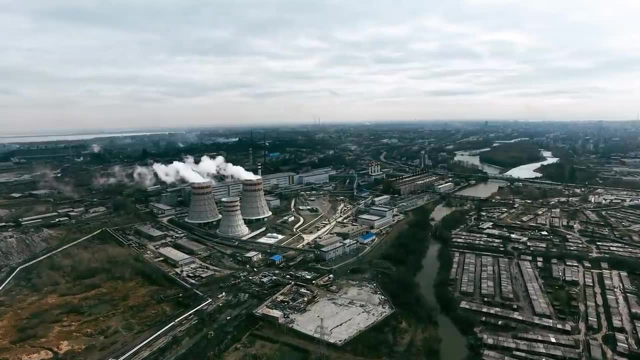 In fact being something we started playing around with less than a century ago. literally all the radioactive waste that's ever been dumped in the ocean has been done within a single human lifetime, meaning we can even look back to the site where the very first nuclear waste was put. 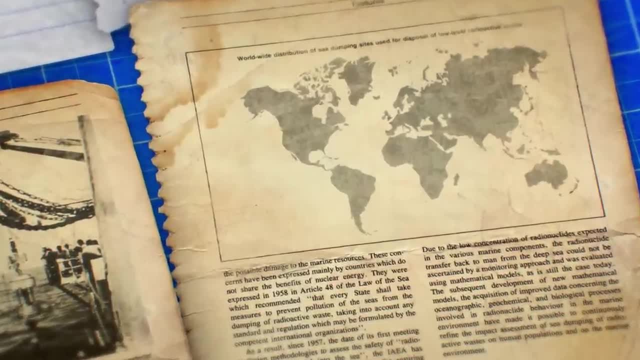 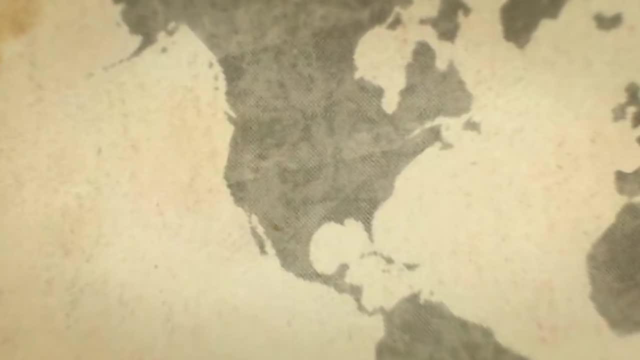 into the ocean As the first country to build and use nuclear weapons. it shouldn't come as any surprise that the United States was the first country to build and use nuclear weapons. The United States kicked off the trend of dumping radioactive waste into the ocean in 1946,. 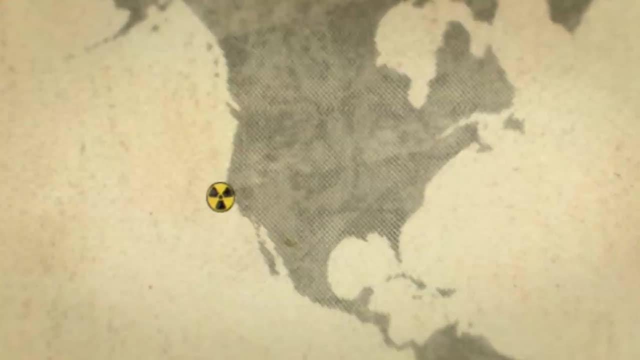 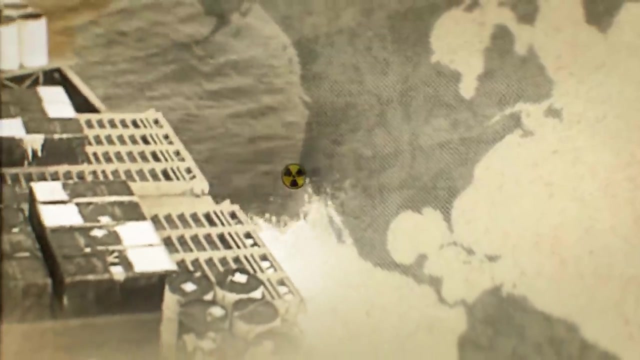 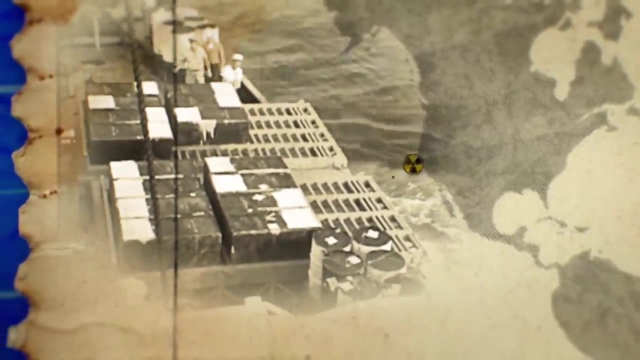 when they sunk the waste products of the Manhattan Project. 80 kilometers off the coast of California, Tripping a dog releases four vaults which go overside almost simultaneously, but without any damaging collisions. This is done at the dumping ground prescribed in the waste disposal license granted by the Atomic Energy Commission. 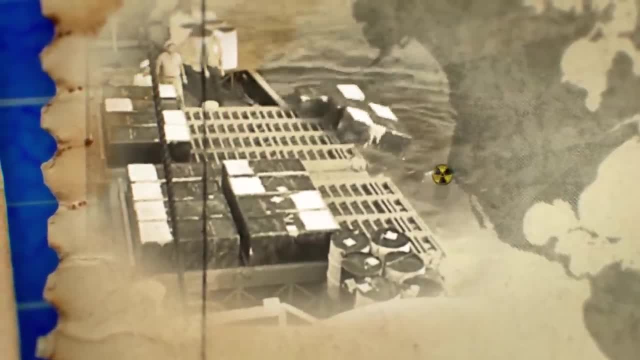 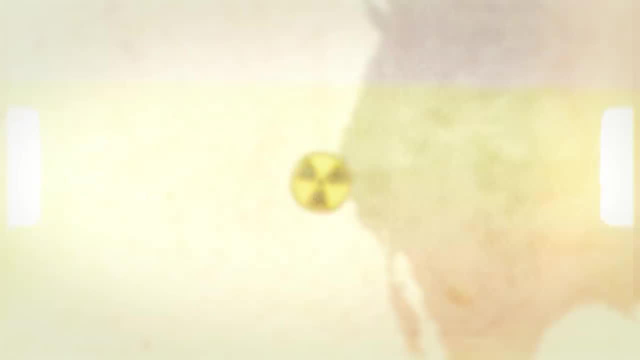 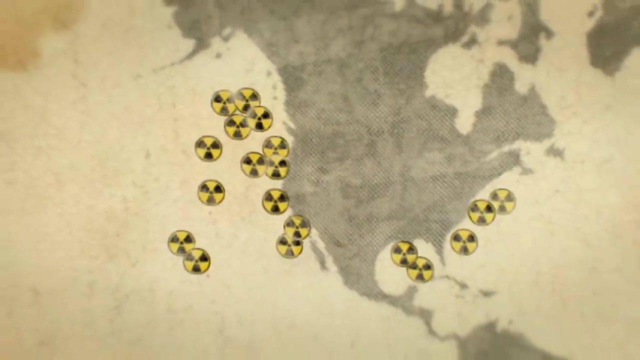 Here, the fathometer reading for one particular trip indicates that disposal is made at a depth of 1,000 fathoms. After this, only more and more nuclear tests were made, generating more and more waste that needed to be dumped, and soon enough, both the east and west coast of the country hosted. numerous large deposits of radioactive material. Of course, while the US might have been the first, it certainly wasn't the only country to unleash the power of the atom, and since then, three or four specific hotspots have arisen as primary locations for radioactive waste dumping Across the Atlantic. we'll find in and around the Celtic Sea to be the. 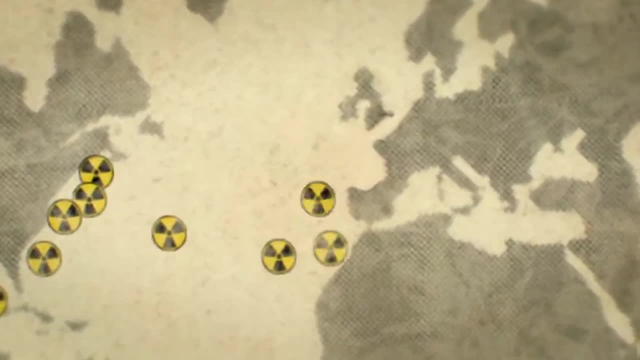 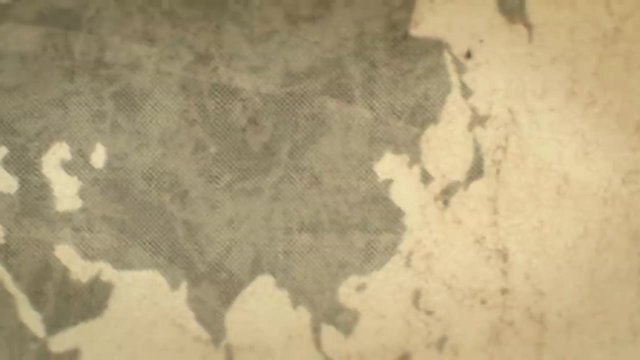 preferred dumping grounds for European countries where 1,, 2,, 3,, 4,, 5,, 6,, 7,, 8,, 9,, 10 sites were used, While on the other side of the Pacific Ocean, Japan tends to dispose of its waste along its 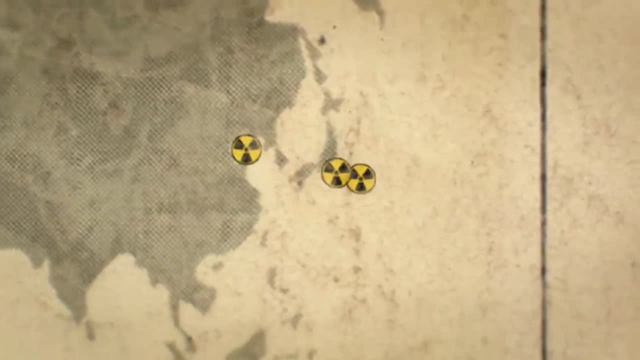 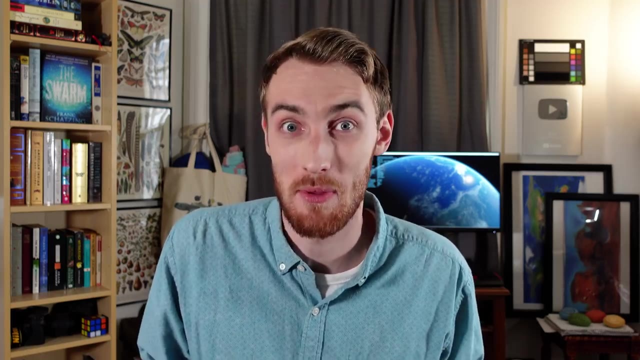 eastern coast in just two or three sites. And then there's this little hotspot all the way down here, off the southeastern shores of New Zealand, Which, I'll admit, confused me at first, especially considering the amount of radioactive waste that was dumped into the Atlantic Ocean. 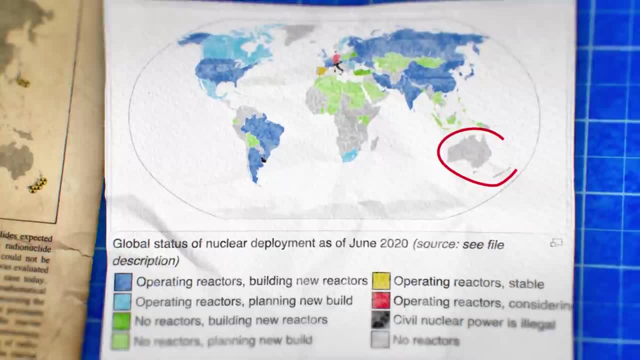 And then there's this little hotspot all the way down here off the southeastern shores of New Zealand. And then there's this little hotspot all the way down here off the southeastern shores of New Zealand. neither New Zealand or even Australia have ever operated nuclear weapons or reactors. 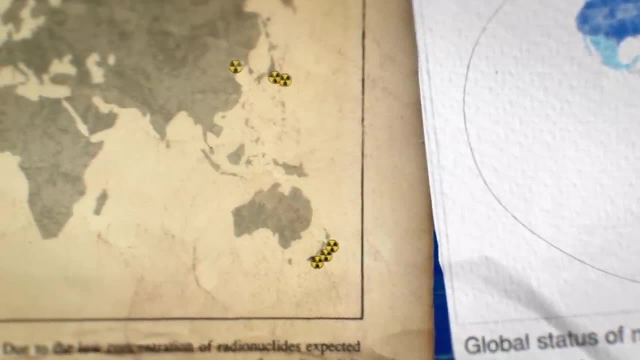 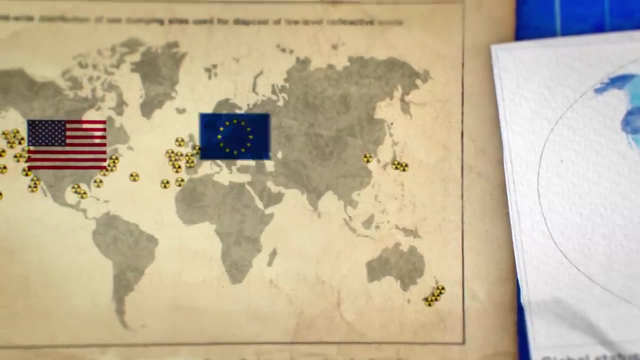 But after a little digging I found that Japan is also responsible for most of these as well. But okay, by now you might have noticed there's something missing on this map, While the US, Europe and Japan are surely responsible for a great deal of radioactive. 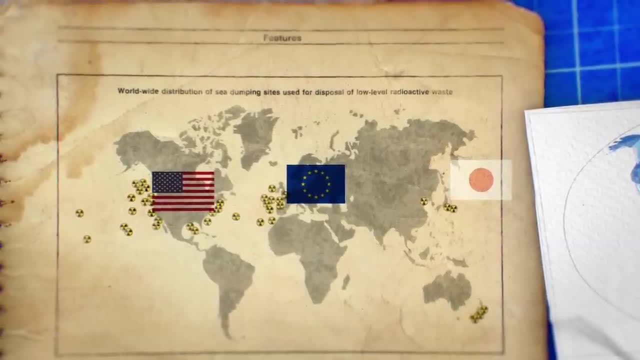 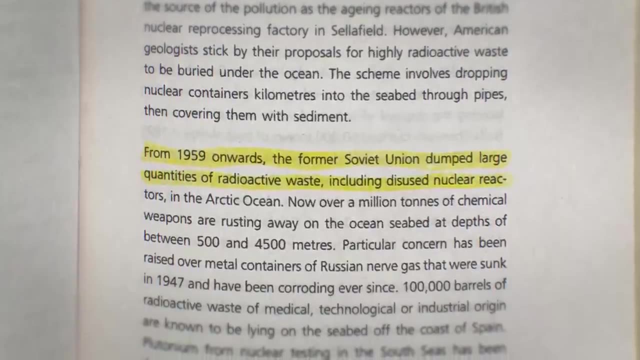 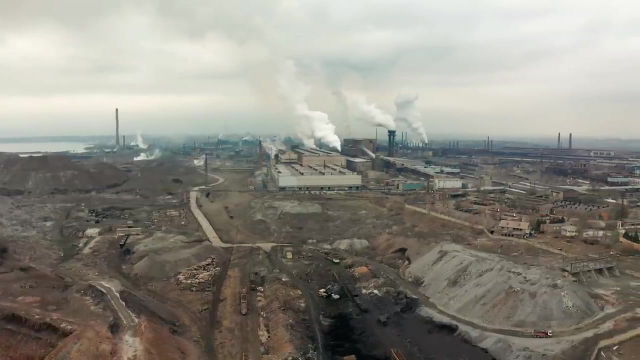 waste. there's one major contributor that's completely absent here: Russia, Or really the Soviet Union. But if that excerpt from the book was any clue, the dumping practices of the Soviet Union were well documented, and by most calculations the USSR accounted for up to two-thirds of all the radioactive waste that reached the ocean. 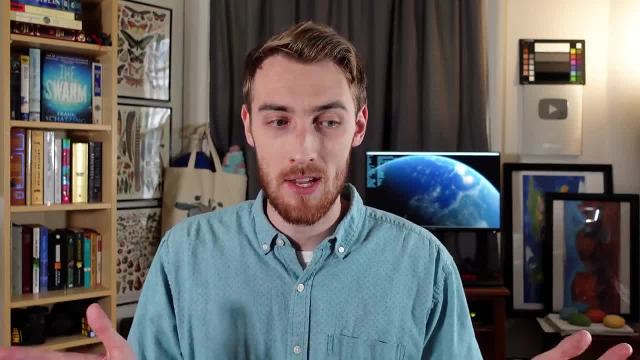 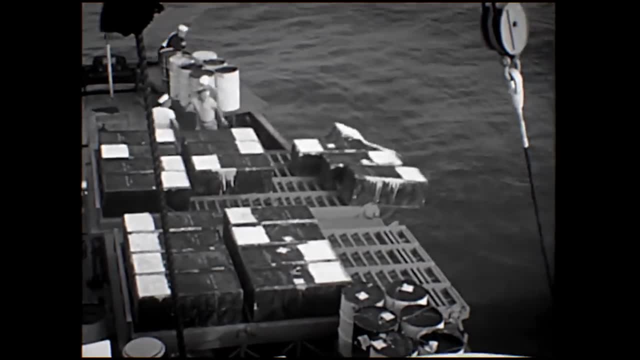 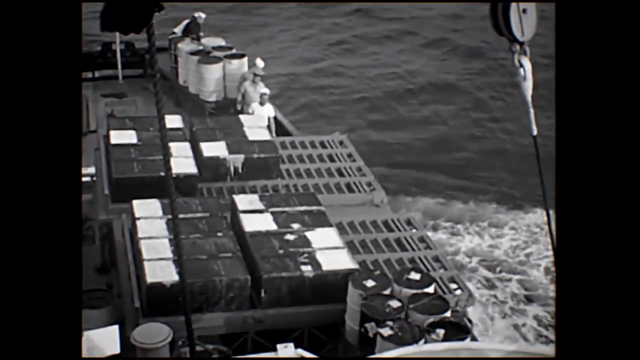 And the real reason none of this shows up on maps is because of how the Soviet Union disposed of this waste. You see, for the most part all the countries we've looked at so far didn't directly dump radioactive material into the ocean, but rather, at the very least, packaged their waste. 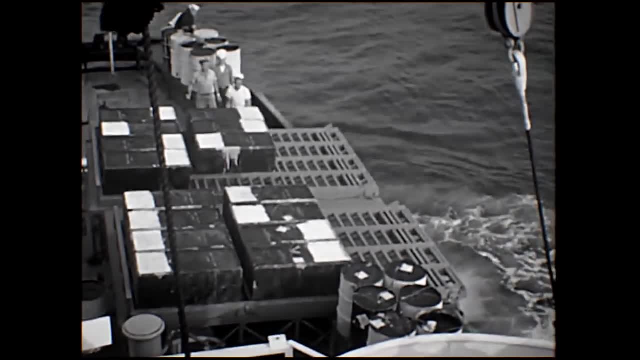 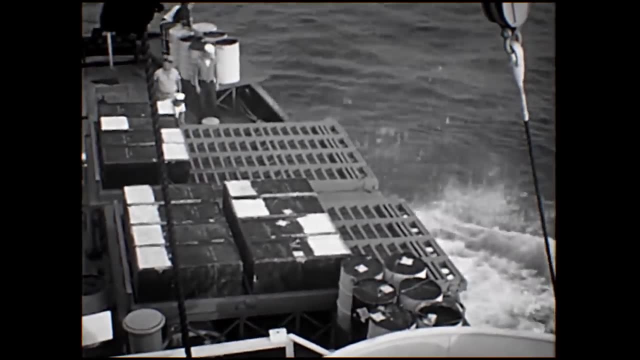 into steel barrels insulated with concrete, which still isn't ideal for reasons I'll get into later, but at the very least this method contains most of the bad stuff inside for the time being. Vacuum pumps used on a radon plant are contaminated to an extent where decontamination. 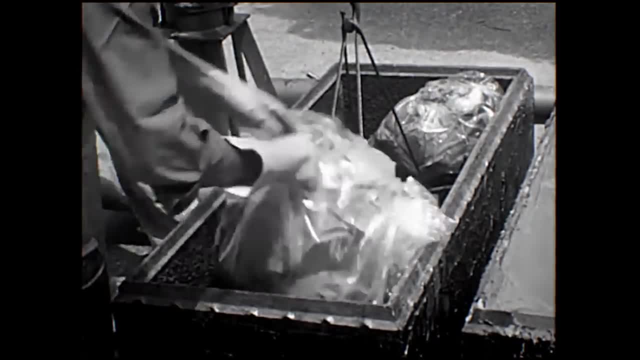 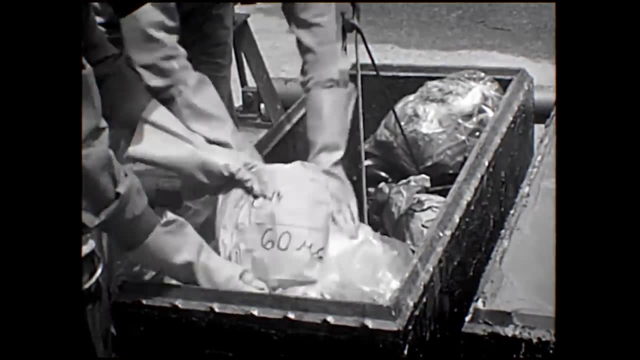 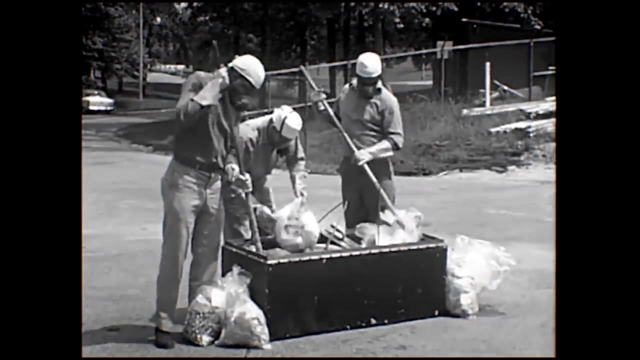 would be more expensive than replacement, So they are disposed of along with other types of wastes. This is a sample of the wastes collected at an institution such as the National Institutes of Health. Waste materials are packed in the concrete burial vaults and mixed intimately with a thin concrete mortar. All of the polyethylene containers. 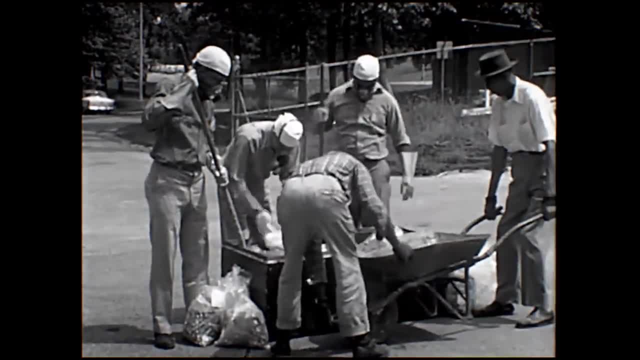 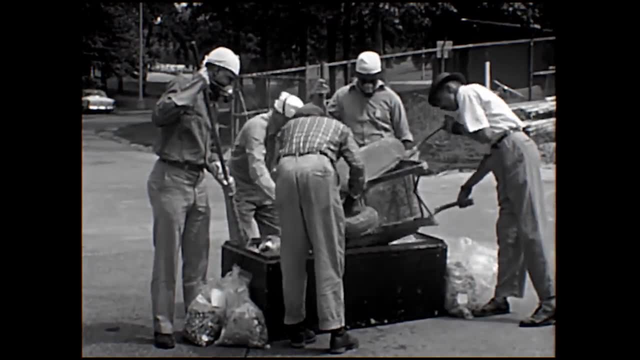 are broken to ensure an intimate mix with the concrete and also to obtain a maximum density to ensure sinking in the ocean. Vaults are shallow enough to permit good mixing of the contents with thin concrete. The safety office personnel working directly over the vaults wear respirators to 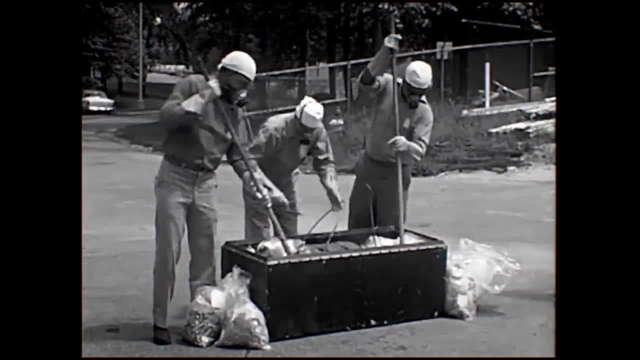 prevent the inhalation of airborne radioactive materials. The vaults are actively agitated during the entire filling operation to eliminate voids and air pockets. The air pockets of the containers are filled with liquid and the air pockets of the containers are filled with liquid. 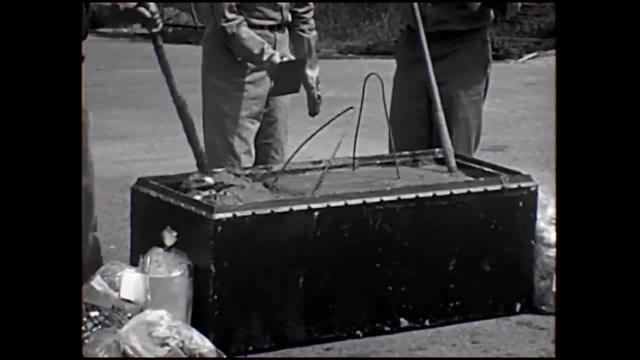 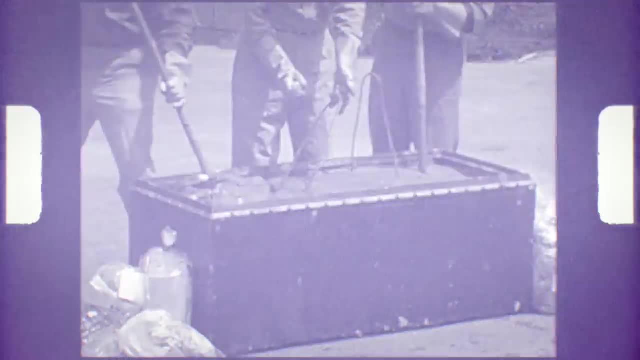 and obtain as intimate mixing as possible. Actual tests show that the finished containers remain intact under the hydrostatic pressures at depths of at least 6,000 feet. The Soviet Union, on the other hand, to put it lightly, did not do this. Instead, most of the 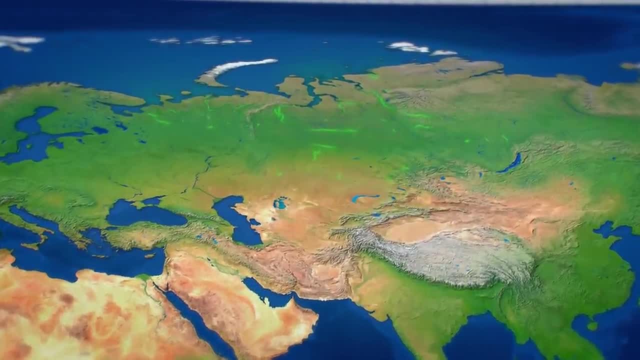 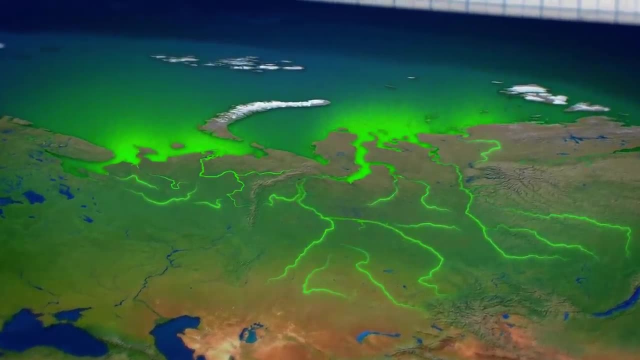 USSR's nuclear waste left its factories and refineries as runoff, released into surrounding areas, where it inevitably made its way into nearby rivers and eventually into the Barents and Kara Seas, spreading radioactive waste throughout the entire Soviet Union. The Soviet Union- 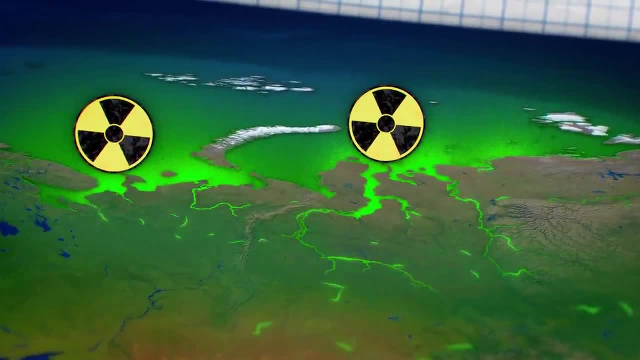 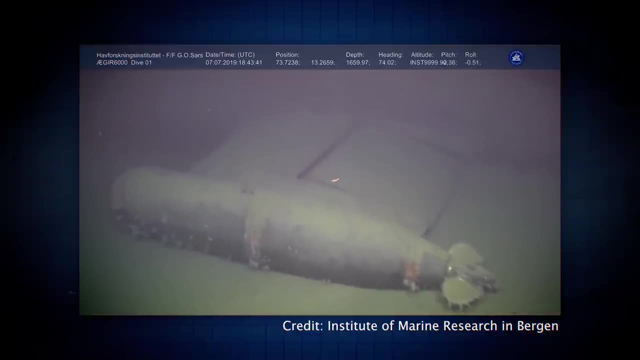 had far more than map from childbirth, which was potentiallyтак señora. a total of nine nuclear submarines have also 당one cause this. struggles начал unintentionally after the collapse of the2005 nuclear gas in the USSR Three by the US. 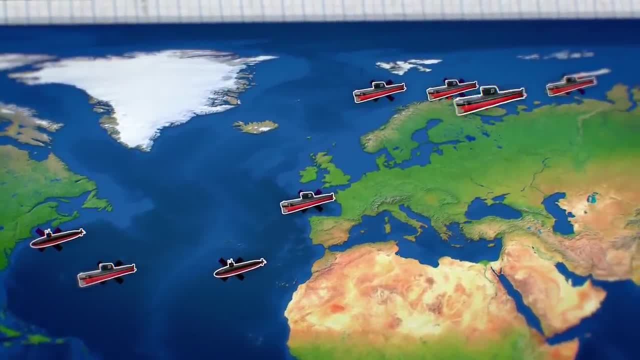 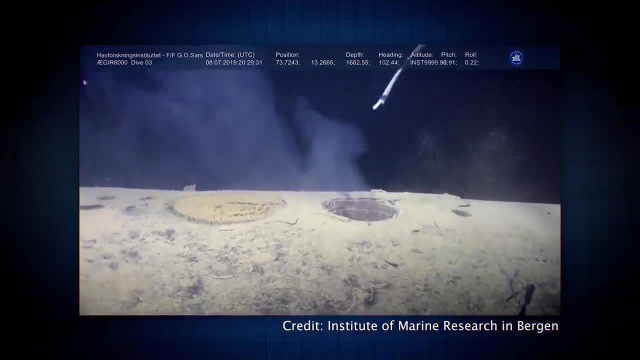 175 by the Soviet Union and 176 by Russia, which have, until recently, has seeking stops, did not follow the needs of the Soviet Union. The Illegal Sanktion of톼낄 Theus espacio anxiety. The USę EH Sank внешний. 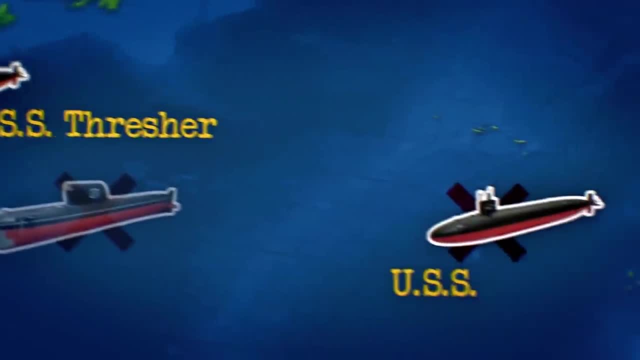 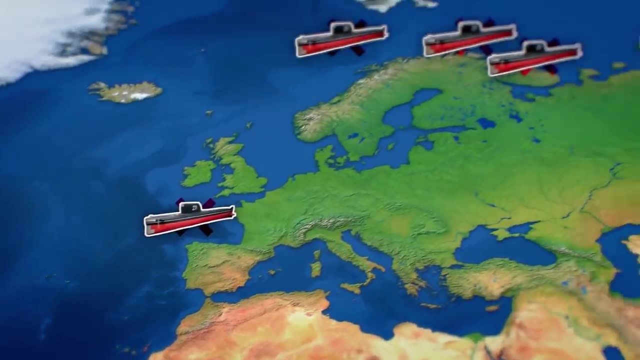 longing Europeç n shouldn't flow away straight. premises饤 Island Pl. Mc25.çN z hoy coast of Cape Cod, while the other, the USS Scorpion, met its end in the middle of the Atlantic Meanwhile, the Russian subs are littered across the North Atlantic and, of course, the Barrens. and Kereses in the Arctic, Because these were all more or less accidents. these submarines still contained active nuclear fuel, thousands of times more dangerous than most low-level waste when they sank, meaning, despite their limited number, these sunken subs still pose a huge threat for contamination. 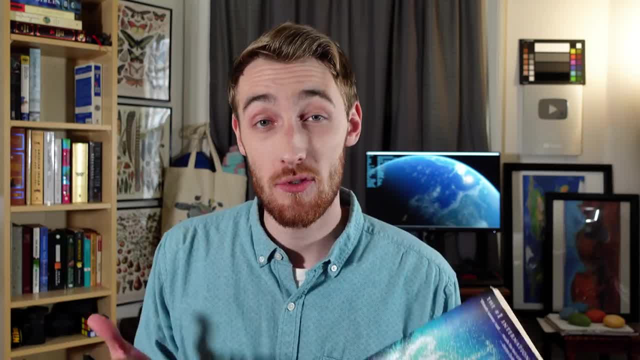 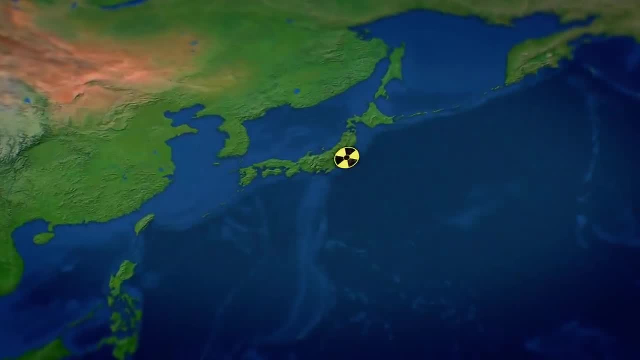 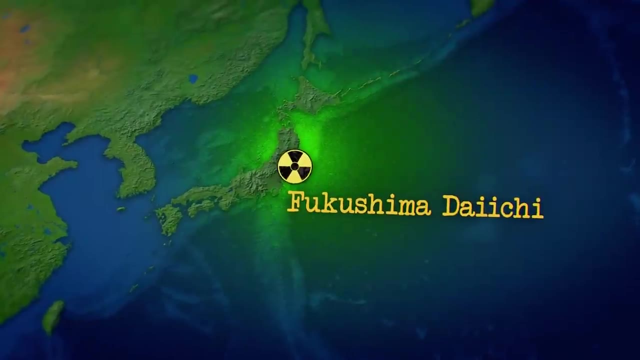 as their containment walls continue to corrode away. And I should remind you that this book was written all the way back in 2004,, meaning it was published well before the worst nuclear disaster to ever befall the ocean: the destruction of the Fukushima Daiichi power plant, in the wake of the 2011 earthquake and tsunami that 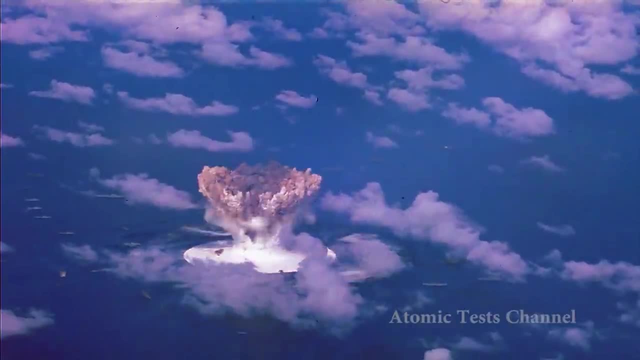 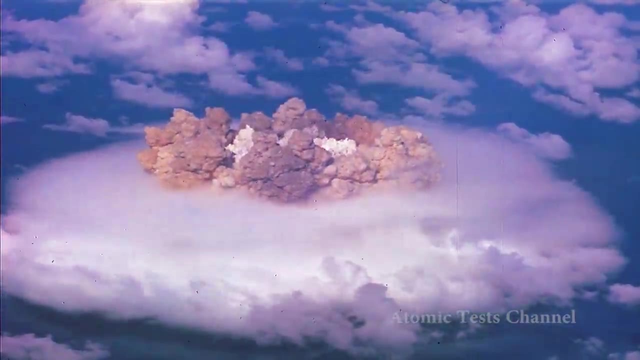 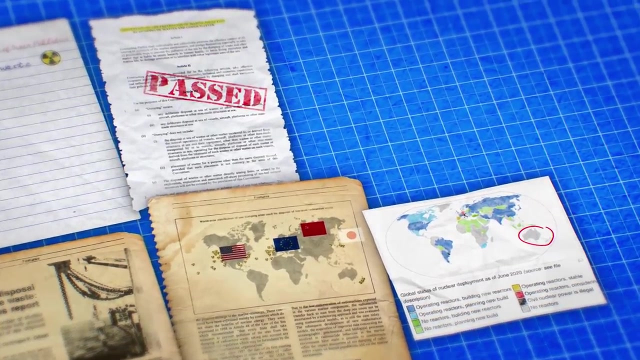 struck Japan, And this is also all without mentioning the countless nuclear bombs that were detonated over ocean water as tests, All of which having left their own fault. Maybe the best method to account for all these different ways radioactive material has entered the ocean is to look at things in simple terms, or, in this case, a list of countries ordered. 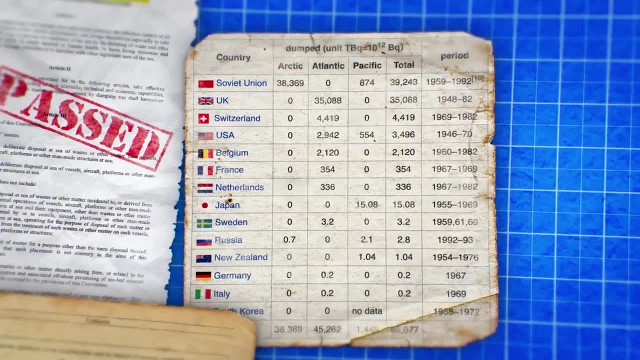 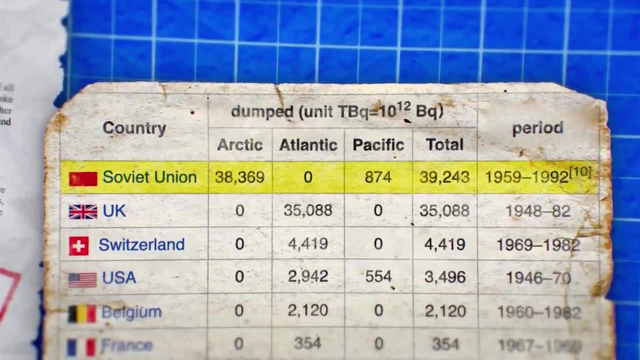 by the amount of waste they've dumped into the ocean. Doing this, we can see that, unsurprisingly, the Soviet Union, not even including Russia, takes the lead. But honestly, the most shocking part of this list might actually be the next two biggest polluters. 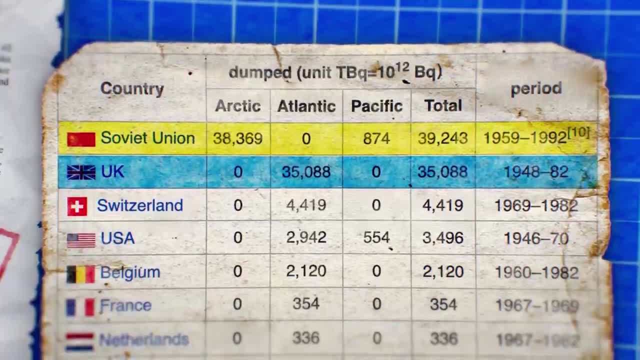 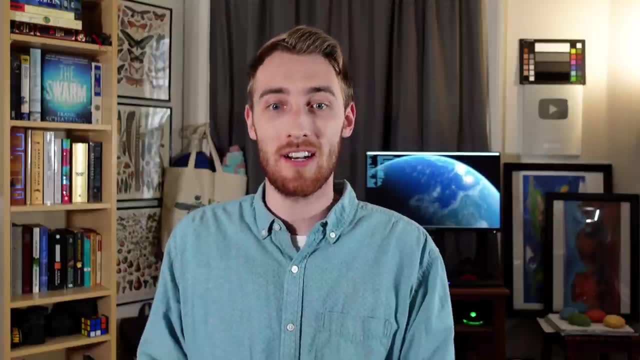 The United Kingdom having put out an almost equal amount of radioactive waste as the entire Soviet Union, and Switzerland coming in a distant third. I honestly could not move on until I figured out why these countries were at the top of this list. but then I remembered what Shotzing wrote. 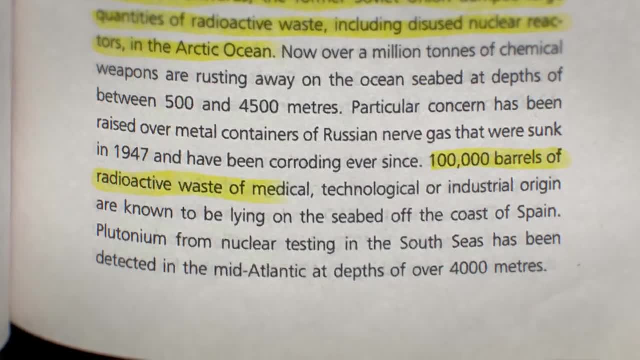 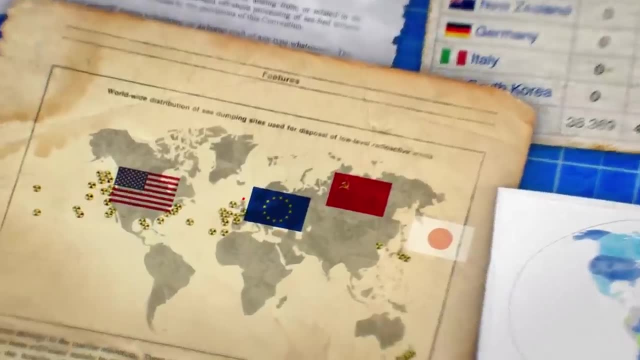 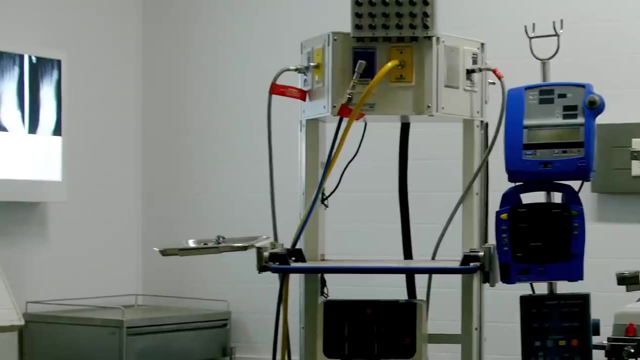 One hundred thousand barrels of radioactive waste of medical, technological or industrial origin are known to be lying on the seabed off the coast of Spain, And I assume these sites were the ones Shotzing was referring to, Speaking more or less off the coast of Spain, and now it all makes a little more sense. 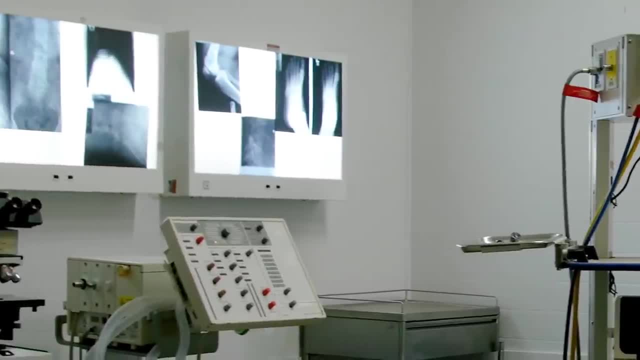 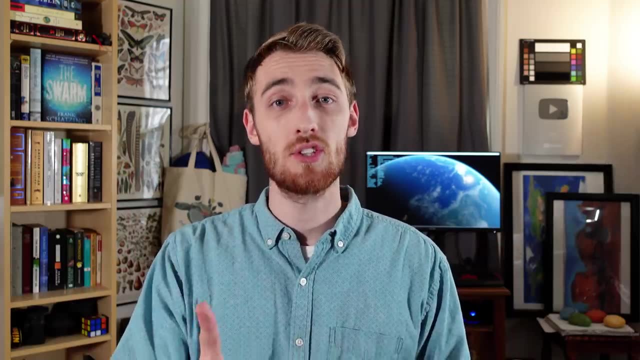 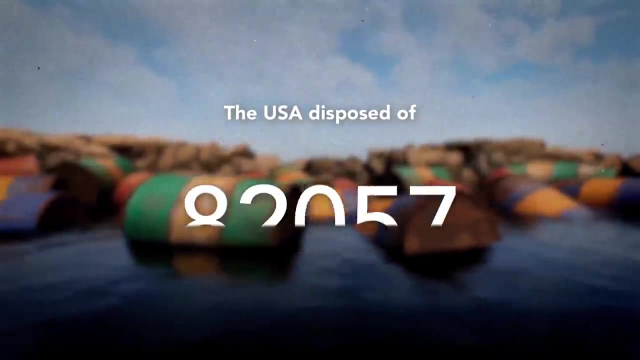 This waste wasn't generated by manufacturing weapons or even harnessing energy, but rather from Europe's booming medical technologies industry. But even still, one big mystery remains: How can the US be so low on this list? Now, okay, I'm no expert, but I suspect it might have something to do with the over 90,000. 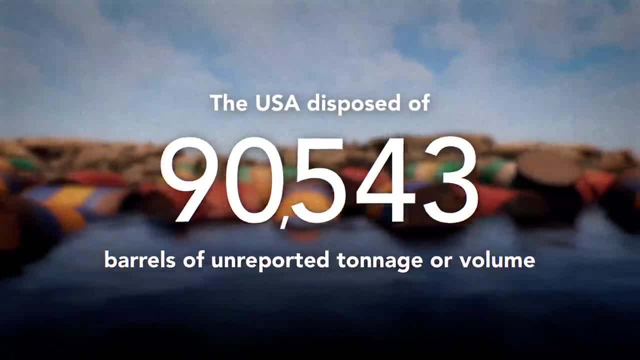 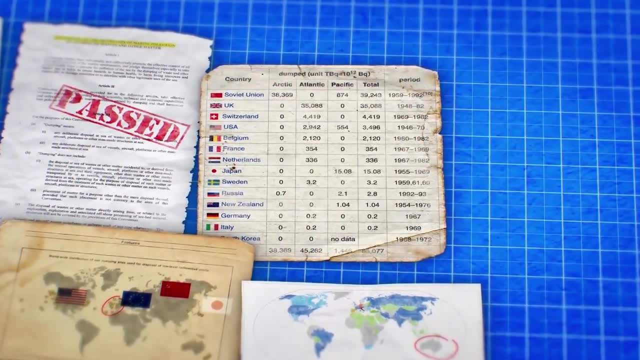 containers with unreported amounts of waste that we dumped, making it really hard for anyone to calculate exactly how much we've dumped in the ocean. Overall, if we consider the European nations together and account for the fact that some of these self-reported numbers may be a little less than accurate, we'll see three major 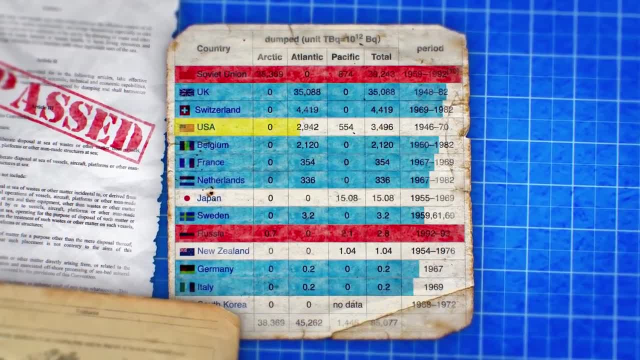 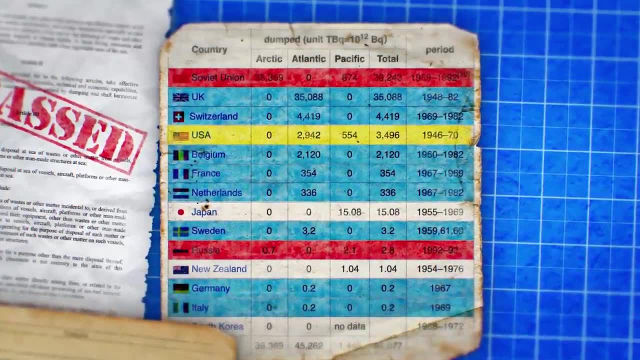 polluters arise: Russia, Europe and the United States, with Japan in a distant fourth, or in other words, basically all the highly developed countries of the world circa 1994, when this activity was finally banned. Moving on, if we check back to our book, we'll see that in the next paragraph, Shotzing. 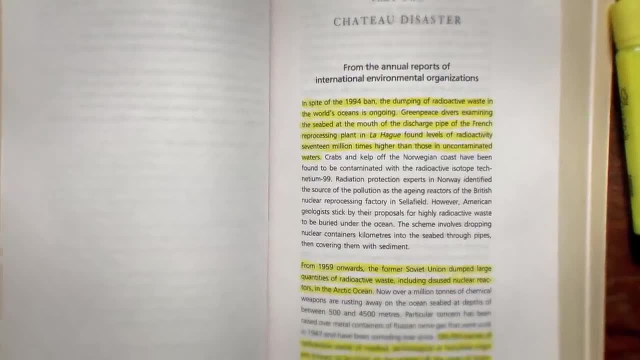 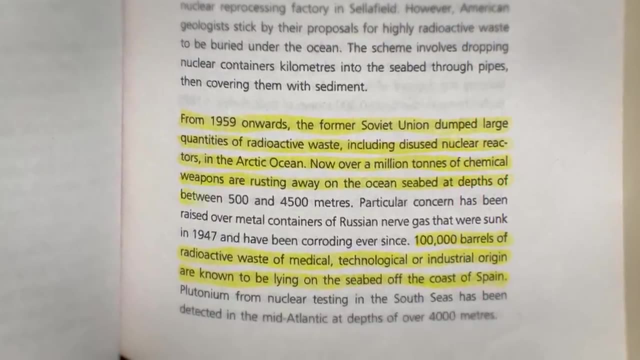 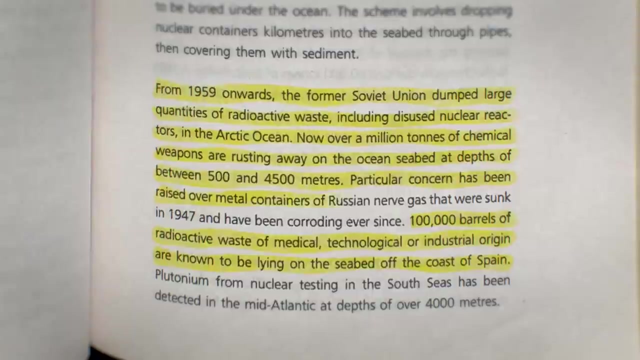 describes for us the second major category of ocean waste by writing. Now over a million tons of chemical weapons are rusting away on the ocean seabed at depths of between 500 to 4,500 meters. Particular concern has been raised over metal containers of Russian nerve gas that were 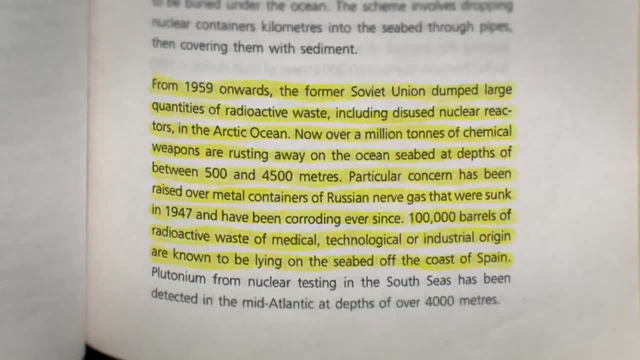 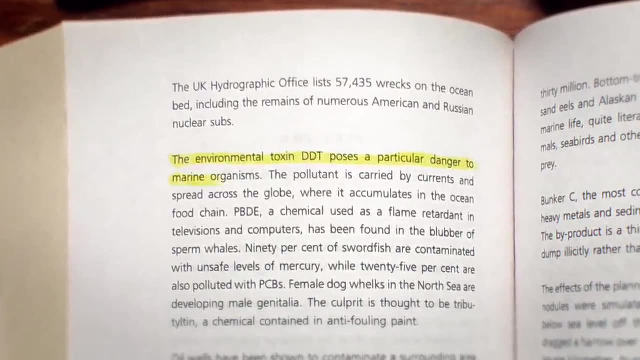 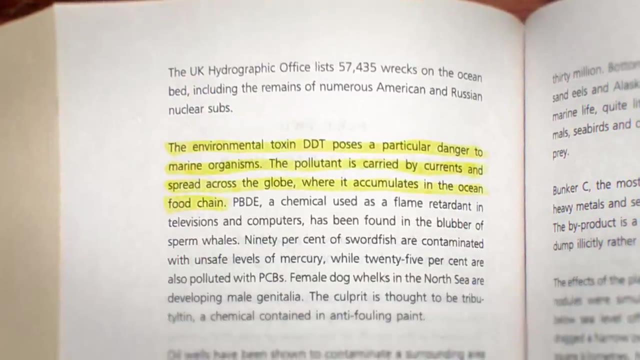 sunk in 1947 and have been corroding ever since. Further down, he continues. The environmental toxin DDT poses a particular danger to marine organisms. The pollutant is carried by currents and spread across the globe, where it accumulates in the food chain. 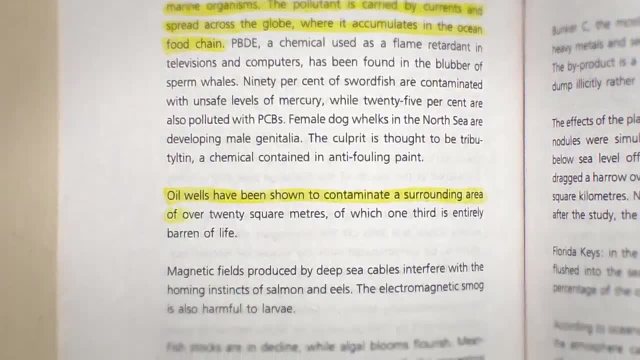 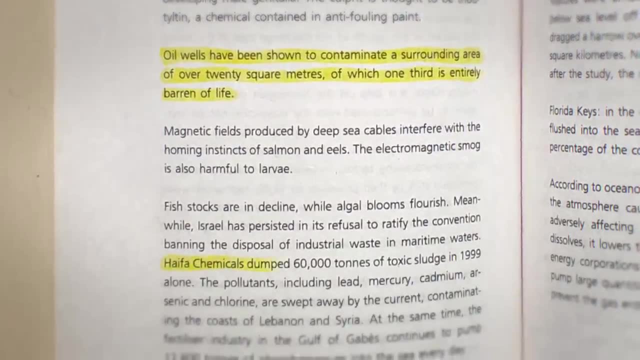 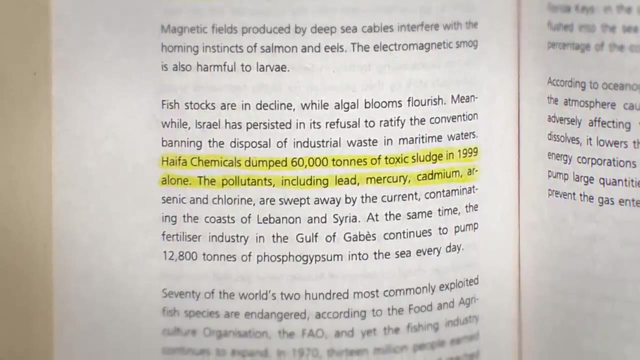 Oil wells have been known to contaminate a surrounding area of over 20 square meters, of which one-third is entirely barren of life. Haifa Chemicals dumped 60,000 tons of toxic sludge in 1999 alone. The pollutants, including lead, mercury, cadmium, arsenic and chlorine, are swept away by the 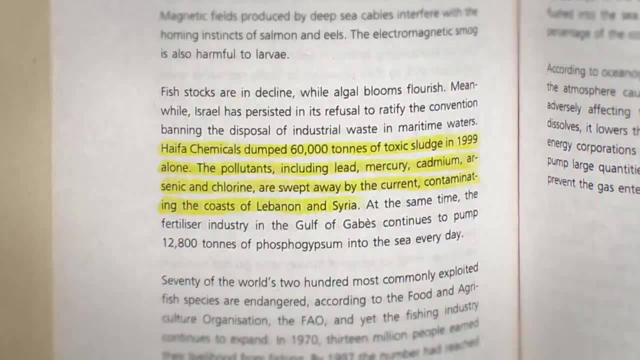 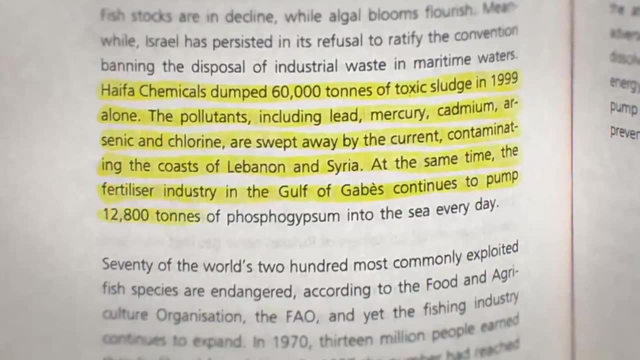 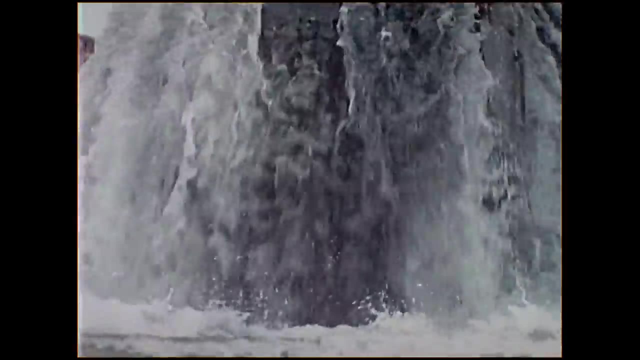 current contaminating the coasts of Lebanon and Syria. And lastly, At the same time, the fertilizer industry in the Gulf of Gabis continues to pump 12,800 tons of phosphor gypsum into the sea every day. The jaws of the dredge stir up blankets of silt and sludge laid down by city sewage and 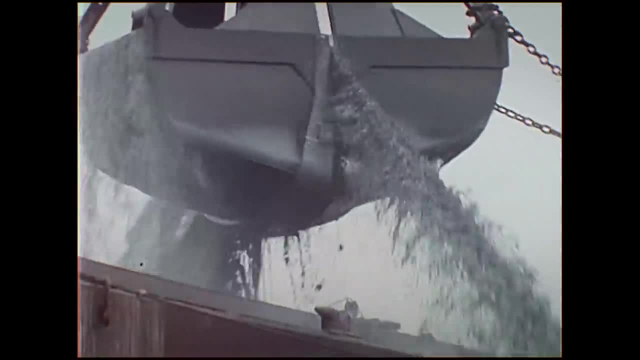 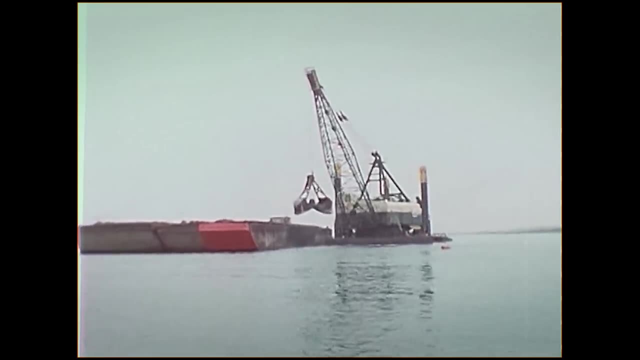 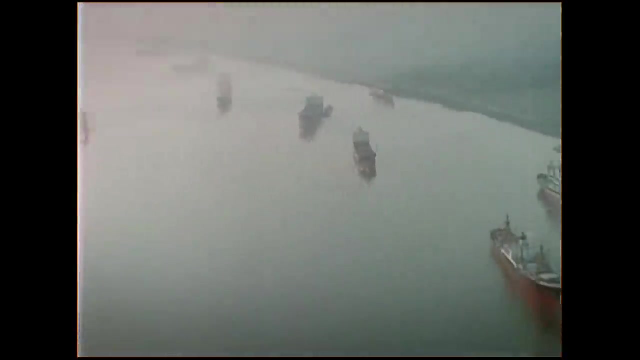 industrial pollution and farm wastes. Dredging, landfill dumping, erosion, the draining of marshes- all destroy the fragile ecology of the estuary. Now even the oceans are polluted. A million tons of oil are spilled at sea each year. 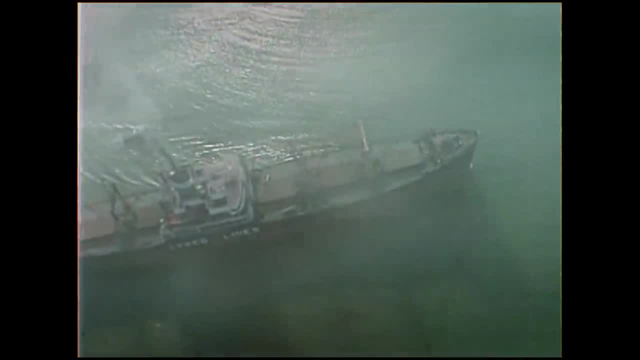 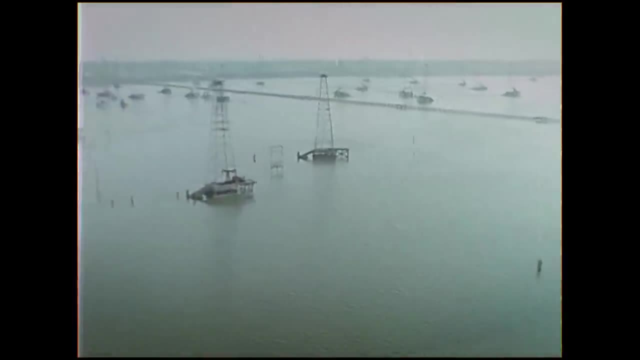 More than 10 million tons are dumped into rivers and bays that run to the sea. Lumps of oil and tar roll in ocean waves throughout the world. Aquanauts report that cans, bottles and other wastes litter the deepest floors of the Atlantic. 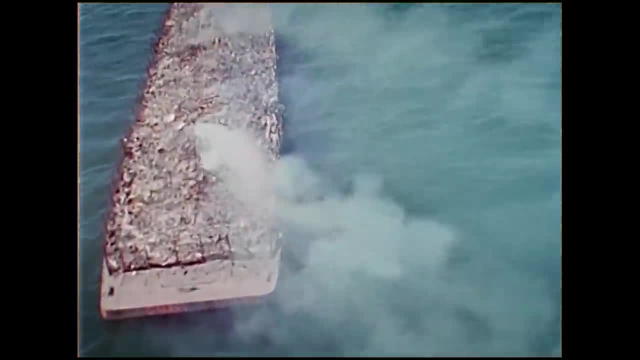 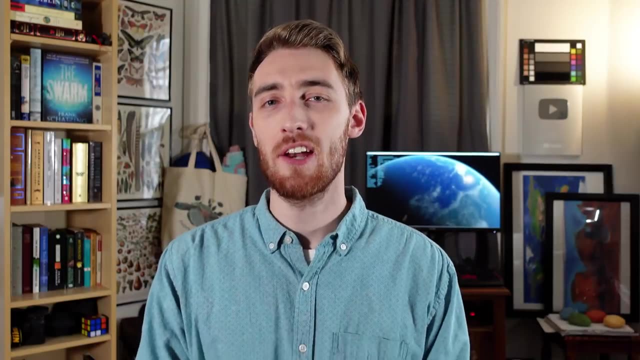 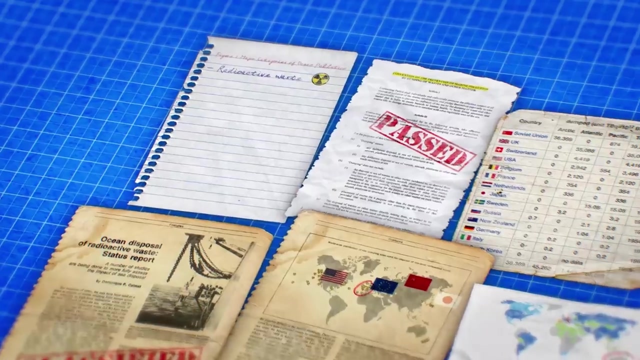 Oil, detergents and water. All of this is polluted. This category was a little harder to categorize, as there are a lot of different substances that we're talking about here, but I think I'm just going to combine these under the 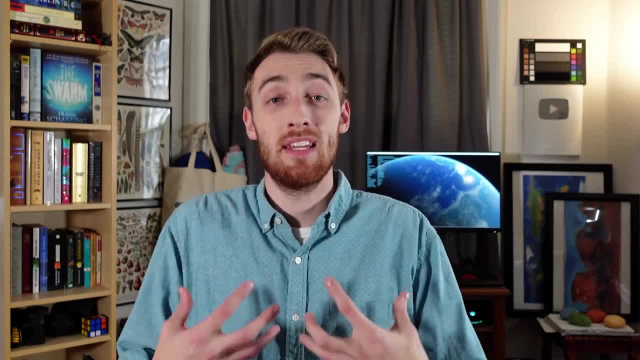 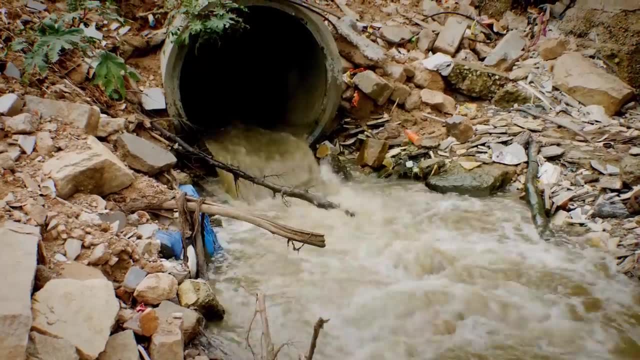 umbrella term, chemical waste, Which in my opinion is by far the most daunting kind of pollution we've unleashed, for a number of reasons. You see… radioactive waste only goes back 80 years, to the 1940s. us humans have been putting random 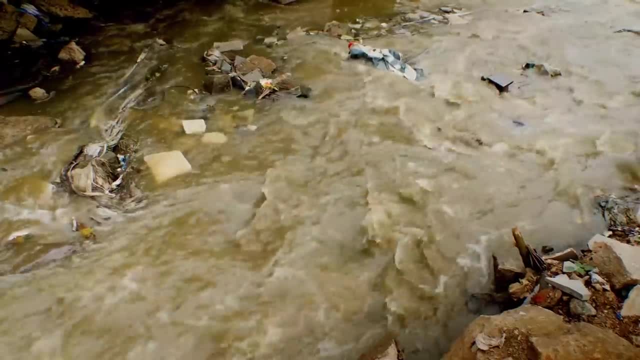 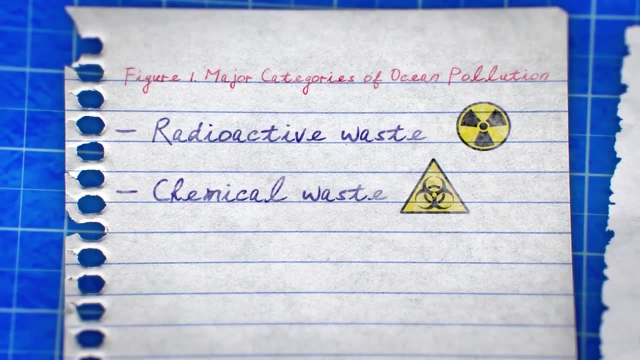 chemicals in the ocean for thousands of years, starting with using rivers and seas to carry away our literal waste and continuing to modern day, where the ocean is used to dispose of horrible things like chemical weapons made for wars that never ended up happening to mass-produced 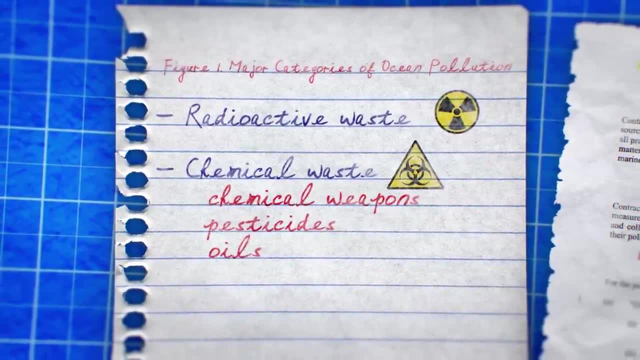 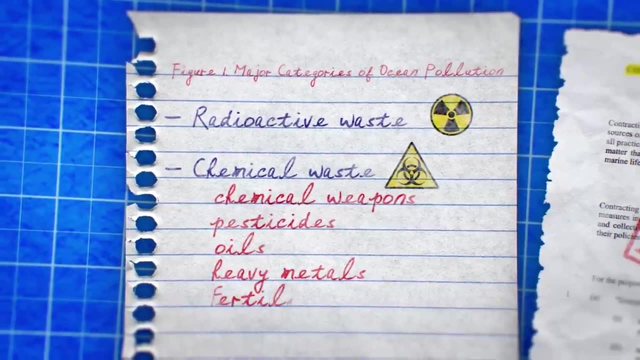 poisons like pesticides, to oils spilled from offshore drilling, to heavy metals like mercury, whose industrial uses inevitably lead to leaking into the surroundings, and fertilizers, which can cause algal blooms followed by massive die-offs- The first of these nasty chemicals to be brought 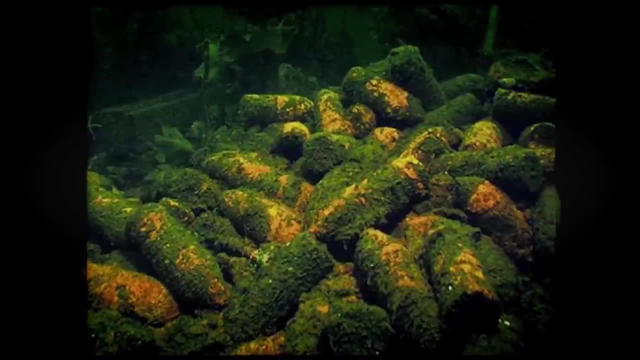 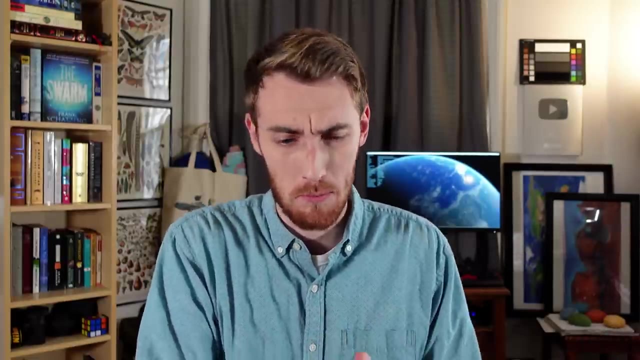 up by the book was chemical weapons, and the example given was nerve gas sunk into the ocean by the Russians. Seriously, though, I think Frank Schatzing just had it out for Russia, because, well sure, the Russians and Soviets certainly dumped tons of chemicals into the ocean. 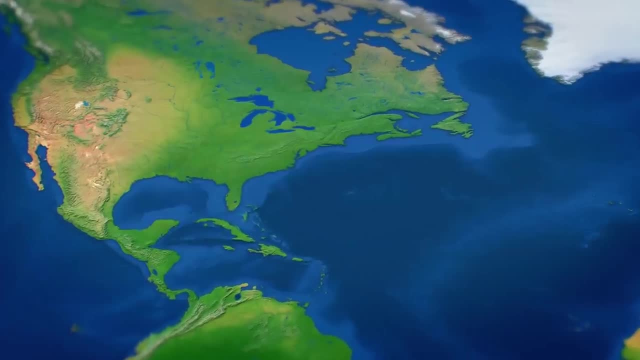 but so did most other developed nations too. The United States, I think, is one of the most developed nations in the world. The United States, I think, is one of the most developed nations in the world. The United States, for example, has dumped mustard gas all along its eastern coast from off the shores of Maine. 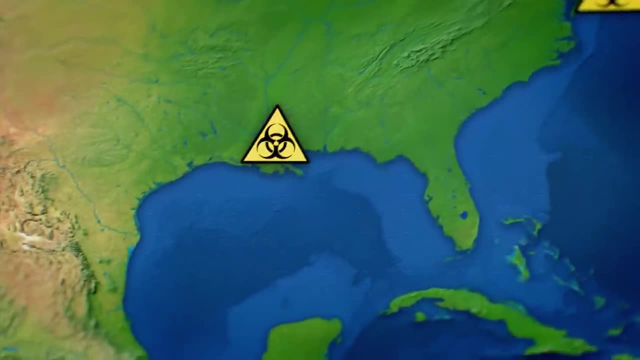 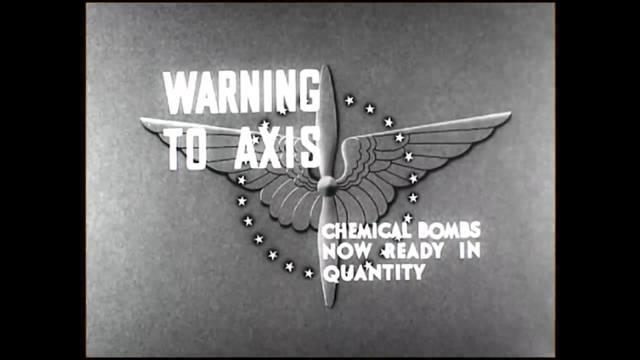 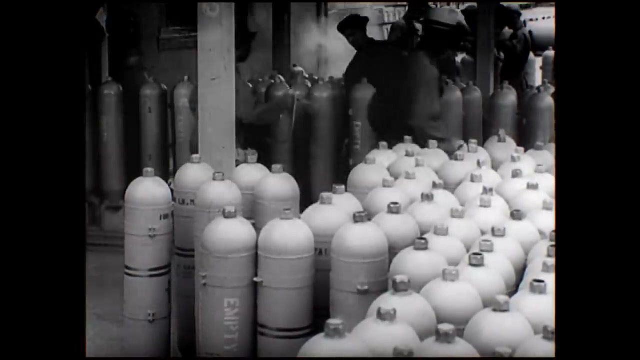 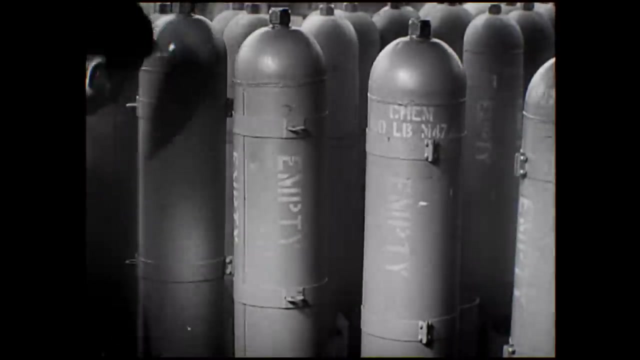 to New Jersey and Delaware, all the way down to the Mississippi River and the Gulf of Mexico, even so far as Panama Warning to the Axis, Deadly mustard gas fills these standard bomb cases, standing ready to meet enemy attacks if and when they come, Ready to make payment in kind, Empty no longer. 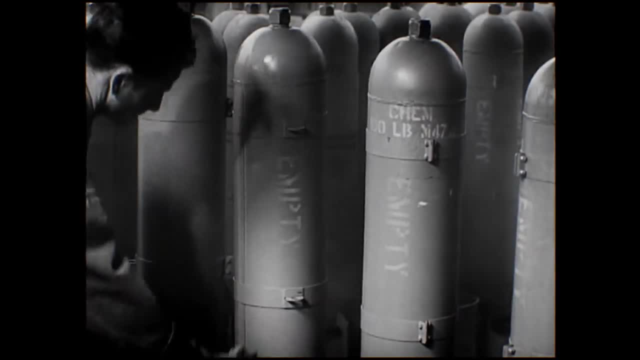 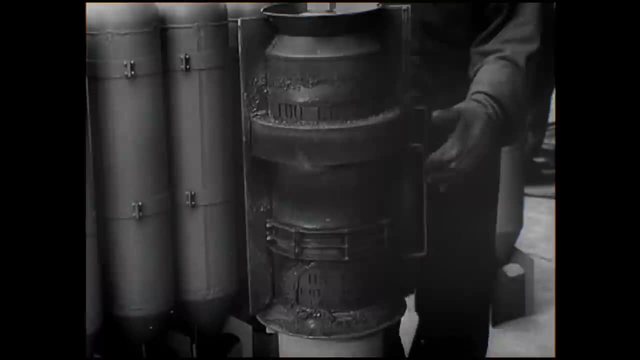 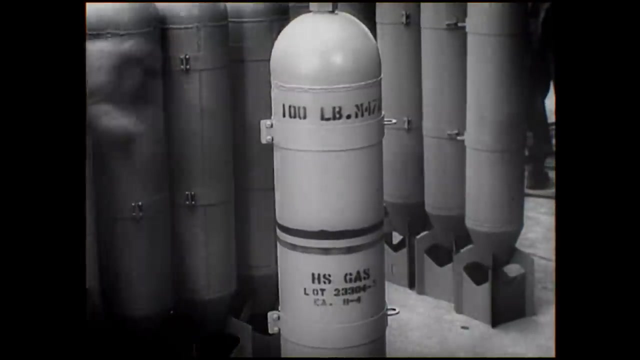 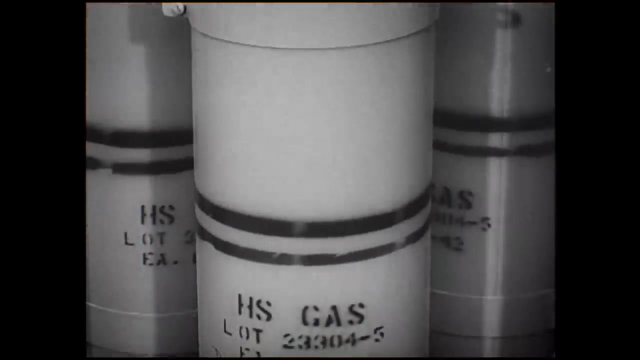 Ready to make payment in kind. Empty no longer. The cases are sprayed a dark gray, Stenciled to tell the world what they contain. 100 pounds of answer to the Axis multiplied thousands and thousands of times 100 pounds of HS. king of battle gasses. 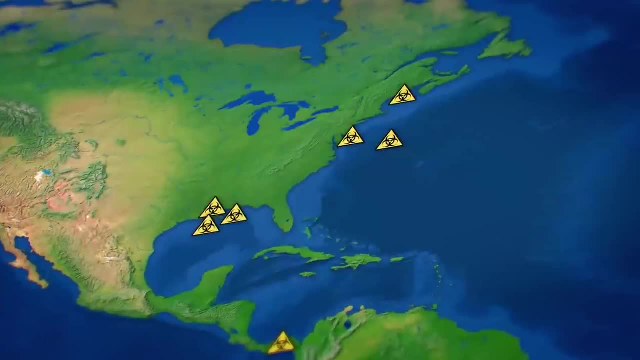 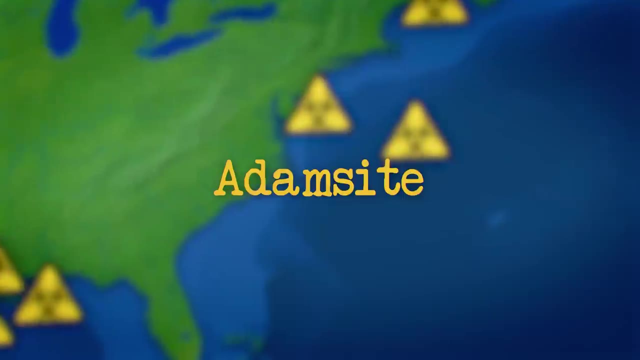 100 pounds of HS king of battle gasses. 100 pounds of HS, king of battle gasses. Of course, that wasn't the only chemical weapon we made in anticipation for a war with the Soviets, and we also dumped what's known as atomcite and leuacite, two equally as bad chemical weapons. 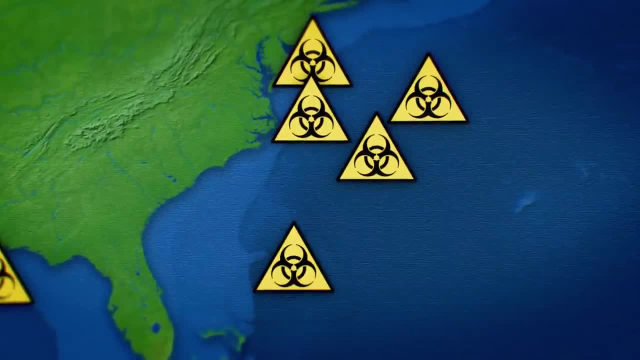 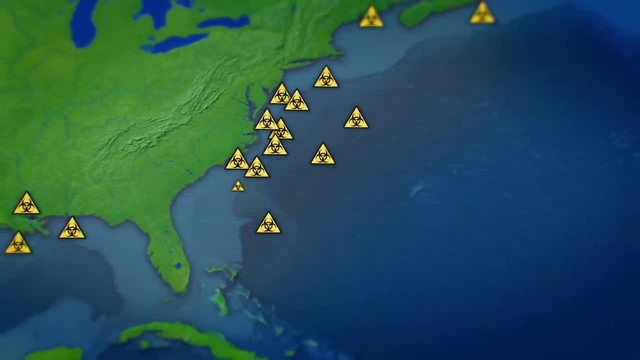 in three locations off the coast of Virginia and Florida. But the real kicker comes when looking at the sites where multiple different chemical weapons, including those mentioned, as well as others like white phosphorus, cyanide, chlorine gas and more, were dumped, littering the entire. 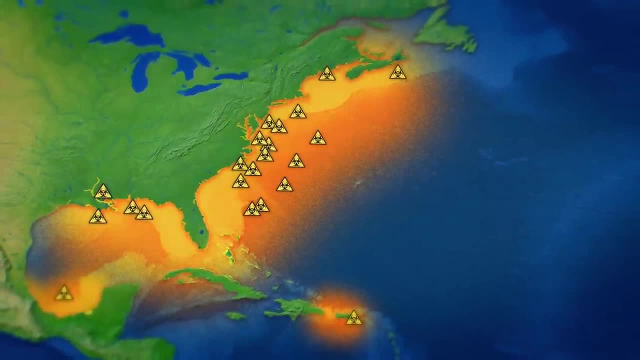 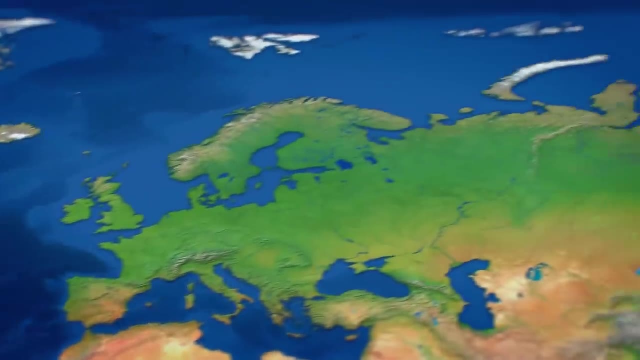 east coast with an arsenal of some of the most important chemical weapons in the world- The deadliest weapons ever made all the way up to Nova Scotia, Canada, and down to Puerto Rico. By comparison, not nearly as many dumping sites of the Soviet Union are known, though there are. 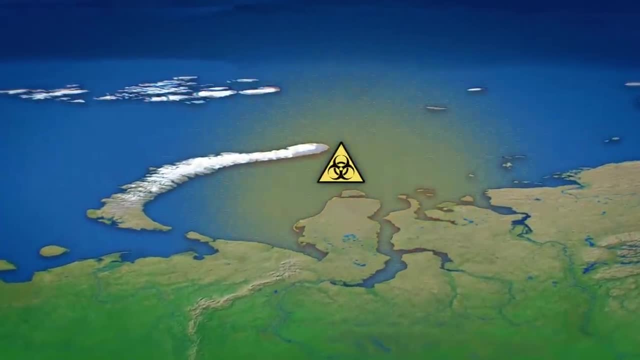 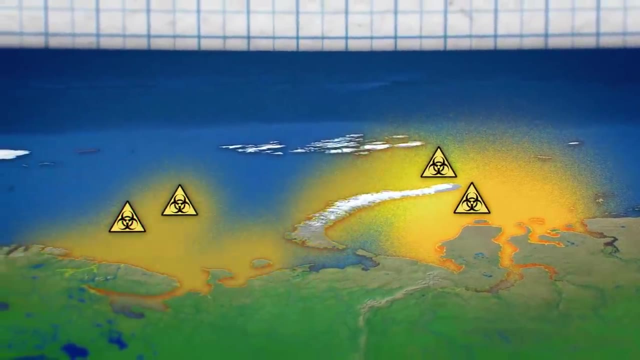 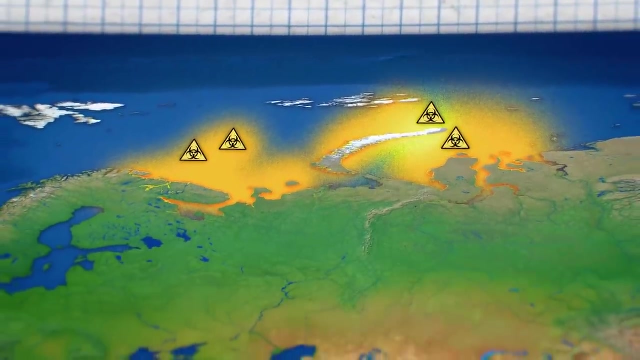 a few like this one again in the Kara Sea, where over 150,000 tons of mustard gas were dumped, along with several more sites in the Barents where more than one chemical agent was disposed of. But don't be fooled: the Soviet Union was huge and had access to a lot more waterways than just the 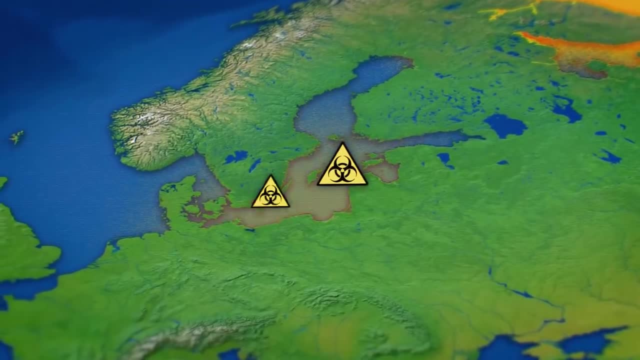 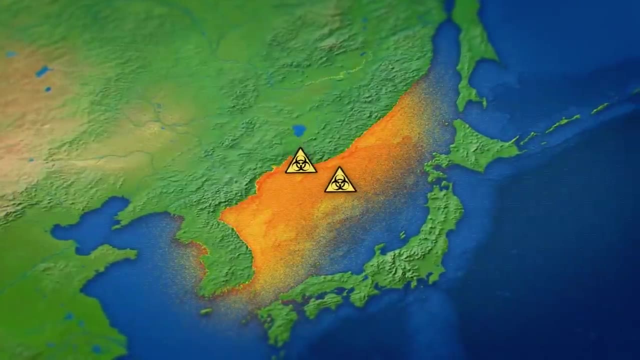 Arctic Ocean, and so additional chemical weapons are thrown out across multiple sites in the Baltic Sea, the Black Sea and even all the way over in the Sea of Japan. Of course, Japan had its own assortment of chemical weapons to get rid of after the Second. 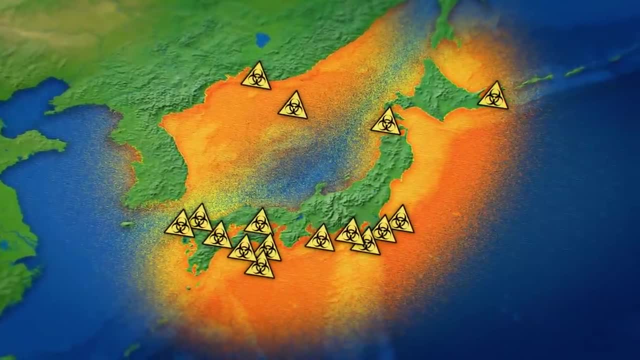 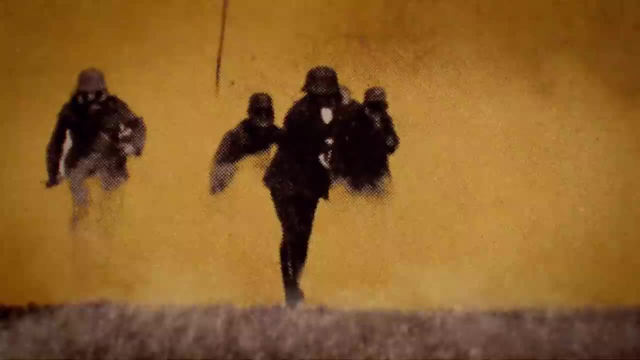 World War, again littering the island's east coast with over ten sites where multiple different agents were disposed of. But this time it's Europe that really takes the cake, After having actually employed the large-scale use of such weapons during the First and Second. 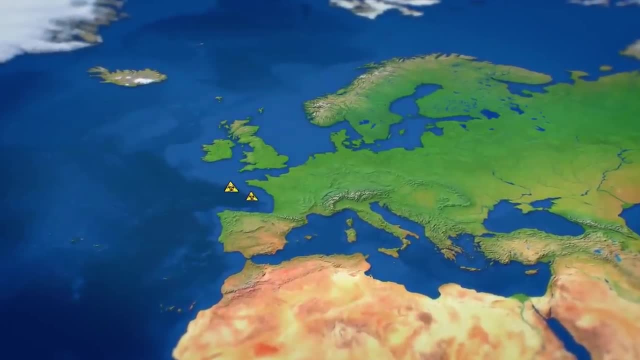 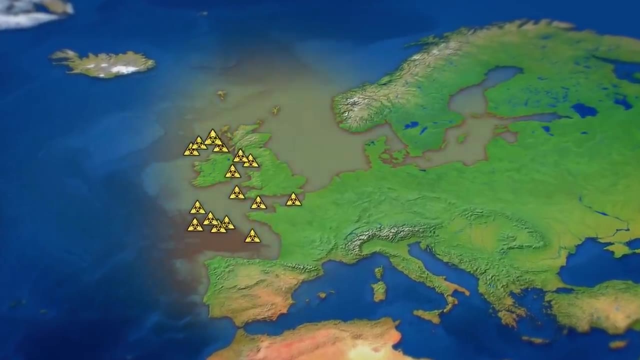 World Wars, there was a lot to get rid of, most of which was confiscated from the no-no Germans after their defeat, where the responsibility of disposing of these agents fell onto the shoulders of the Allied powers and really mostly the United States, leaving countless. 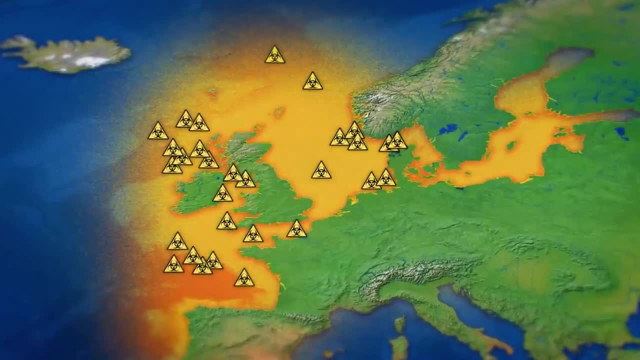 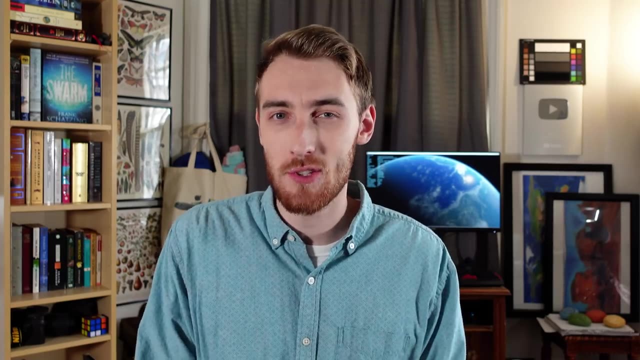 sites all across the Baltic North and Celtic Seas full of the worst chemical weapons 1940s German scientists could produce. And when I say countless… Countless, what I mean is that I literally tried counting them all and I just couldn't. 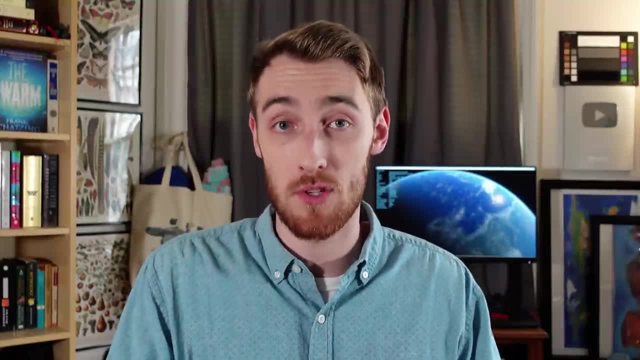 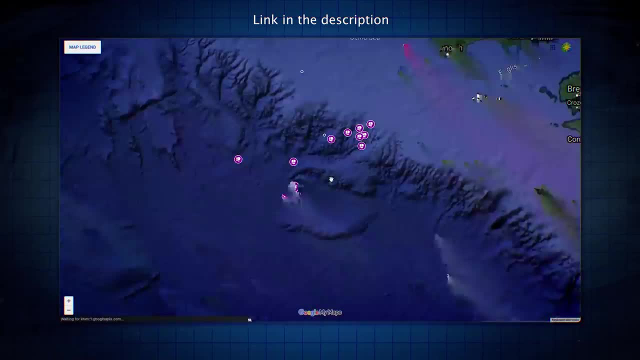 But if you want to learn more about where these weapons were dumped- how much was dumped, when and by who- I actually found this fantastic interactive map you can use to explore the wonderful world of chemical weapons dumping. A link for it will be in the description and you can see for yourself how what I've mentioned 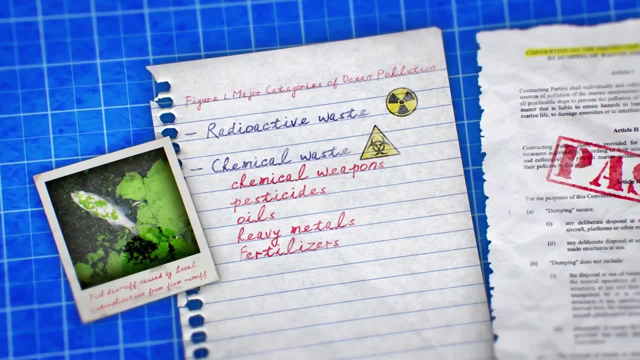 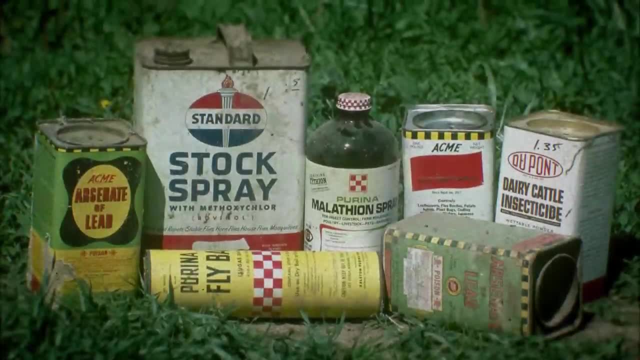 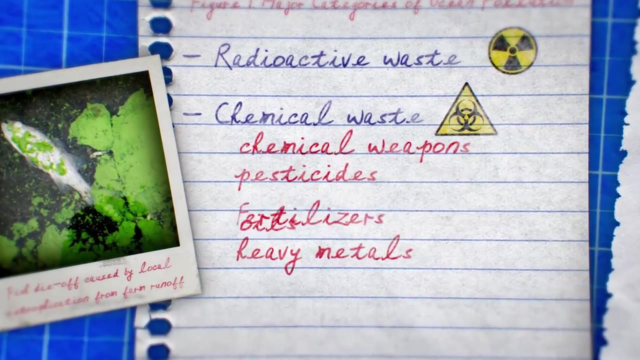 so far really only scratches the surface. Of course, chemical weapons were only one facet within our much larger chemical waste, and the second example our book gave for this was the release of a pesticide known as DDT. To make things simple for us, I'm going to lump these in with fertilizers. 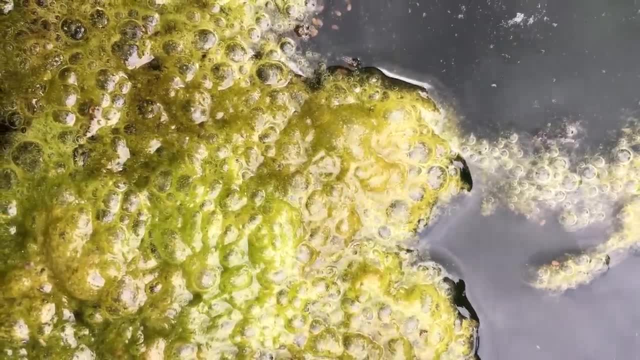 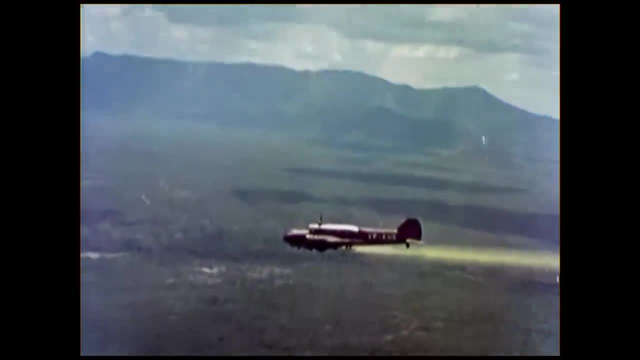 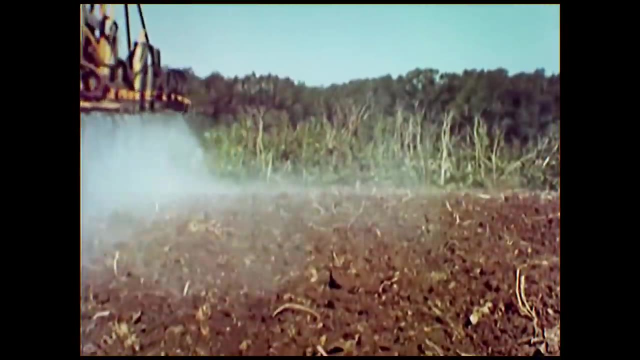 Although they have drastically different- even opposite impacts when released into the environment, they both originate from the same places: Farms. Man fights back. His early victories were astonishing. Yet within five years, the first resistant insects were reported. New pesticides, New pesticides. 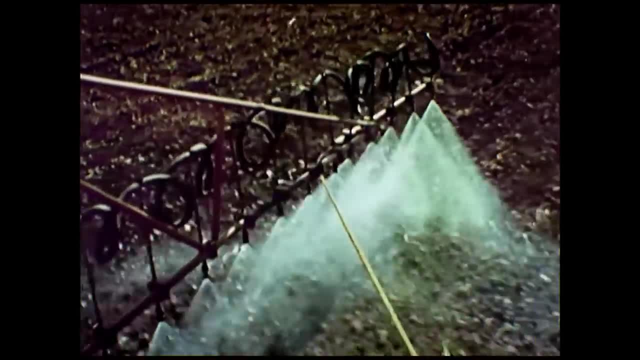 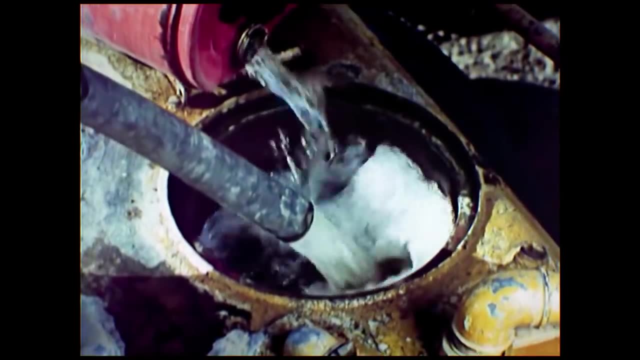 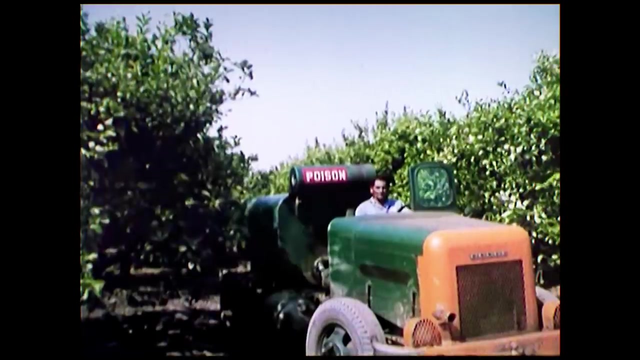 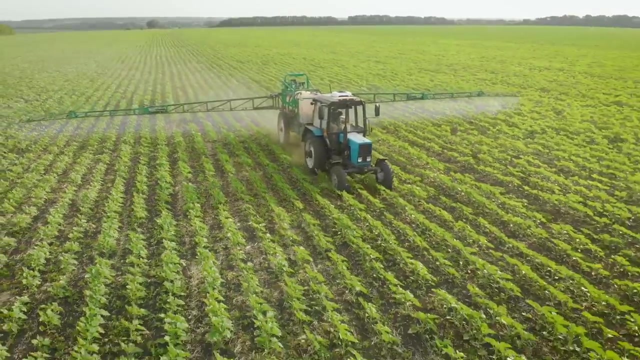 More spraying. But now a second problem began to emerge: In terms of human hunger, we were gaining, But in terms of harm to wildlife, we were losing. Unlike most nuclear waste and chemical weapons, these chemicals aren't typically packaged and dumped into the ocean. 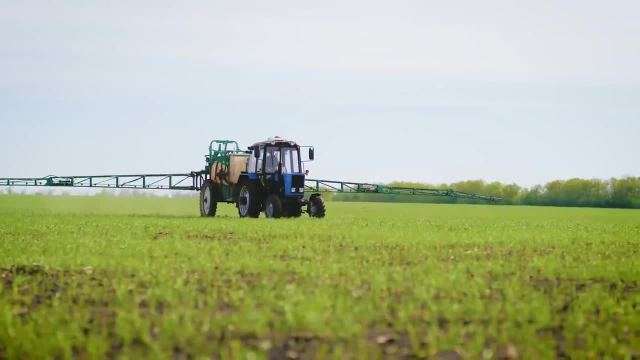 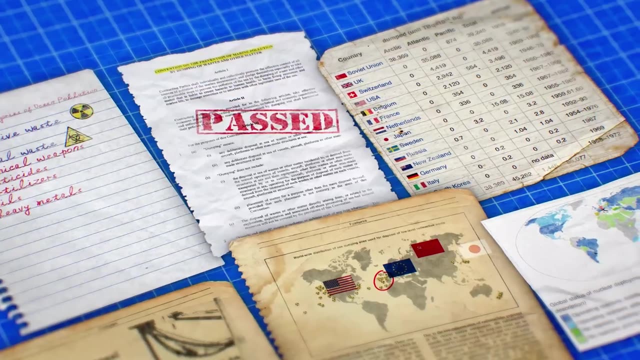 But rather they're typically sprayed onto fields and carried away by rain into rivers and, yeah, eventually the ocean, again making them virtually impossible to clean up. However, if I had to guess the reason, DDT of all the pesticides was the one mentioned. 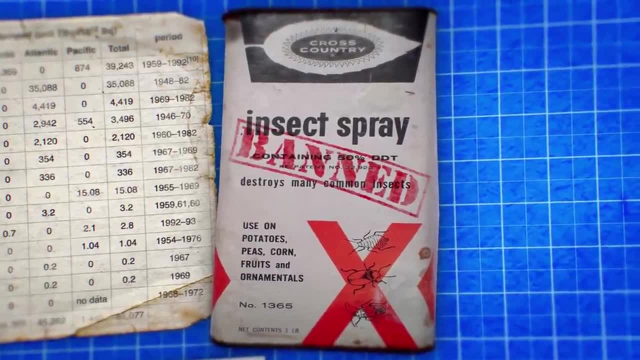 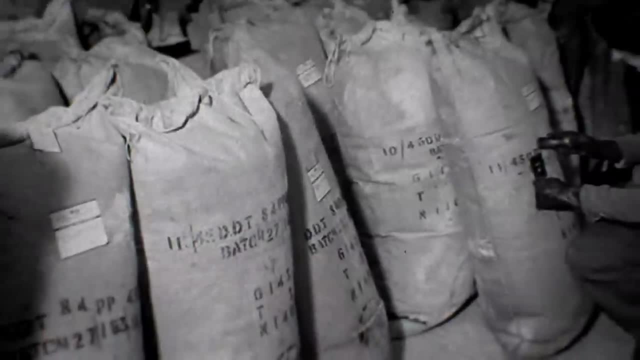 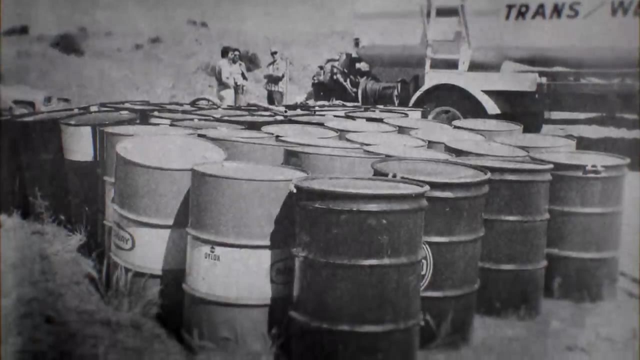 is because of how abruptly it was banned after it was discovered just how harmful it was to wildlife, Meaning industrial chemical companies, almost overnight, needed to get rid of literal tons of what had become a worthless chemical. This led to the pesticide being poured into containment barrels just like if it were. 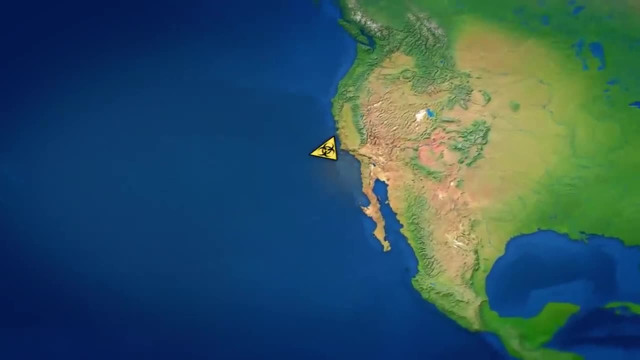 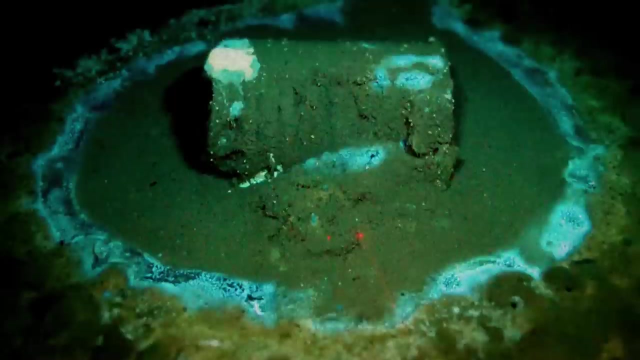 a chemical weapon- which I guess technically it is- and was dumped off the coast of California, where now up to half a million of these barrels are known to be sitting on the ocean floor. To make matters worse, an exploratory trip to some of these barrels just earlier this. 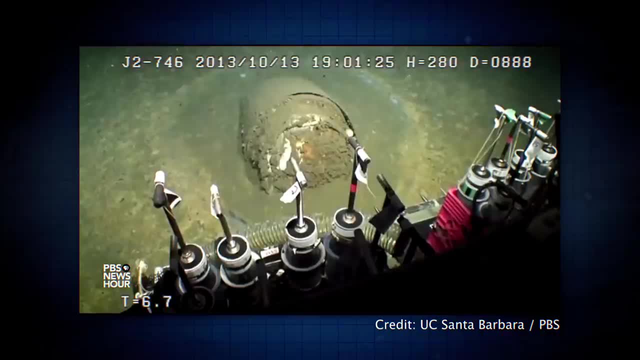 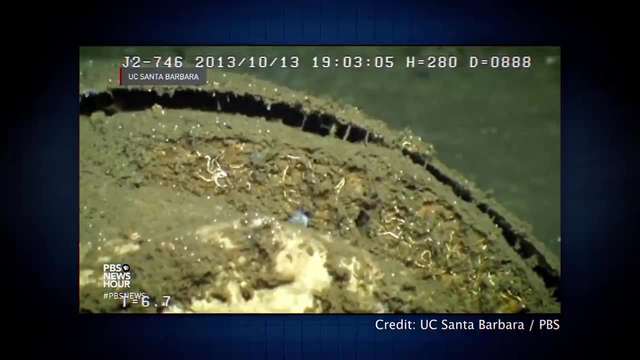 year revealed that they'd already begun to corrode and leak, something we can assume is happening to not only these, but really all the barrels used to dispose of waste we've seen so far. As time goes on and more and more of these barrels break down, they'll begin releasing. 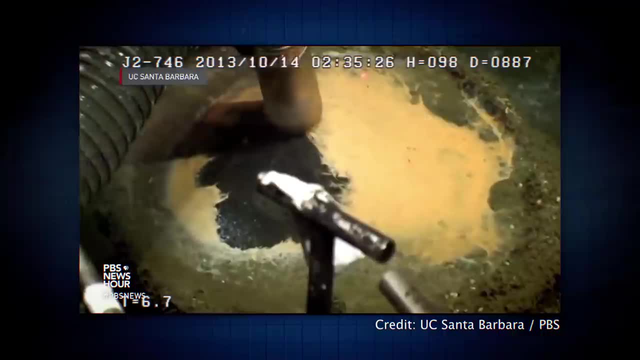 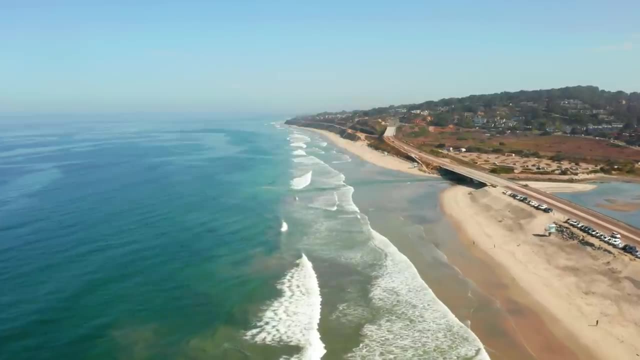 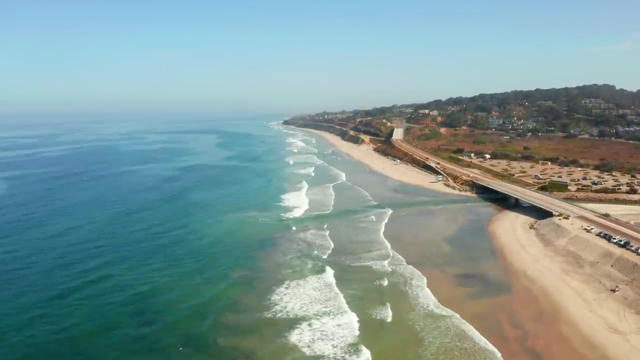 their contents into the environment, and whether it's nuclear waste, chemical weapons or pesticides, they're all designed for the same purpose: killing- And so that's exactly what they'll do as they start entering the waters directly off our coast: killing plants, killing fish, killing beaches, killing tourism economies, and yeah. 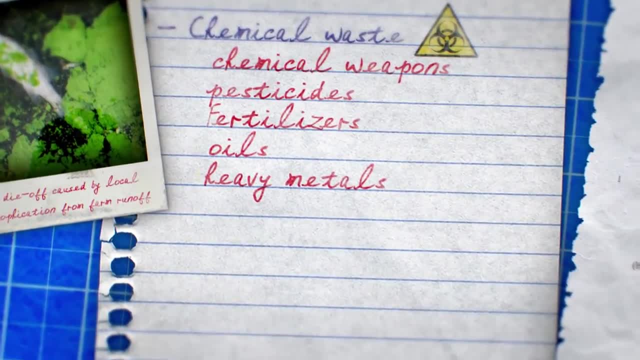 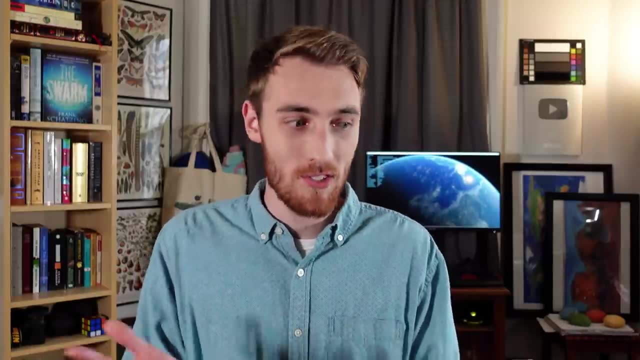 killing us. Okay, In terms of chemical waste, we have oil and heavy metals. While I wish I could go into more detail for these, this video is already getting pretty long and we still have more categories to get to, so just take my word for it. these 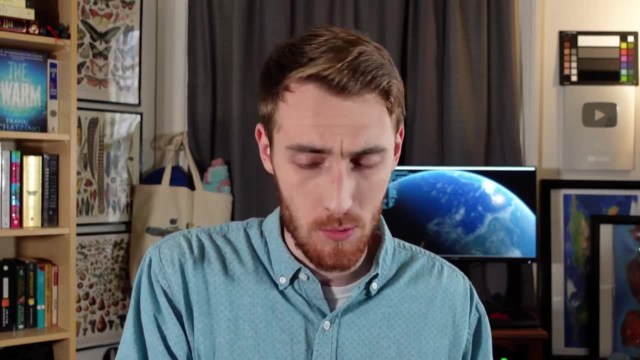 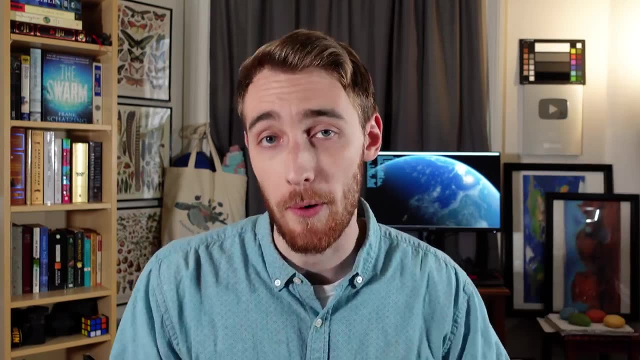 are also a huge problem. we've all witnessed oil spills and we've all heard about mercury poisoning fish, So let's move on and see the last major pollutant Schatzing included in his report. According to oceanographers, rising levels of carbon dioxide in the atmosphere caused 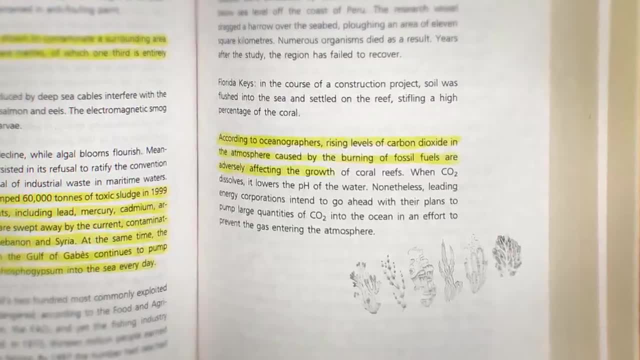 by the burning of fossil fuels are adversely affecting the environment. According to oceanographers, rising levels of carbon dioxide in the atmosphere caused by the burning of fossil fuels are adversely affecting the environment. According to oceanographers, rising levels of carbon dioxide in the atmosphere caused 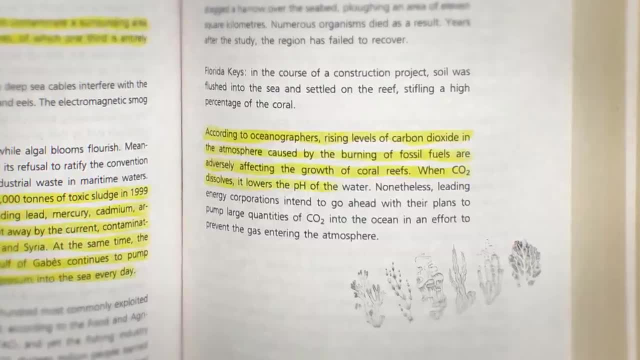 by the burning of fossil fuels are adversely affecting the environment. When CO2 dissolves, it lowers the pH of the water. When CO2 dissolves, it lowers the pH of the water. Nonetheless, leading energy corporations intend to go ahead with their plans to pump. 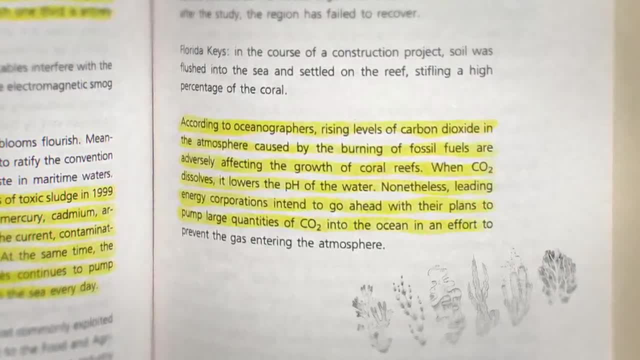 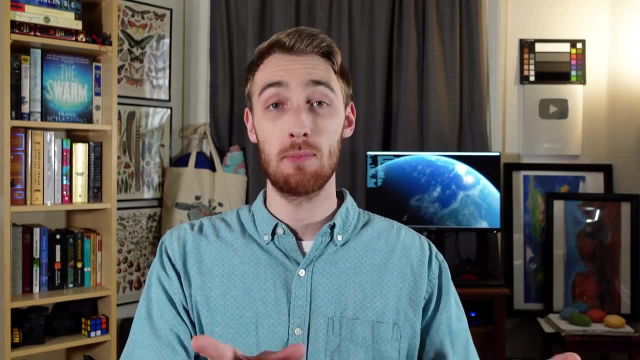 large quantities of CO2 into the ocean in an effort to prevent the gas entering the atmosphere. Okay, so this category we can call atmospheric pollutants and, trust me, carbon dioxide is by no means the only example of this. Virtually every gas we produce is a byproduct of energy production, transportation and 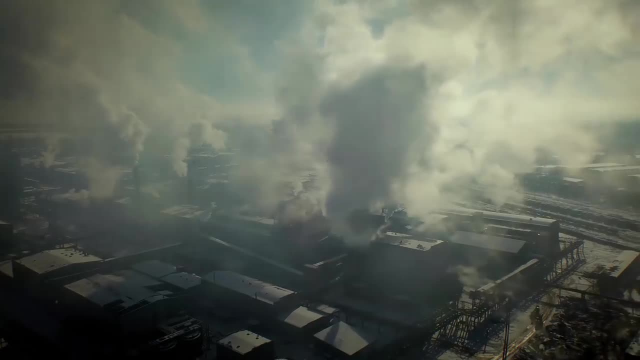 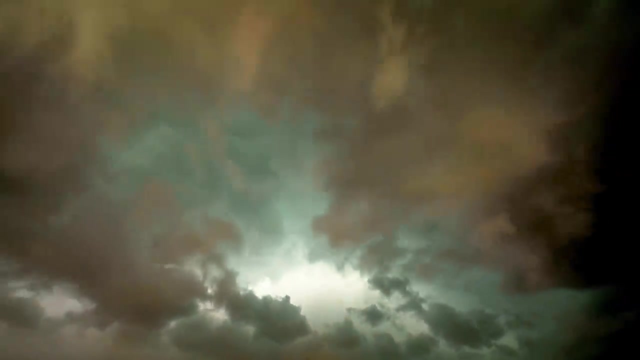 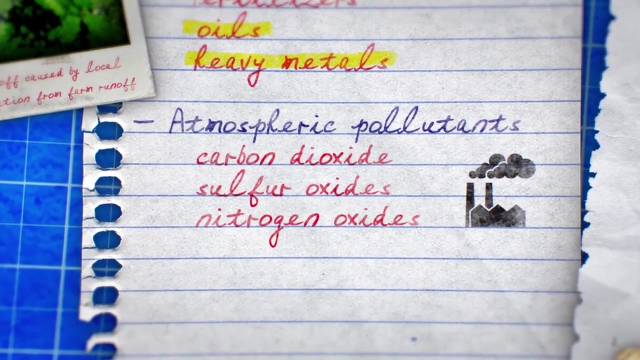 energy consumption. That's why we have so many of these- transportation, agriculture and more all end up in our atmosphere and from here can dissolve into rain droplets, where they eventually fall back to the surface as acid rain. This includes gas groups like sulfur oxides and nitrogen oxides, which become sulfuric acid and nitric acid upon entering. 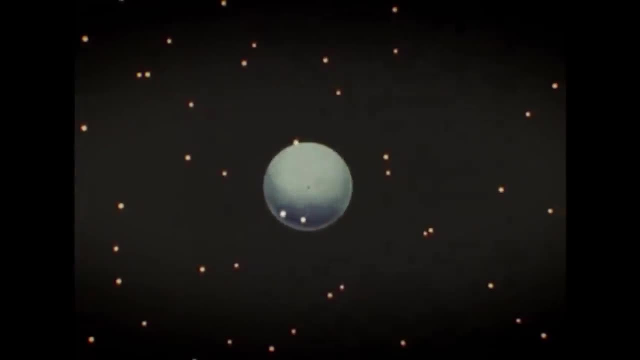 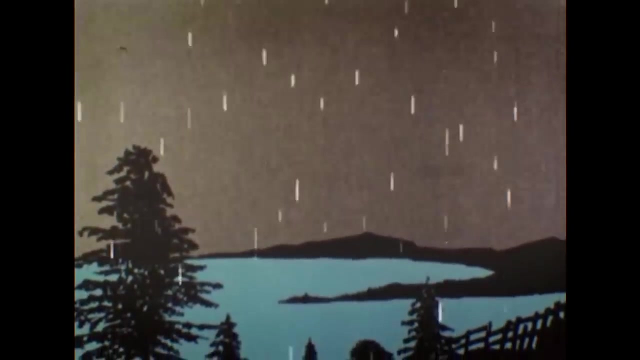 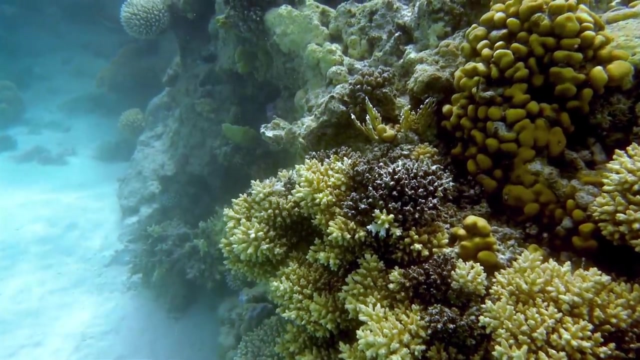 our seas. Sulfur and nitrogen oxides and other substances chemically combining with airborne water droplets change their acidity and play a key role in subsequent acid rain. This acidification in turn drives many of the water's inhabitants to the very limits of their 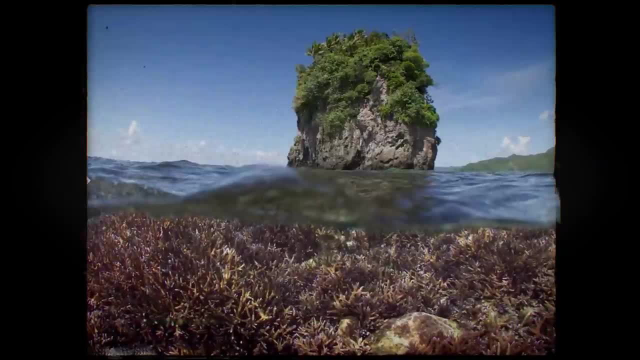 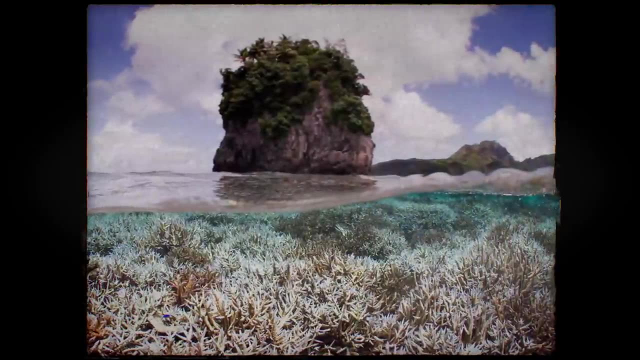 tolerance, not least of which being corals, which are extremely sensitive to changes in pH, to the point where even a small increase in acidity can cause wide-scale bleaching, And I feel like I shouldn't have to explain why protecting coral reefs is important. but okay for the people who still aren't convinced. taking care of the earth benefits us all directly. corals not only serve as the foundation of what are by many considered to be the richest ecosystems on the planet, but also serve as the spawning grounds for many of the fish we rely on for food. 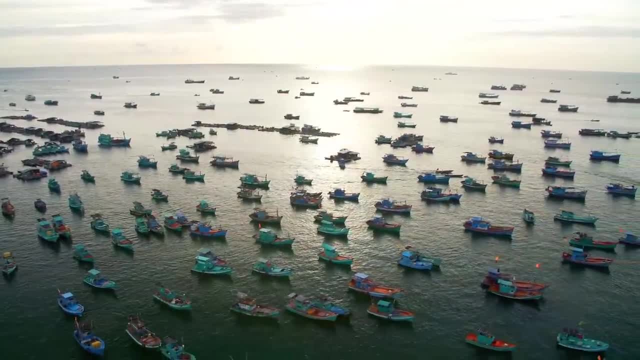 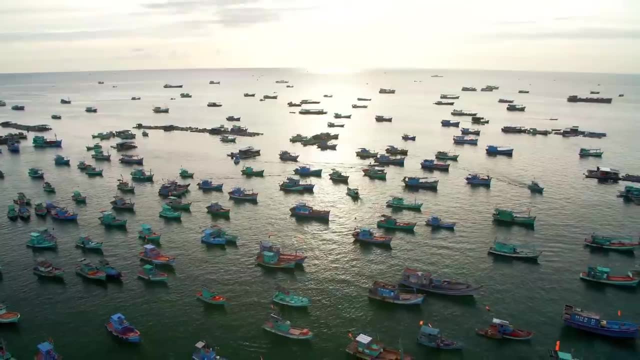 feeding over 3 billion people. But even more than that, we rely on corals to support our entire fishing industry, employing 260 million people worldwide and generating over 240 billion per year of fish per year, And that's why corals are so important to us. Corals are so. 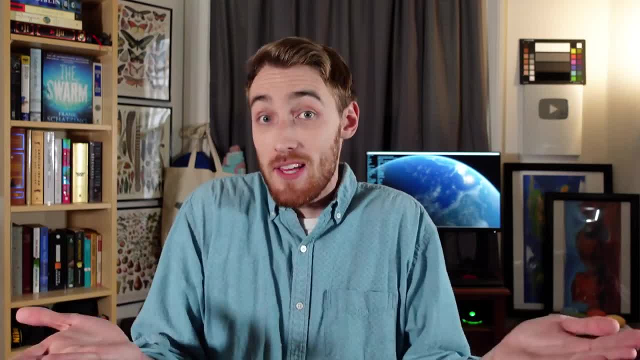 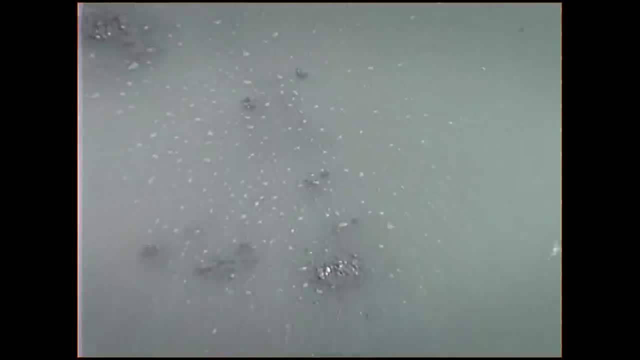 important to us because they make up about a billion dollars in revenue each year. So, yeah, a pretty important thing for us to protect from an acidifying ocean. The devastation of lakes is matched by the corrupting of our coastal bays and estuaries. 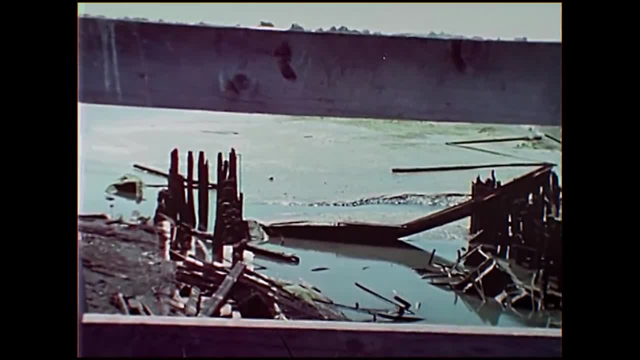 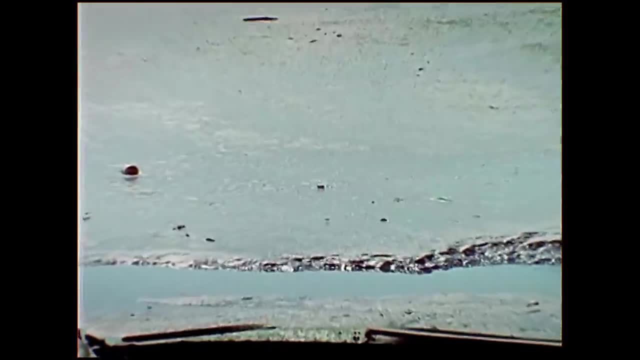 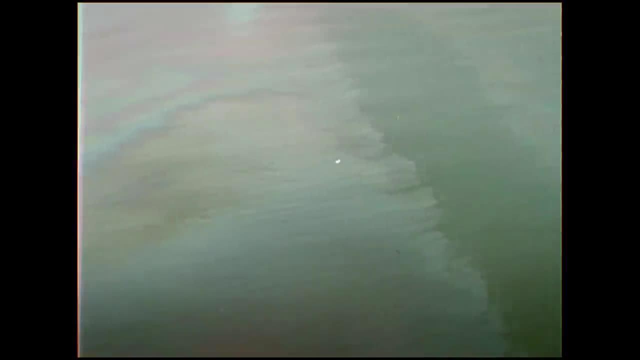 In filling and polluting these water resources, we are burying major sources of oysters, lobsters, clams and shrimp. Oil wastes are even entering the organic food chain. We may lose the sea, but we'll have to deal with that later. 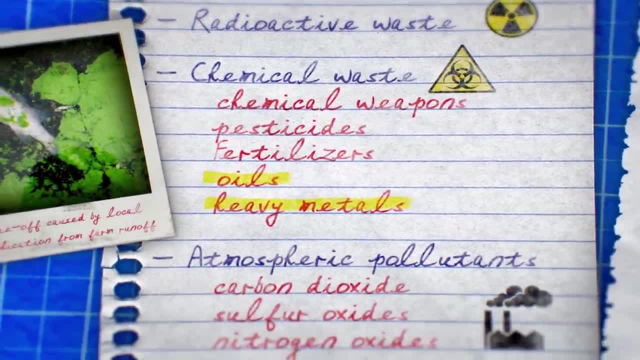 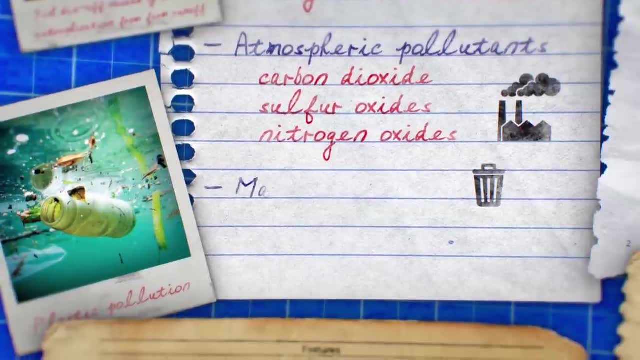 Okay, and the last category of major ocean pollution is the one you've probably all been waiting for, the one Team Sees is actually trying to address trash, or what we'll be calling material waste. Okay, and the last category of major ocean pollution is the one you've probably all been. 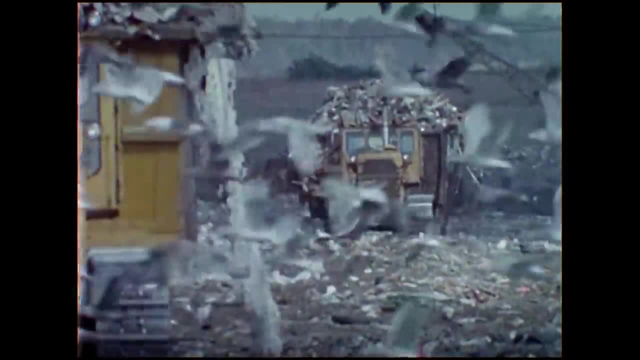 waiting for the one Team Sees is actually trying to address trash, or what we'll be calling material waste. Now, our genius for production and consumption mocks us. We are converting to garbage the gifts of the land and water that we use to feed our people. The ocean is our source of food and water, and it's 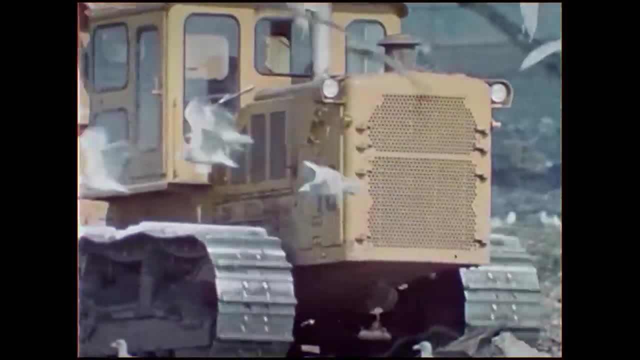 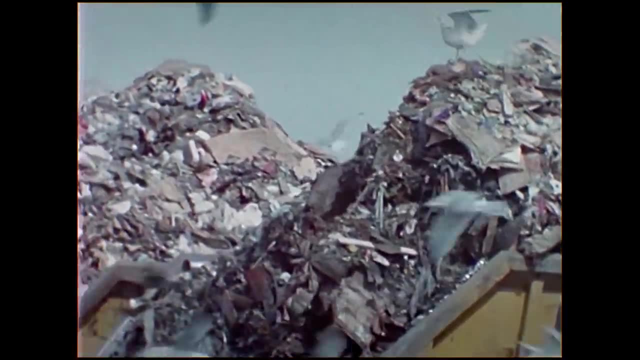 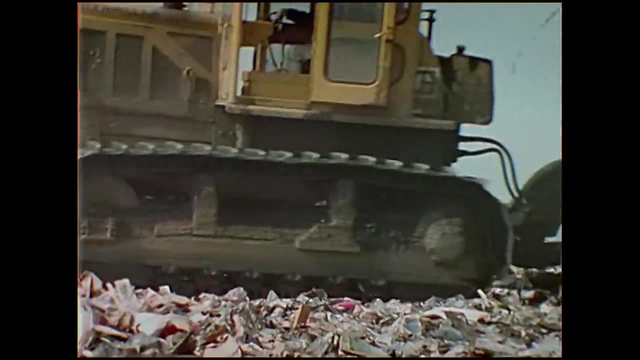 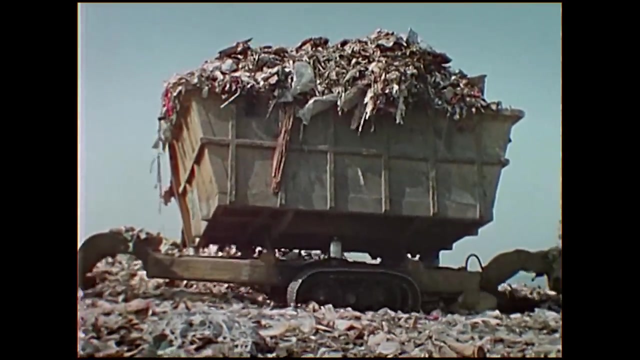 water so rapidly that some of our vital resources are beginning to run out. In the old days we threw it out the window. Now we employ armies to haul it away, burn it or dump it at sea. Tires, mattresses, steak bones, orange peels, cans and 33 million immortal. 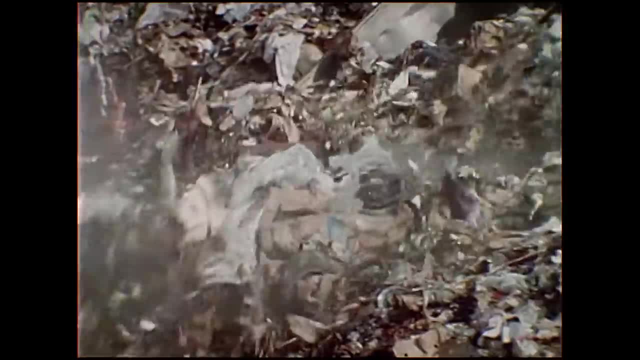 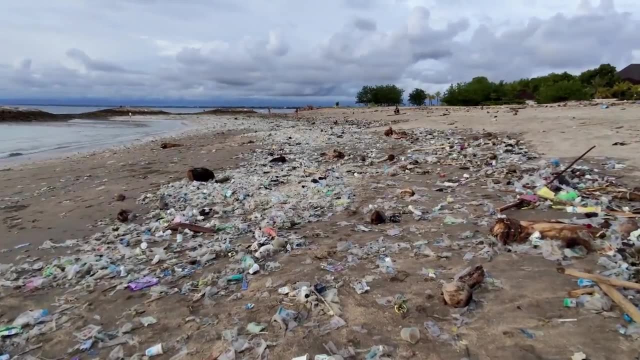 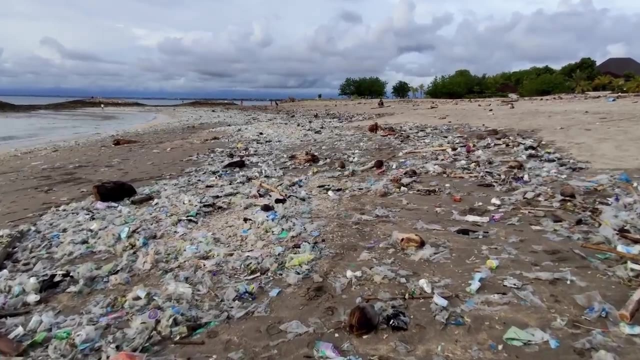 bottles, Six pounds per person, Half a million tons a day, Every day. While material waste like this may not be as toxic as some other forms of pollution we've talked about so far, there's no doubt it is by far the most widespread, Afflicting riverbanks, coastlines and far into the middle of. 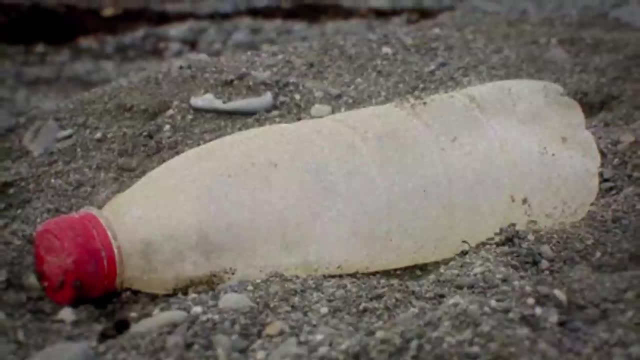 the ocean. plastic pollution can now even be found as far as the beaches of Antarctica, where it washes ashore thousands of tons of plastic. And that's not all: Plastic pollution can now even be found as far as the beaches of Antarctica, where it washes ashore thousands of tons of plastic. Plastic pollution can now even be found as far as the beaches of Antarctica, where it washes ashore thousands of tons of plastic. And that's not all: Plastic pollution can now even be found as far as the beaches of Antarctica, where it washes ashore thousands of tons of plastic. 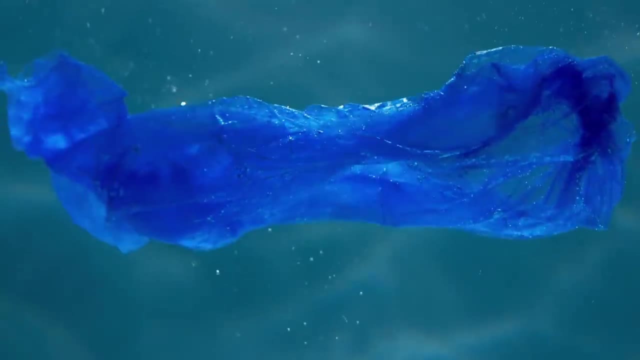 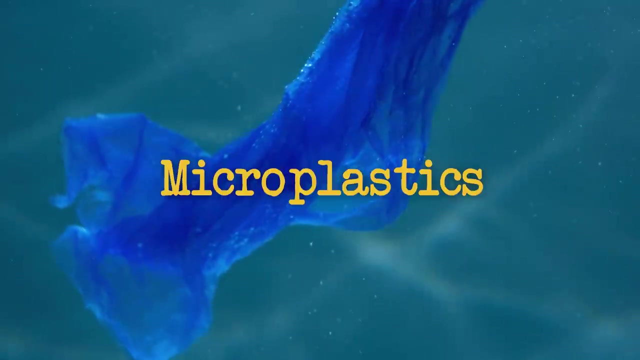 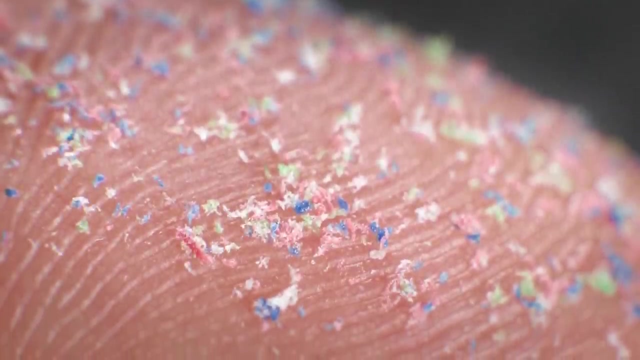 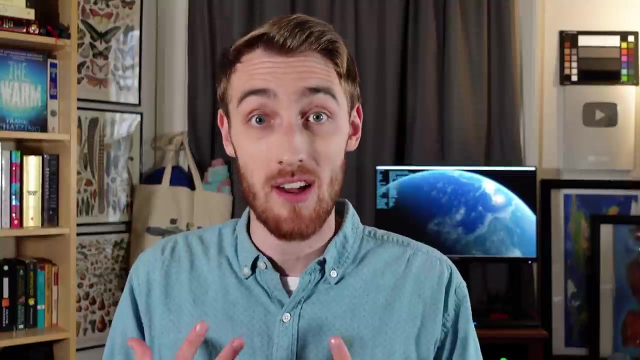 The overall health of an environment is degraded by the plastic calm that comes around us, as the plastic that receives more pollution in the ocean as a whole tends to evolve in one direction or another over time and can produce even more things on us, is always detrimental. And okay, now that we've had a basic introduction to the true scale. 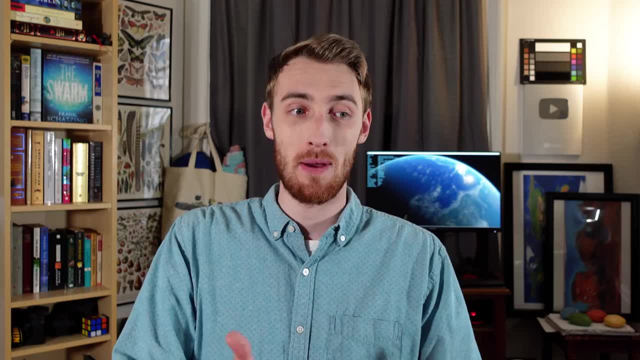 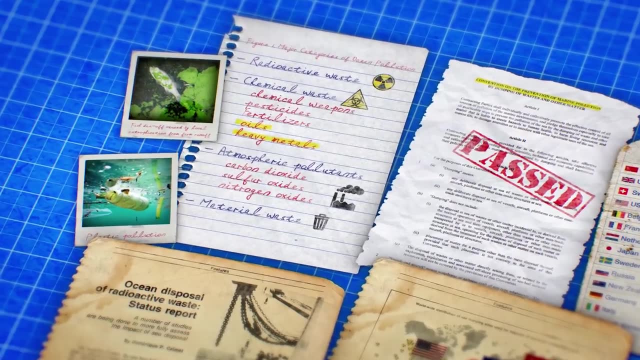 and depth of ocean pollution, we can finally start talking about the strategies for remediation, or in other words, how to actually clean up the ocean. And in case you didn't realize it, the real reason I broke everything into categories is because each one requires a different approach. 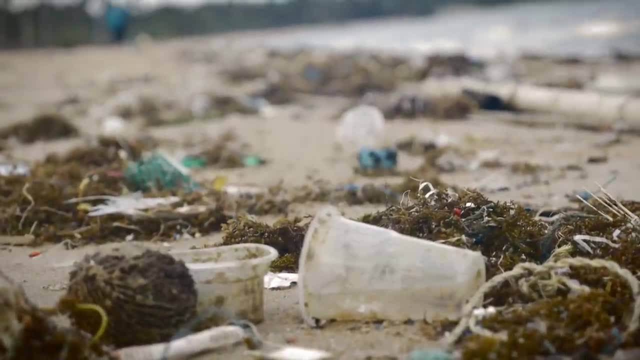 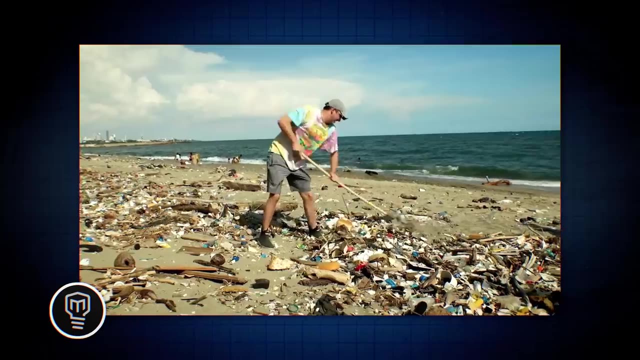 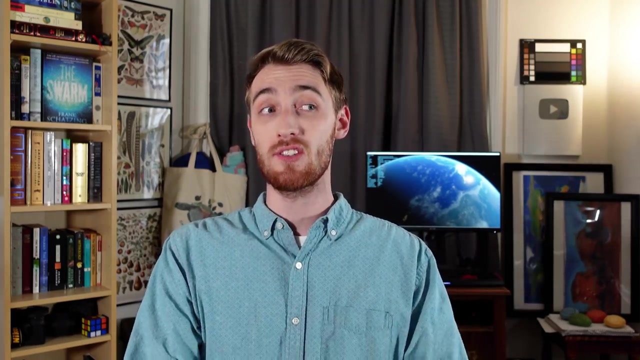 to remedy. To start us off, material waste is possibly the easiest pollutant to clean up, given its- you know- solid nature. collecting trash can be done both by human hands or by fairly simple machines, And I expect this is why removing trash from the ocean is the main focus of Team. 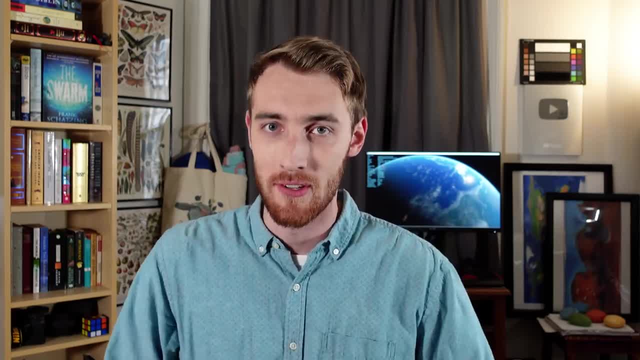 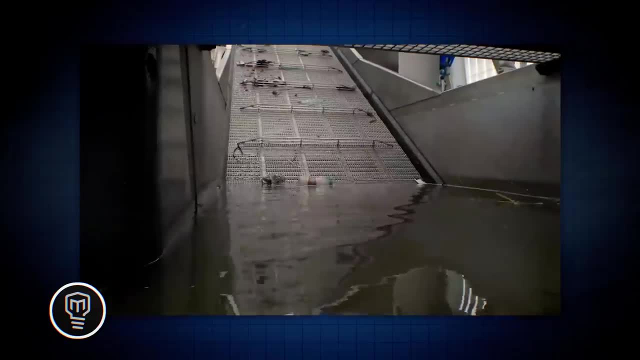 Seas. Remember: one dollar equals one pound of trash removed. Now I don't want you to see this as a knock against Team Seas. It isn't. Not only is cleaning up material waste still an important aspect of ocean remediation, but also it just makes sense to focus on what we can directly affect. 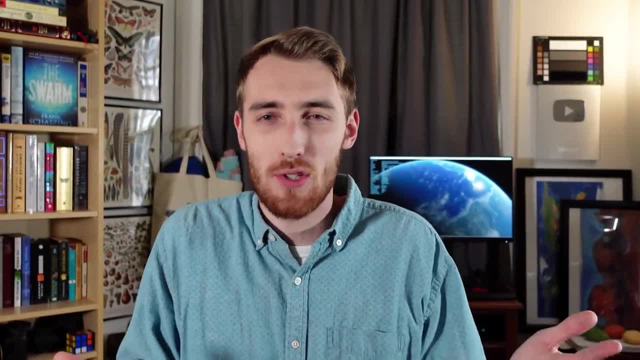 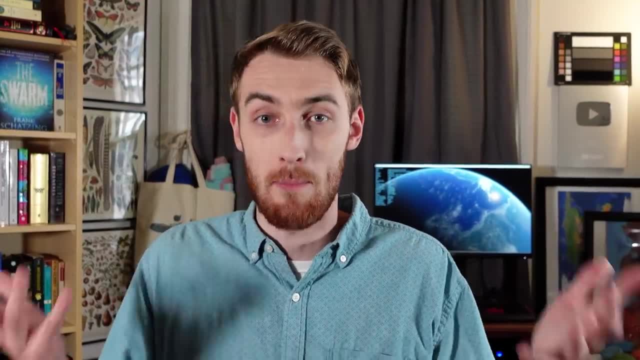 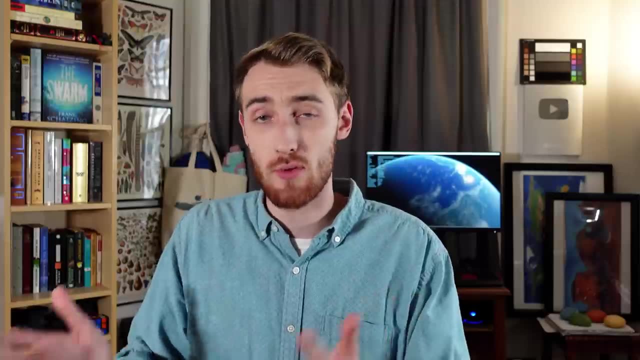 heavy metals, pesticides and mustard gas from ocean water at an impactful scale. smart And sure, Mr Beast can spend money or whatever, but not like the billions of dollars required to retrieve and treat everything lurking on the ocean floor In every way, sticking to cleaning up material. 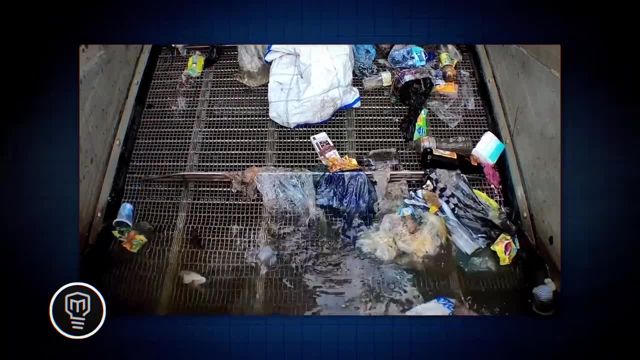 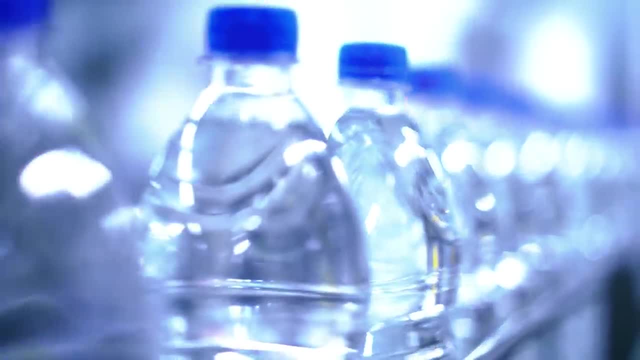 waste, and even catching it before it gets the chance to enter the ocean, is the most we can expect individuals to be able to do, And really, by this point, the onus should be on the company producing this waste more so than the people consuming it. That being said, this still leaves. 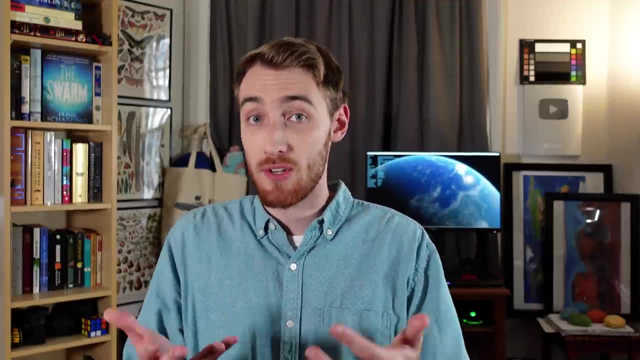 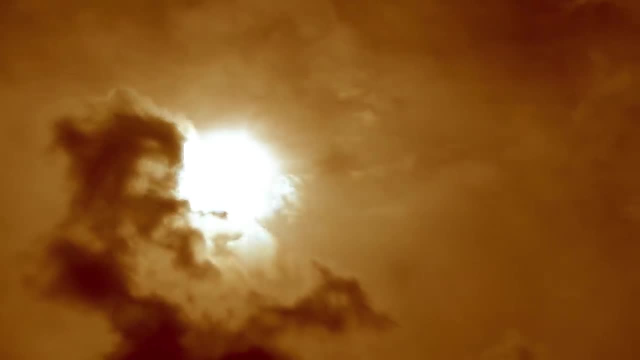 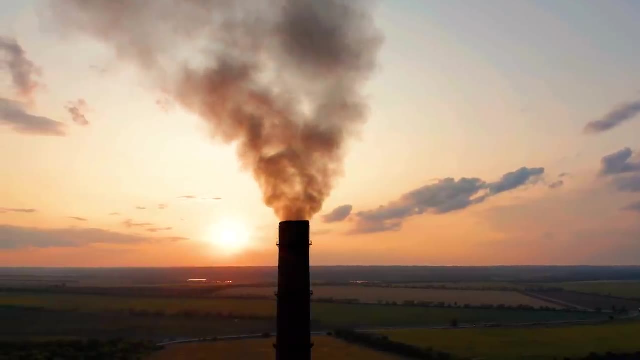 us with three whole categories of pollution, each one more dangerous than the last, and each one with their own array of challenges to clean up. Maybe the next easiest, but also maybe the hardest pollutant to keep out of the oceans is dissolved gases. You see, while we in fact have absolutely 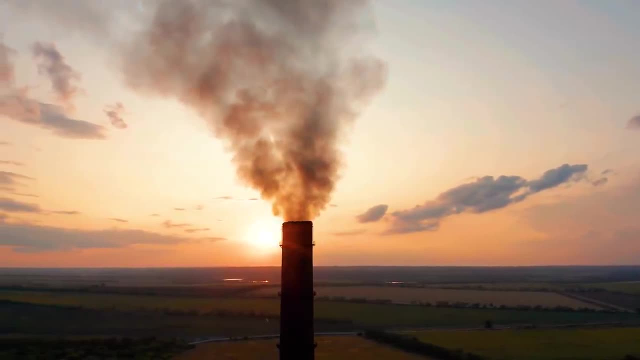 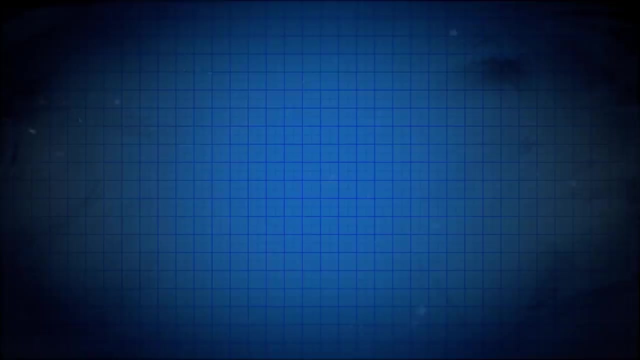 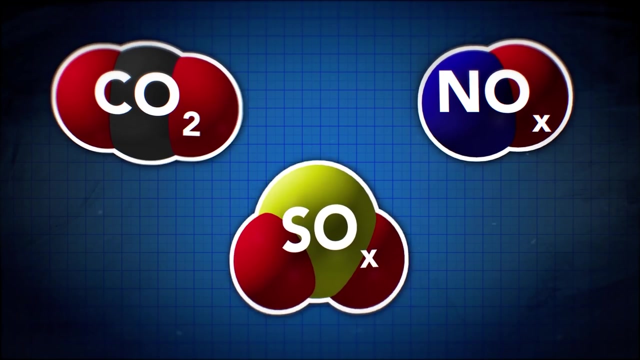 no control over what gases dissolve from the atmosphere into the ocean, we do have control over what gases we put into the atmosphere, Lucky for us. whether it's carbon dioxide, sulfur oxides or nitrogen oxides, all of these gases share the same points of origin: the burning of fossil fuels. 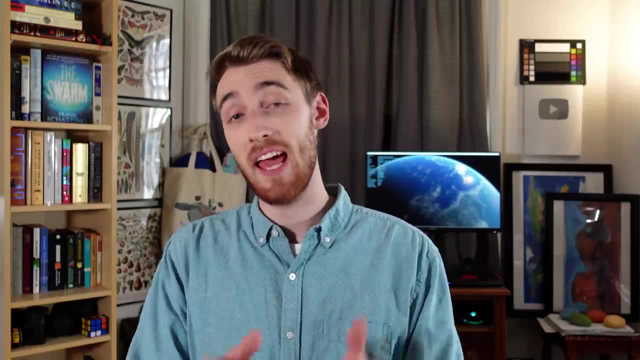 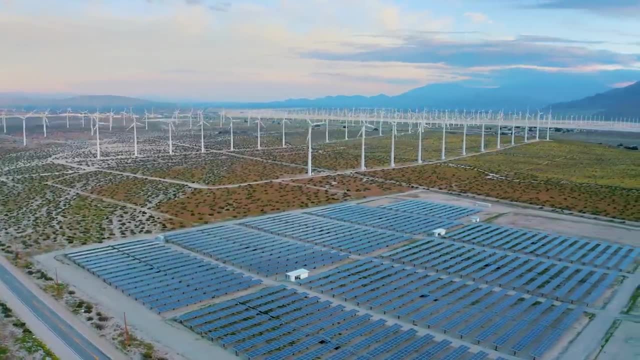 This means combating ocean acidification goes hand in hand with combating climate change, and so the steps we've only just started taking, like investing in renewable energy sources, electrifying our machines and increasing overall energy efficiency, also need to be taken into account, And that's why we're talking about how to clean up the ocean. 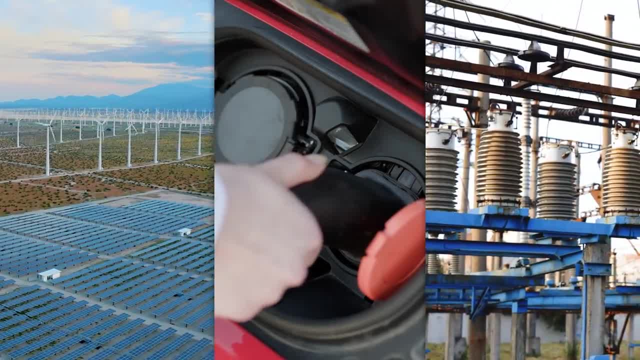 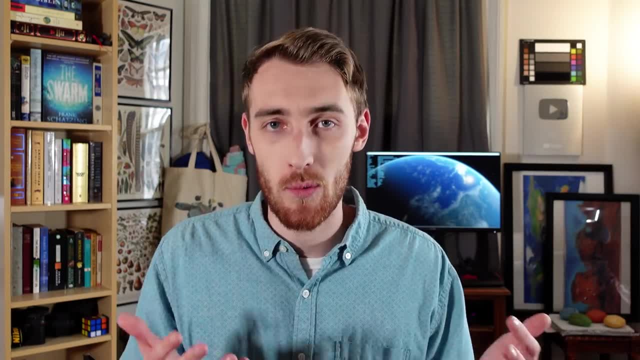 have the added benefit of preventing these gases from escaping into the air and from there into the water. And while tackling our emissions is still a Herculean task in its own right, it's one that, at the very least, has already begun, which is more than we can say about our last two categories. 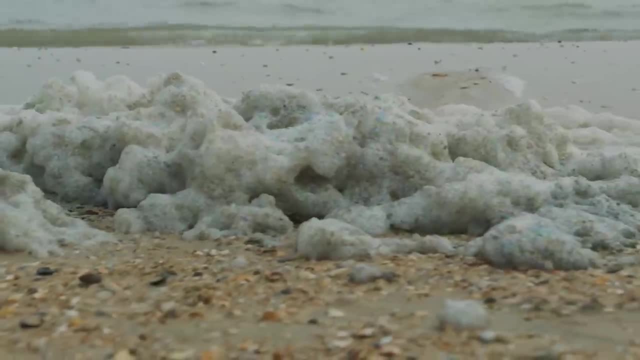 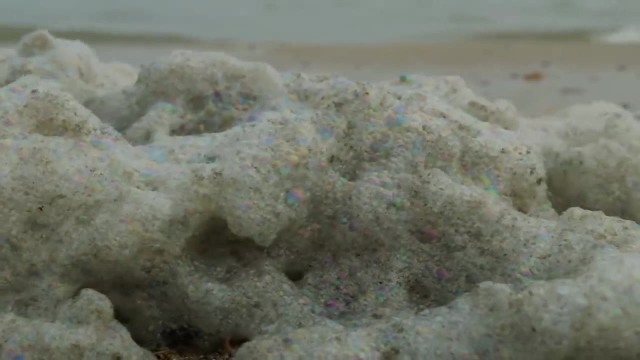 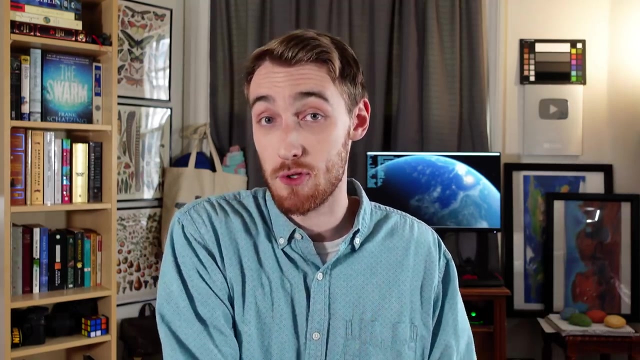 And I'll admit this is where things get tricky, as most forms of radioactive and chemical waste that's entered our oceans has already mixed in thoroughly with ocean water and can never be filtered out in a cost-effective manner. But maybe you noticed I spent most of my time talking about the few examples. 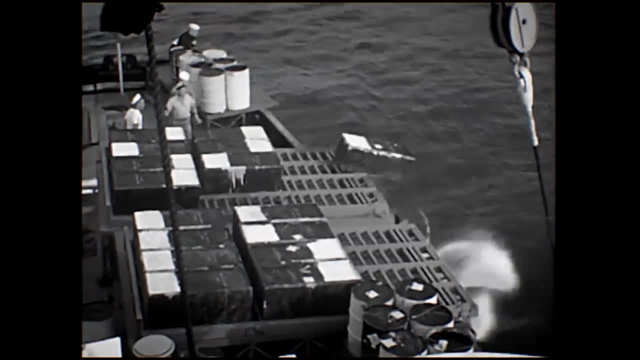 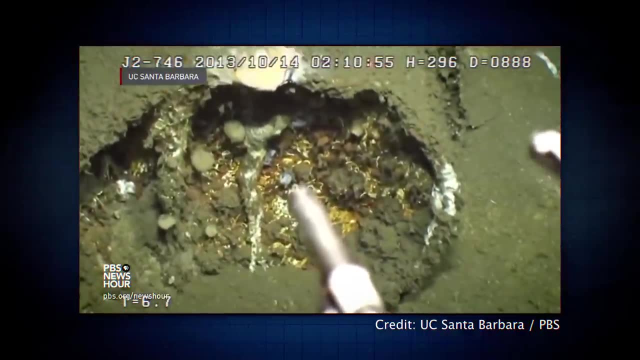 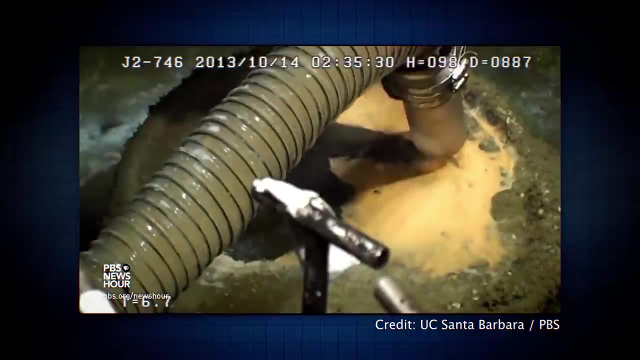 where the contaminants have been neatly packaged and dumped within specific sites. Like I said earlier, while this still isn't a perfect solution, because these barrels will all still eventually break down and leak their contents, packing them up like this at the very least has given us a window of time to act and retrieve most of the barrels before they rust away. Because, say it with me- the number one way to clean up the ocean is to prevent pollution from entering the ocean. Because, say it with me- the number one way to clean up the ocean is to prevent pollution from entering the ocean. Because, say it with me, the number one way to clean up the ocean is to prevent pollution from entering the ocean. 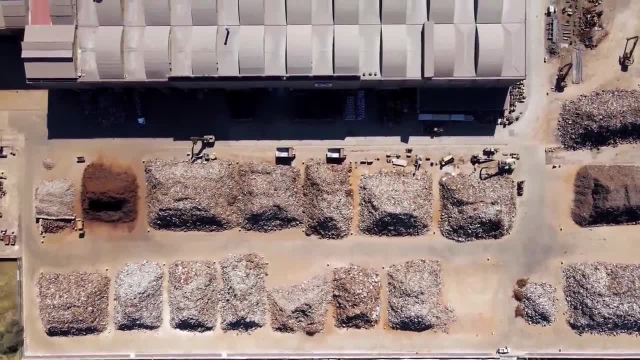 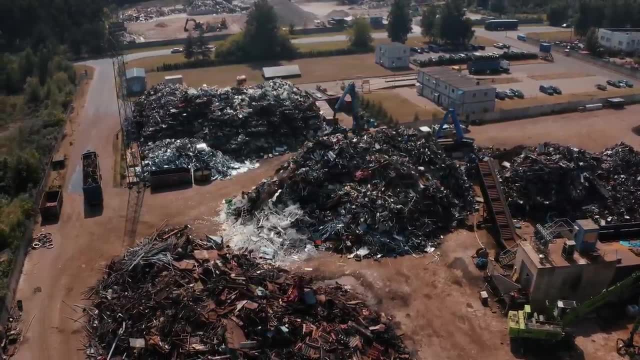 Now, of course, this still leaves us with the huge problem of what to do with these hazardous waste materials once we've gotten them back on land. but at the very least we'll be able to keep a better eye on where these pollutants end up. 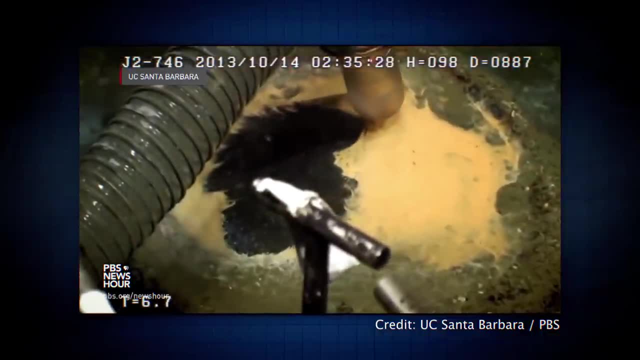 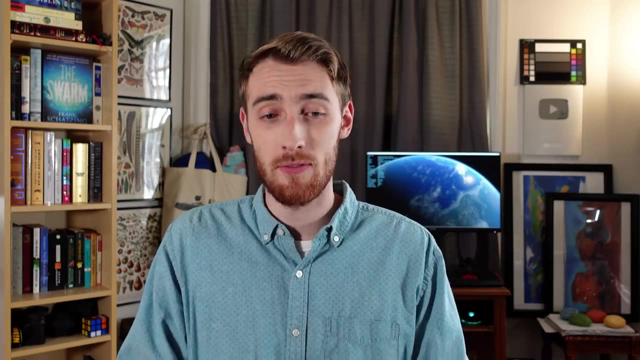 and make sure they don't just willy-nilly spill into their surrounding environment. The only real obstacle this all faces is that this big of an operation just isn't within the realm of possibility for a group of ragtag YouTubers like us, and really the responsibility falls on the shoulders. of larger organizations like governments and corporations to clean up, Which again, is easier said than done. but hey, it's a start. Take all those chemical weapons sitting off the shores of the eastern United States, for example. They were all produced in American factories under orders of the American government. 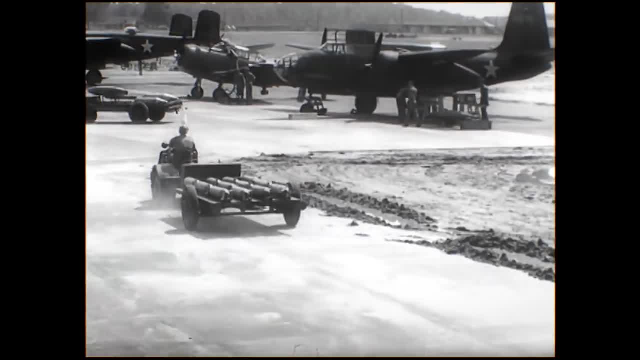 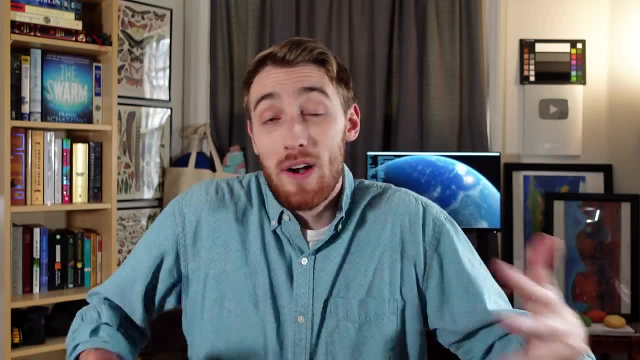 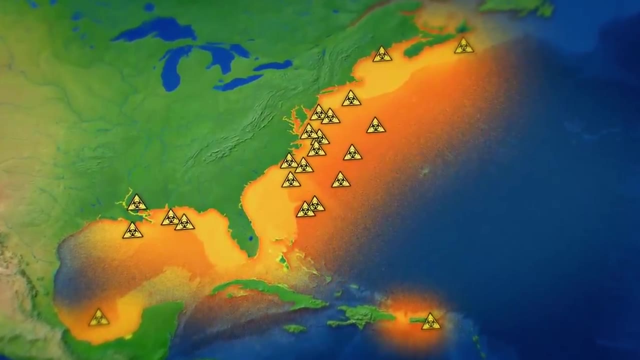 for use by the American army against any possible American enemies. But now I want you to imagine a different scenario, One in which China or Russia or Iran or whatever vague anti-American boogeyman you want, if any hostile country planted millions of barrels of chemical weapons. 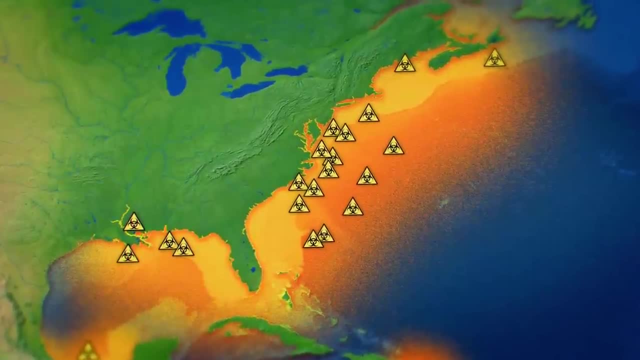 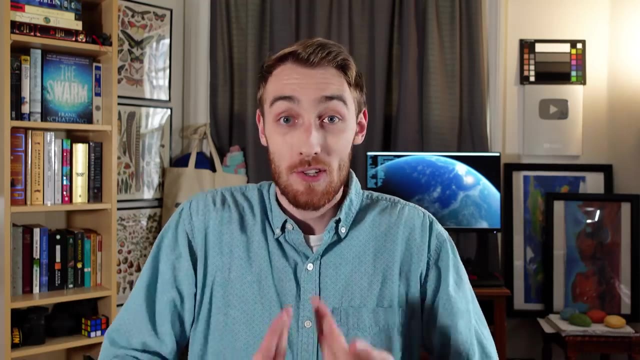 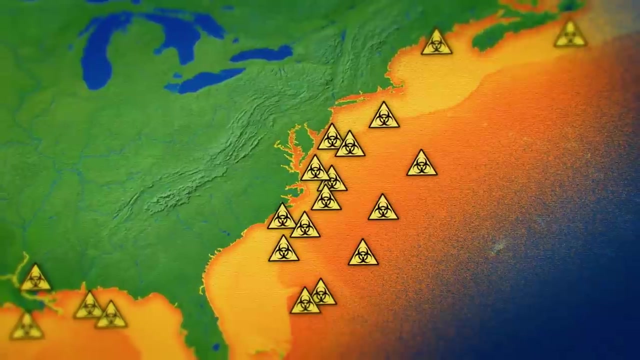 off American shores, we would immediately respond with an attack, and our number one priority would be to clean these up before they hurt us. So why do we tolerate them now? simply because we were the fools who put them there. I mean, these are chemical weapons, after all, Tools of war located directly off our shores. 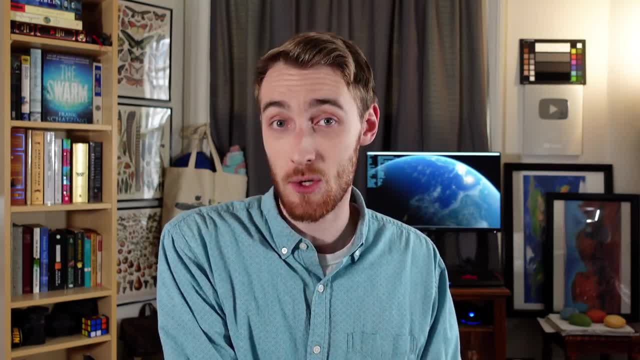 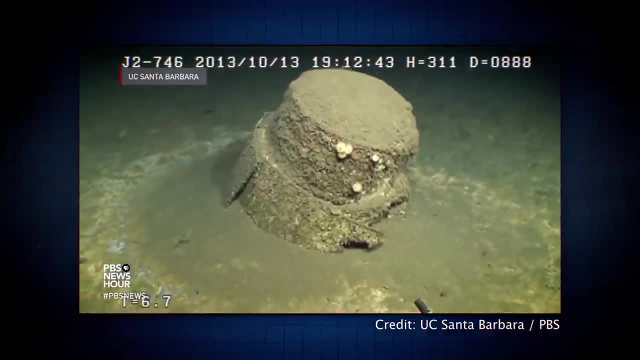 Which, in my opinion, makes this not even an environmental issue, but rather one of homeland security. I mean, think about it. all a foreign agent really needs to do to wreak havoc across the entire eastern seaboard is to take a submarine down to the unsurveilled seabed. 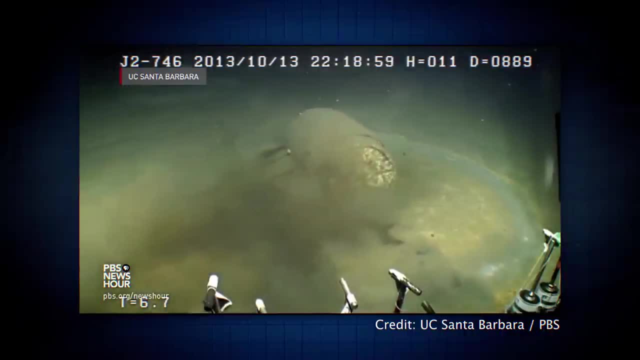 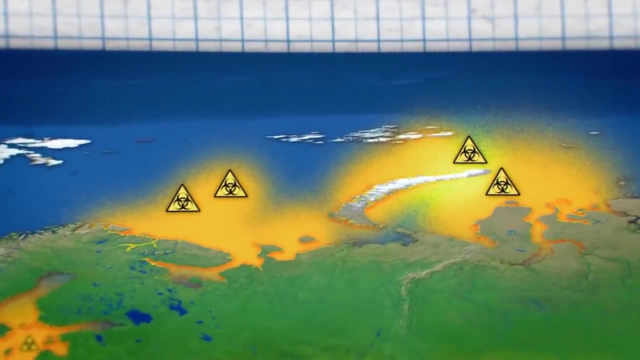 and just start poking holes in our already-rotting barrels. And this goes for not only the US, but really every country. How would Russia feel if it was the US putting 150,000 tons of nerve gas on their shores? How would Europe feel if Nazi Germany? 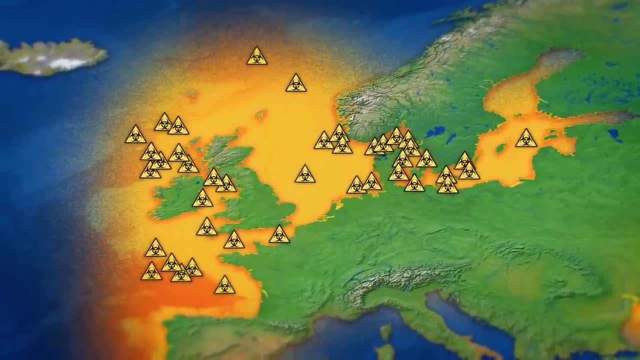 How would Russia feel if it was the US putting 150,000 tons of nerve gas on their shores? How would Germany came back and planted mustard gas all throughout its seaways? How would Japan react if it were North Korea putting poisons under their fishing grounds? 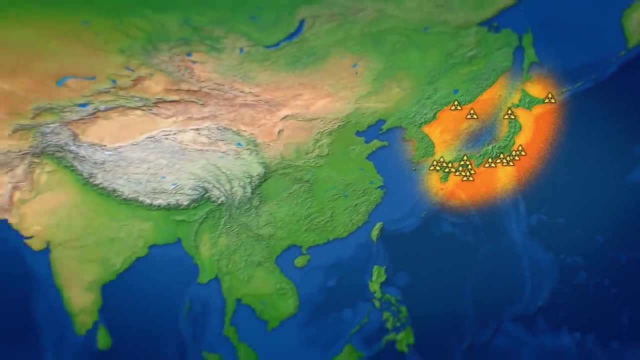 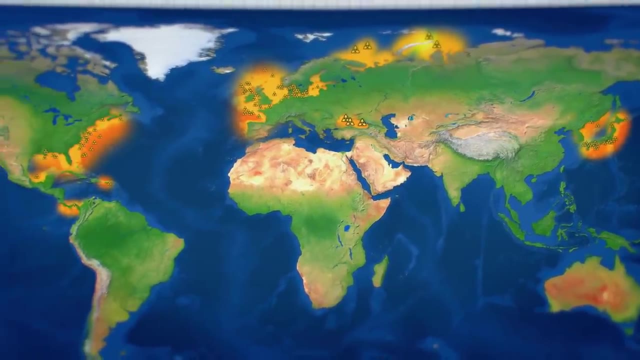 And that's not even to mention all the other countries of the world that haven't partaken in any of this but would still feel the consequences if these chemicals were released into the environment, Because of the similarities between how nuclear waste and chemical weapons were disposed of. 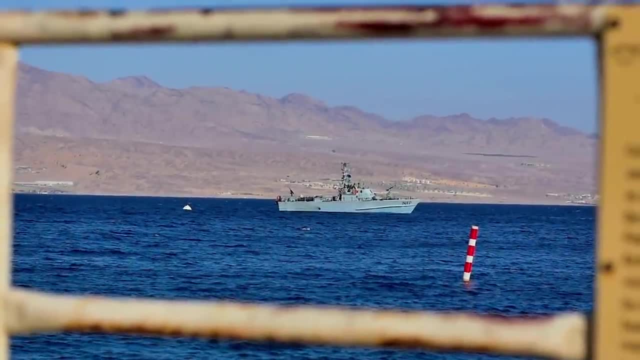 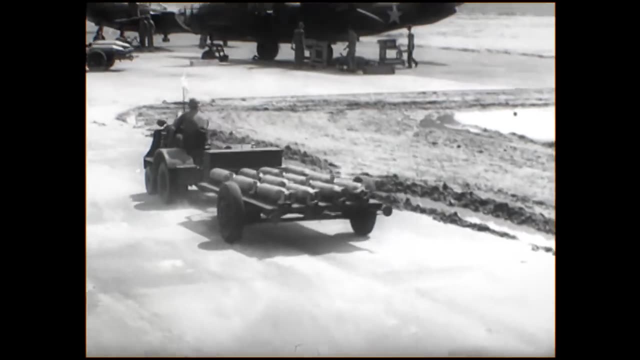 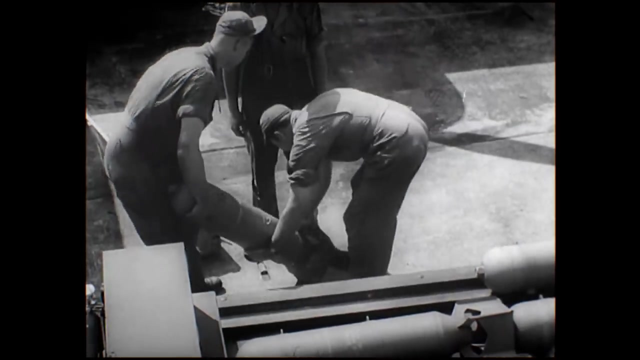 and who was in control of this dumping. this means this approach of holding governments responsible also works for radioactive waste, though with one big exception. You see, while chemical weapons were almost exclusively made by governments for military use, not all nuclear waste was. 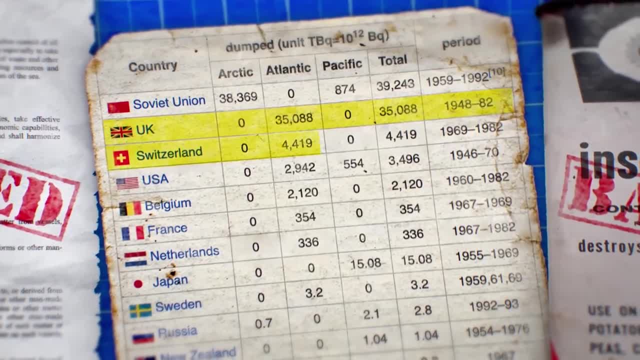 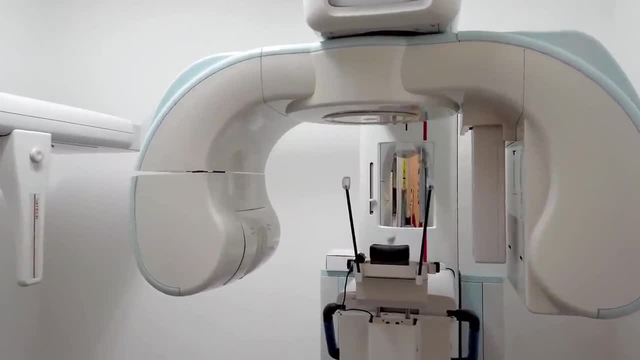 If you'll remember, countries like the UK and Switzerland topped the charts despite not having a large or any nuclear weapons, and instead most of their waste came from the manufacturing of advanced medical devices which use radioactive materials for a wide range of machines and purposes. And considering somebody profited off the creation of nuclear waste. now the responsibility not only falls on governments, but also companies and corporations that made money off of this. In fact, the same goes for oil companies, pesticide companies and really anyone who benefits from polluting the world's waters. 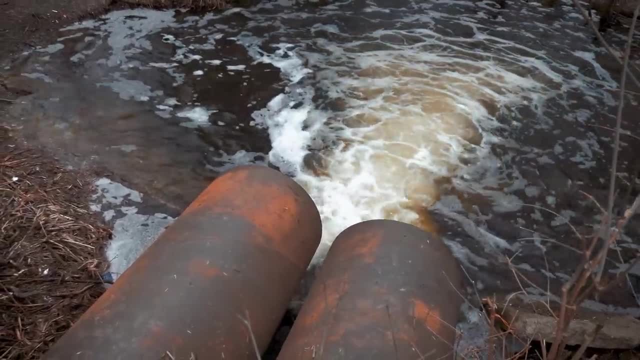 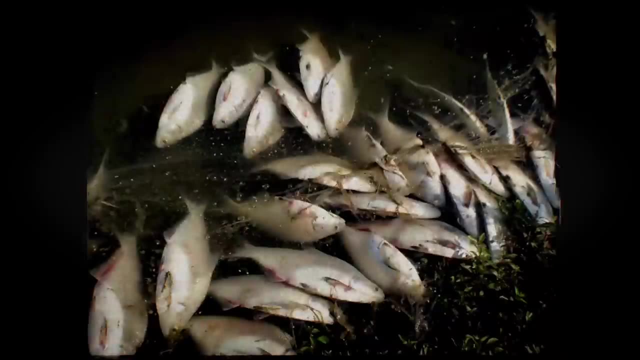 At the end of the day, while it might be free to dump waste in the ocean, this nevertheless doesn't come without a price, one that's paid through environmental damage, reduced fish hauls, lost tourist dollars, adverse health issues and more.